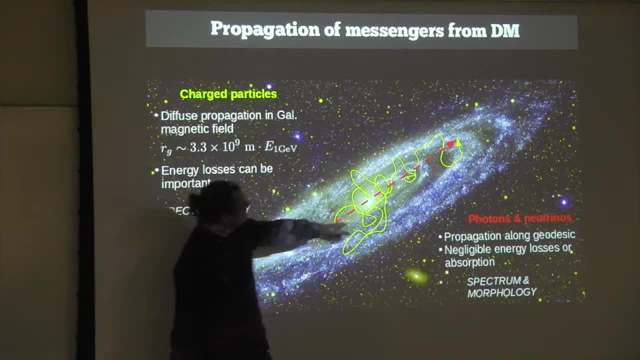 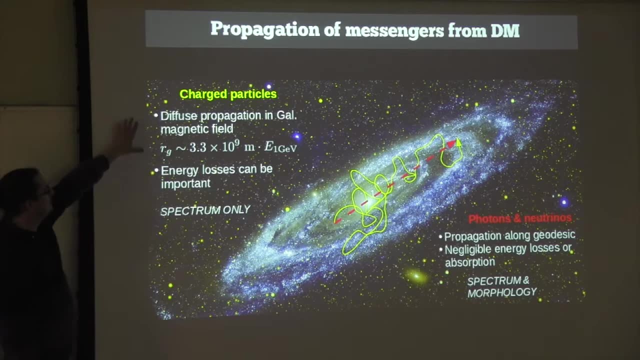 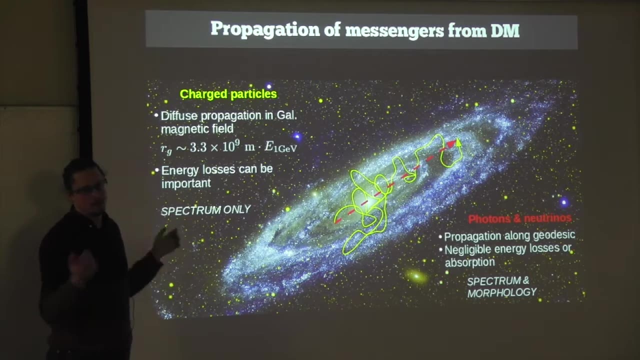 neutrinos. that's easy, because in some way, because they just come to us on straight lines. If it instead generates charged particles, then the gyro radius of these particles in microgauss magnetic fields is of the order. it depends on the energy, but it's typically of the order of the 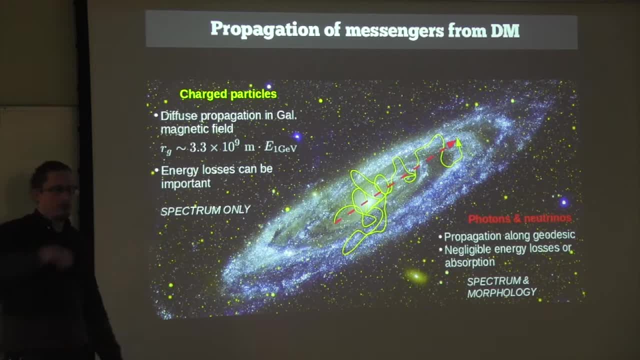 oscillators. So if you have a field and you have a magnet and you have a particle that is made up of two or three astronomical units or something, so these particles would spiral around, follow magnetic field lines and then, because magnetic field lines in the galaxy have a turbulent 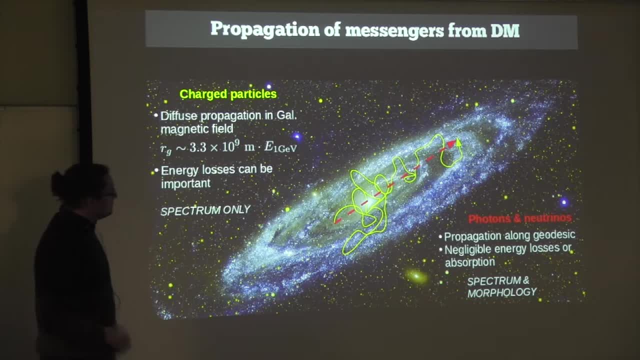 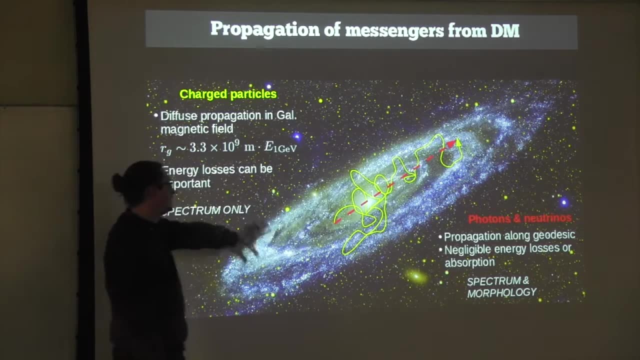 component, they would basically start to scatter. So this can be calculated with pitch, angle scattering And ultimately this would lead to mostly diffuse propagation, And in fact, what one does in reality is to usually just model this with isotropic diffusion. So, instead of knowing, 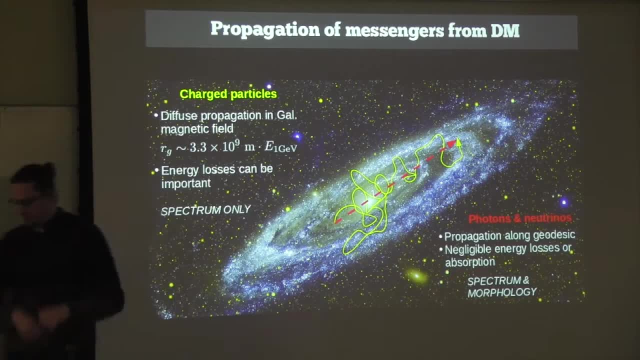 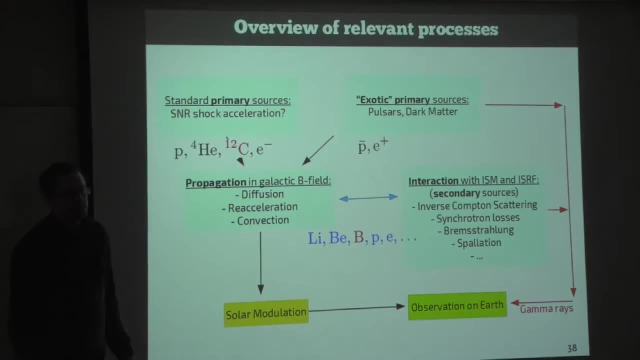 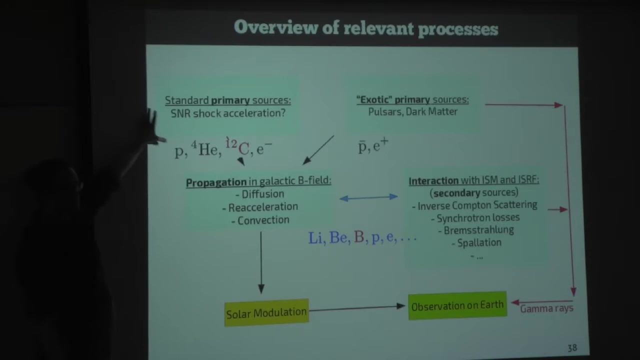 field. you just assume they diffuse, like in the diffusion equation and this. this process is isotropic, but that's only one of the processes one has to think about. so if we want to discuss what's actually the background- and first the signal, but then also the background component for anti, anti proton searches, we first have 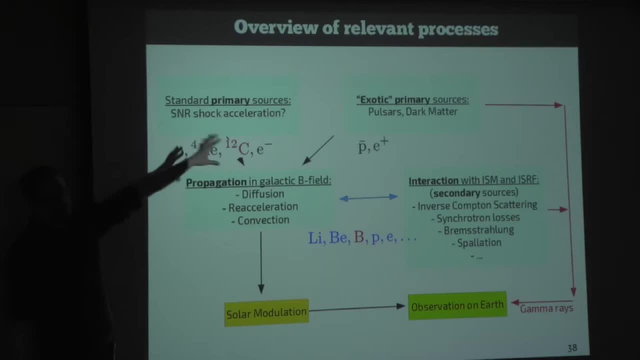 to think about primary sources. so the primary sources for cosmic rays in the galaxies, in the galaxy are still not hundred percent proven, but it's a good working hypothesis that this comes from diffuse shock acceleration and supernova remnants, which would then accelerate protons, helium, carbon, everything charged. 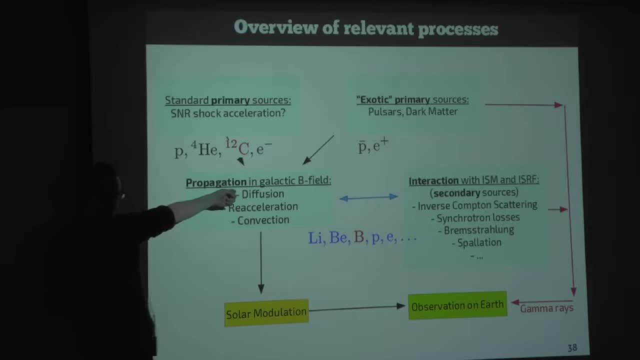 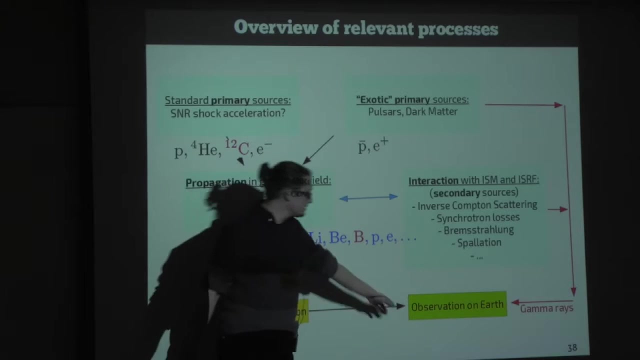 and propagate in the magnetic field the diffuse way, but also a convective. winds can play a role, or a acceleration, which is something like diffusion in momentum space. so particles could accelerate by scattering on- I've been Vinic, I've been Vinic waves. then these particles, before they are actually measured at Earth, would suffer from solar 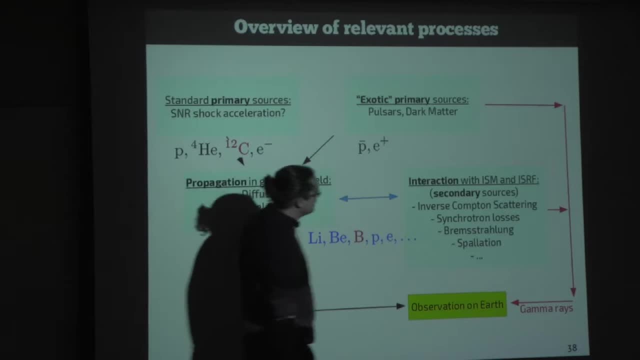 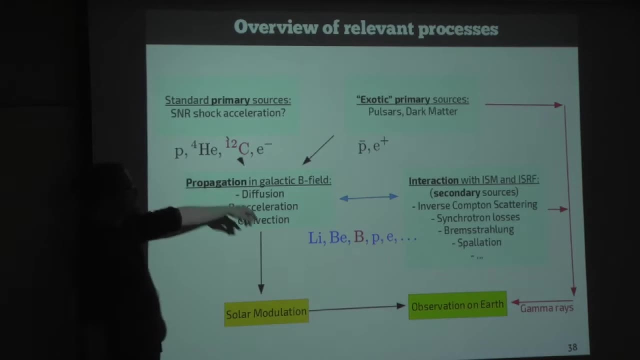 modulation, which affects mostly the low energy part of the spectrum. and then there are also interactions with interstellar medium in the interstellar radiation field. so in particular electrons would lose energy by synchrotron and branch column and inverse Compton scattering and the the nuclei would, in particular the heavier ones would have spallation, so spallation processes. 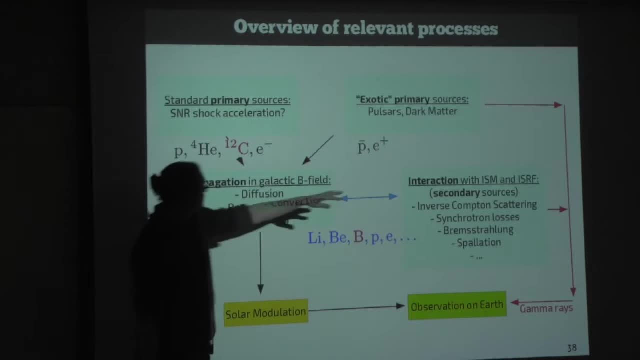 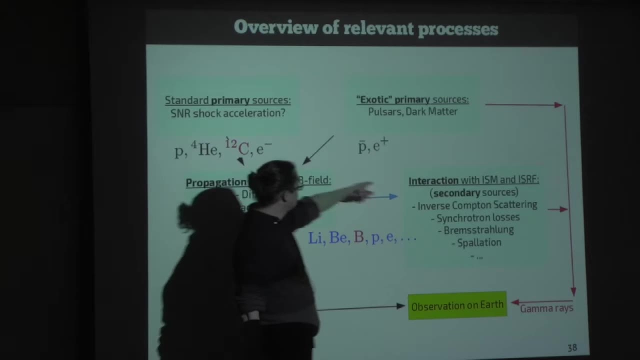 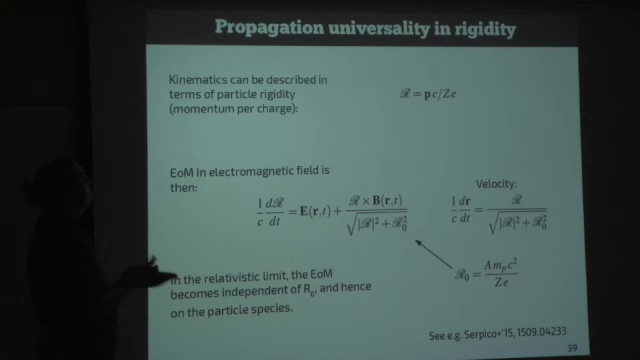 play a role- I will come to that in a second- which then again feeds back into what actually propagates in the galaxy and affects observations, and these interactions actually produce what is called secondary sources, secondary cosmic rays. okay, what's interesting and important to understand- why one can understand anything at all- is 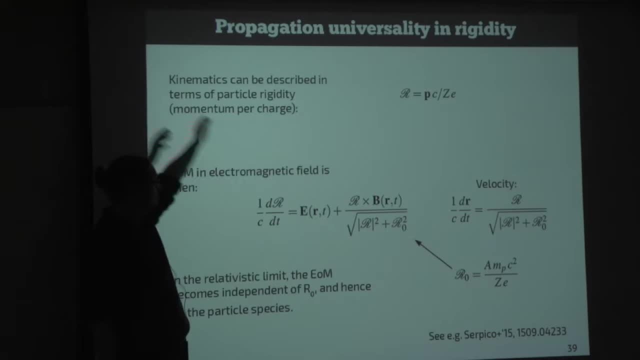 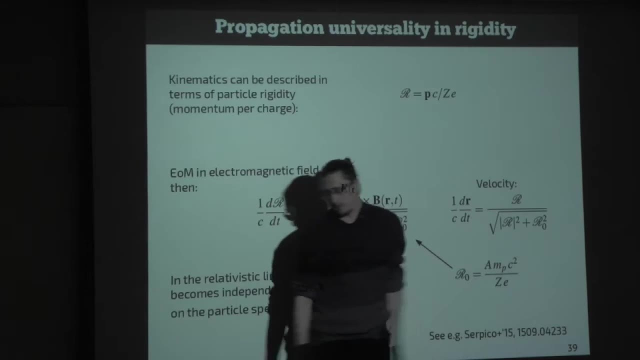 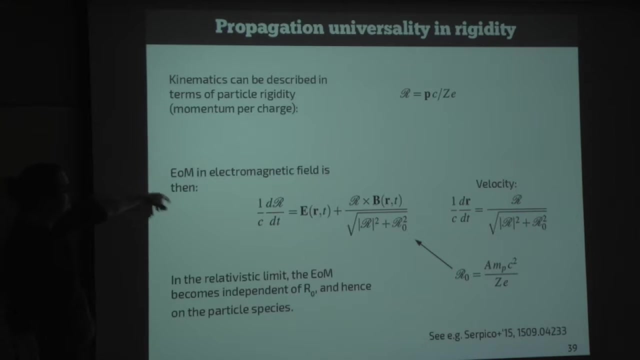 that what matters at high energies, when particles are relativistic, is mostly just rigidity. rigidity is defined as the momentum of the particle divided by its charge, and if you write down the equation of motion of particles in electromagnetic fields in terms of rigidity, it turns out that, yeah, it only depends that it only depends on rigidity, ultimately. so it just 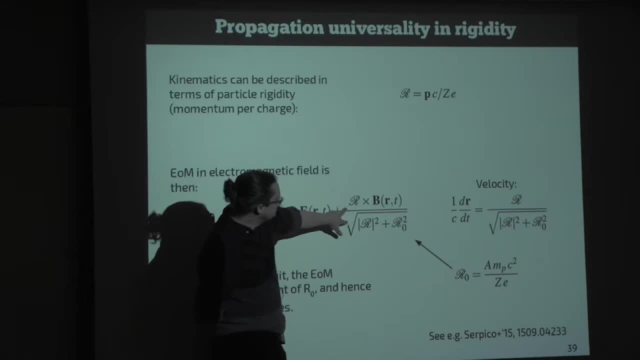 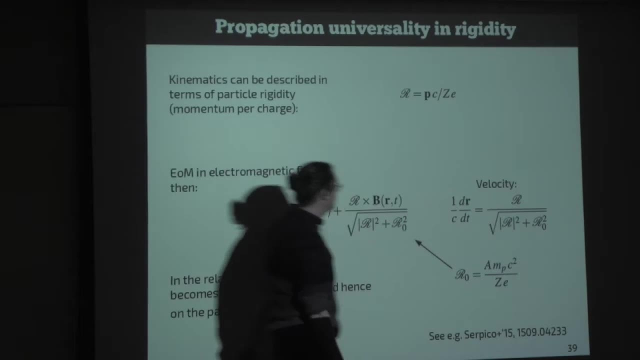 depends on the magnetic field. and then you have here the B field, times, velocity, and the velocity part still has this R0 which depends on the particle mass. but in the limit where the particle is relativistic, you see that the particle mass doesn't play any role anymore. because this anymore? because 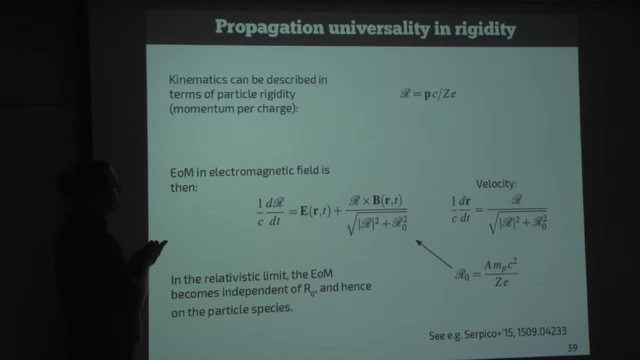 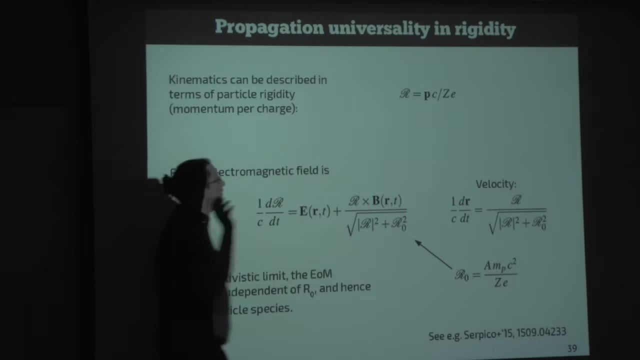 this term dominates and then then the propagation of all particles becomes universal. so it doesn't matter whether you have iron, nuclear, or a proton. if you just look at the, the rigidity, and if both particles are relativistic, they should propagate in exactly the same. 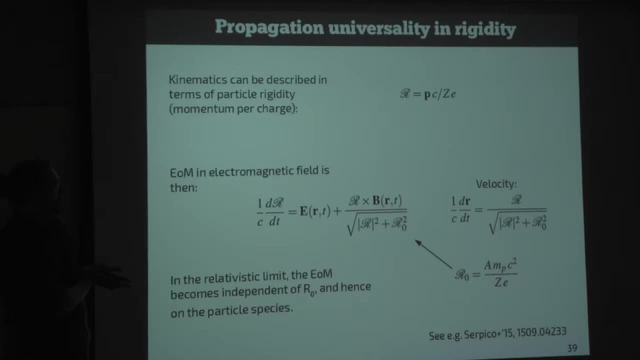 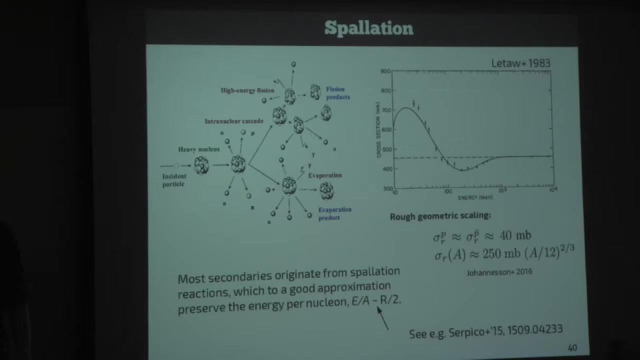 way for the galaxy. So there's a universality of cosmic ray propagation at high energies. This breaks down to the extent that heavier nuclei have a larger interaction cross-section and would scatter more often, so they suffer spallation losses more often. But ignoring that, we would expect cosmic rays to have this universal propagation properties. 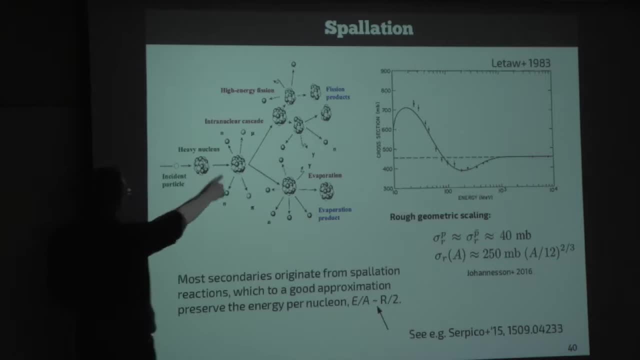 Then, as I said, spallation plays a role. So if you have heavier nuclei, it's drawn in the wrong way. Basically, heavy nucleus would hit an interstellar medium proton and then it would induce a spallation process that ultimately gives rise to just lighter nuclei. Spallation cross-sections are the level, The level of millibarn, and the very rough scaling is that they just scale geometrically. So the more nucleons you have, the bigger the cross-section. This is a very rough scaling, but just to give you an idea. 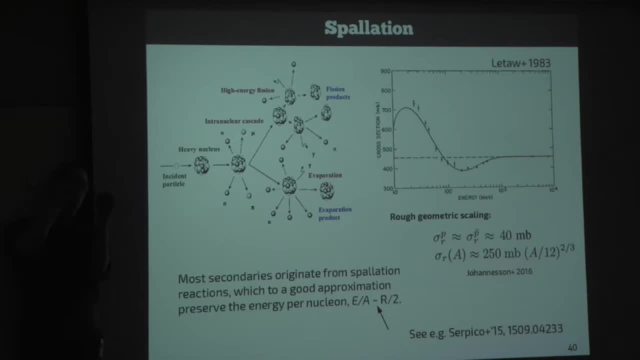 And what's important is now that usually what happens in this spallation process? you have a tiny little interstellar medium proton that is hit by a huge nucleus, So all of the kinetic energy sits in this nucleus And this thing splits up. 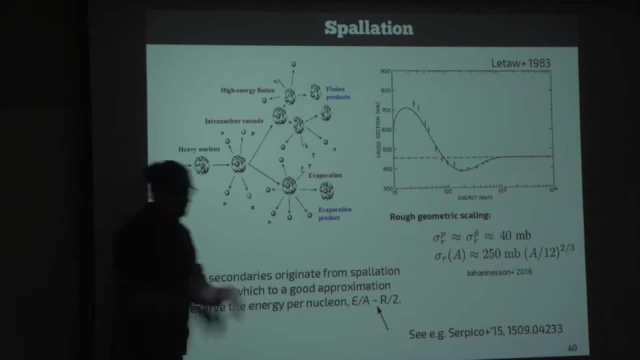 What happens then is that the kinetic energy is equally distributed onto the products, the spallation products, so that ultimately the kinetic energy divided by atomic number, A or rigidity, half is kind of conserved. So if you have a spallation process and if you look at a particular nucleus and then 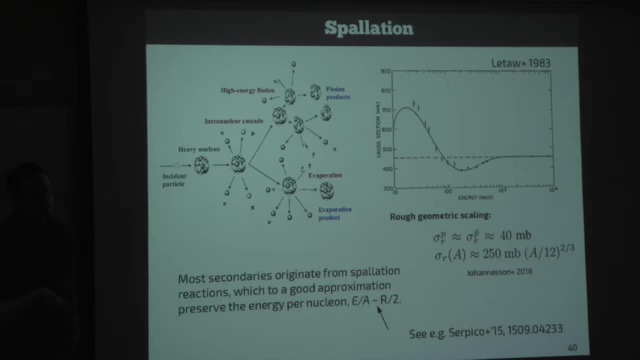 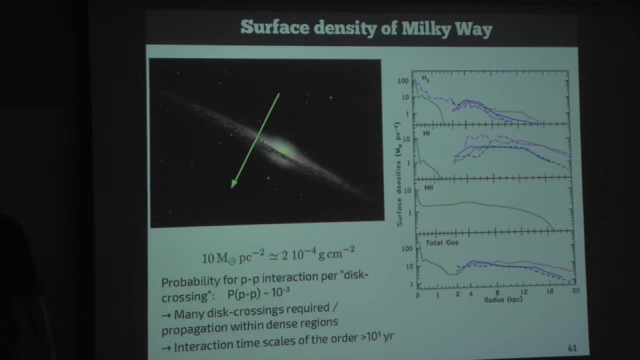 just consider The rigidity divided by number of nucleons. if this thing splits up, then the rigidity per nucleon will be approximately conserved, which makes again life much easier, because this is again another thing that simplifies actually predictions. 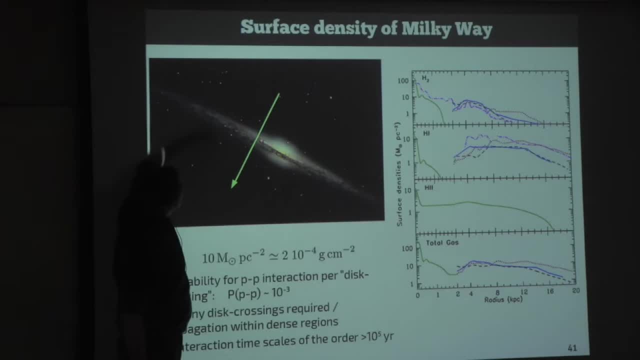 Good. So now cosmic rays propagate, not just like this but like this, And the probability And what matters now is the column density. If you look through the graph, you can see that, the column density. if you look through the graph, you can see the column density. 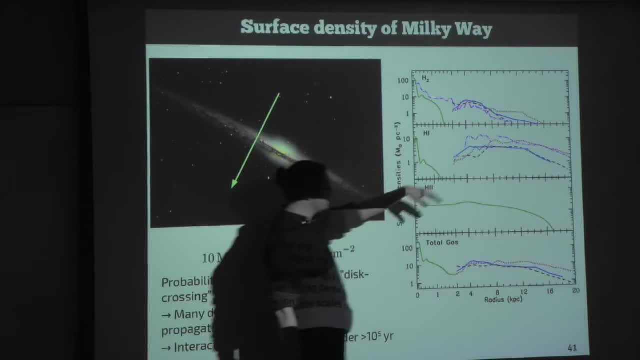 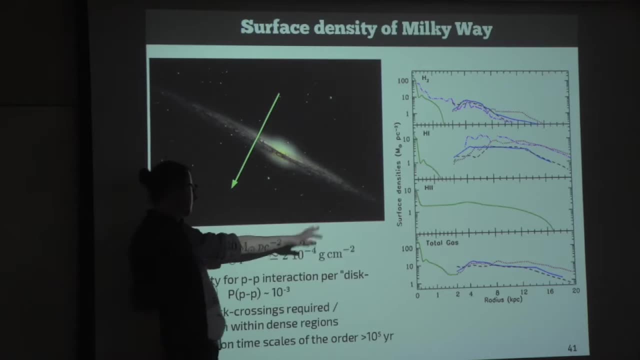 If you look through the Milky Way. this is plotted here. there are various contributions to the gas. I don't have time to go into details, but it's usually of the order of 10 to minus 3,, 10 to minus 4 grams per cubic centimeter, per square centimeter. 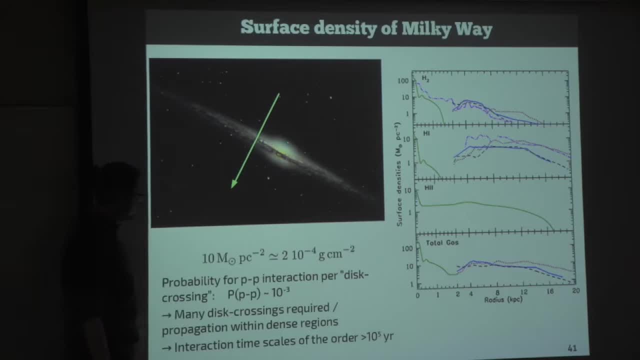 So if you go once through the anti-galactic disk, this is the amount of material that you hit. And if you multiply this with a cross-section, spallation, cross-section, the probability that something interacts, The proton-proton interaction, is about 10 to minus 3.. 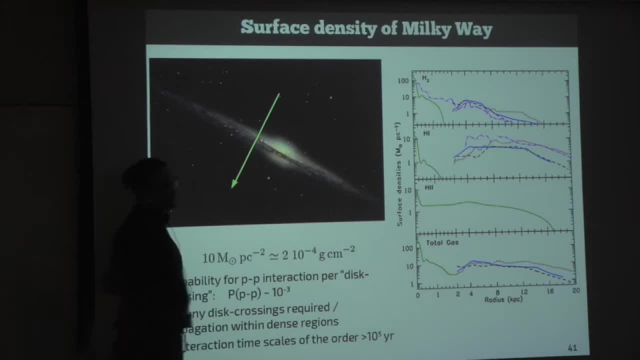 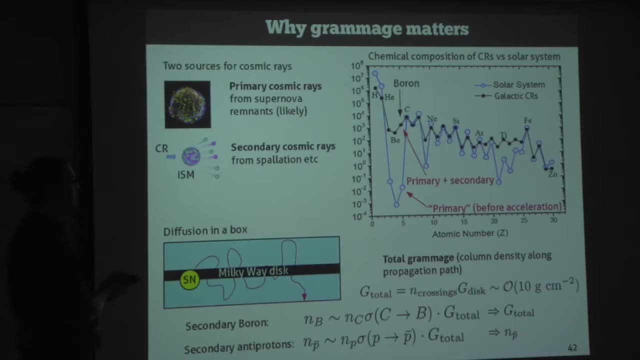 So for proton-proton interactions to happen, a cosmic ray has to go through the galactic disk quite often, And interaction timescales are of the order of hundreds of kilo-years or mega-years. So why does this all help? Well, why gramage matters. 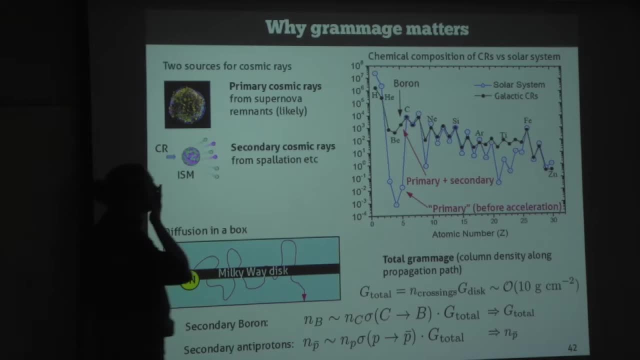 That's the story, So why can we say anything? So the main reason is that there's a distinction, as I already said, between primary cosmic rays that are accelerated in the primary sources, whatever they might be, and then the cosmic rays that are generated in the interstellar medium. 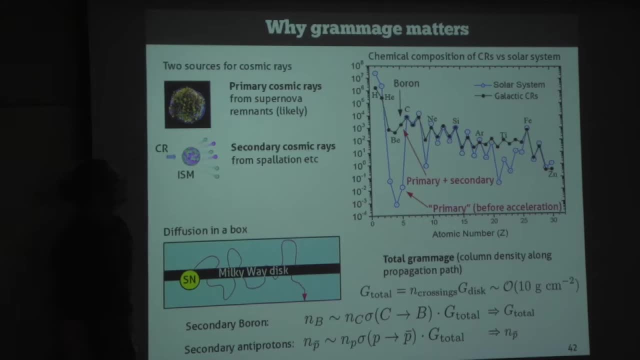 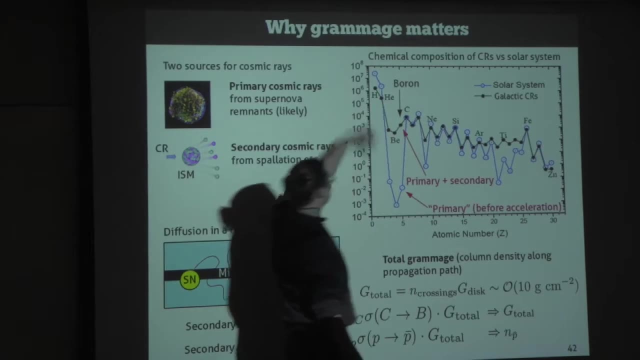 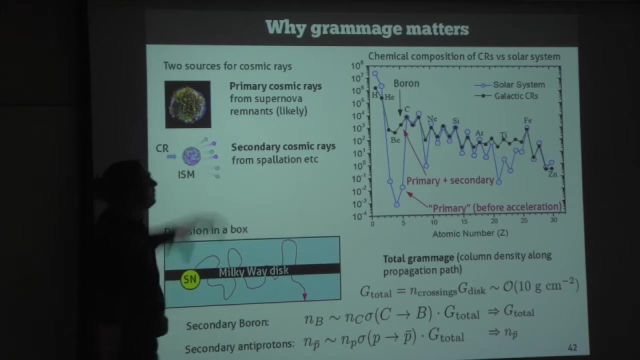 And the nice thing is that there is actually a difference in the chemical composition. So this plot here the blue line shows the composition, the chemical composition, It's basically the number, density for different function of the atomic number of material in the solar system. 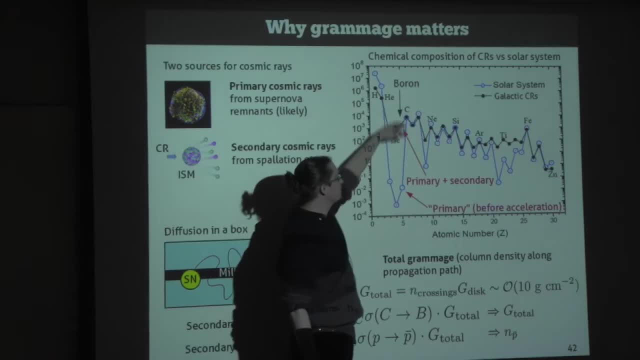 And that's also thought to be the distribution of the chemical composition. Okay, So this is the distribution of primary cosmic rays, because everything is accelerated, that is around, And you see that there would be lots of carbon, or that you expect lots of carbon as primary. cosmic rays but almost no boron, simply because that's not very abundant in the interstellar medium, So it cannot be accelerated. However, the secondary cosmic rays don't care about what's abundant in the interstellar medium. You just produce anything that you can produce. 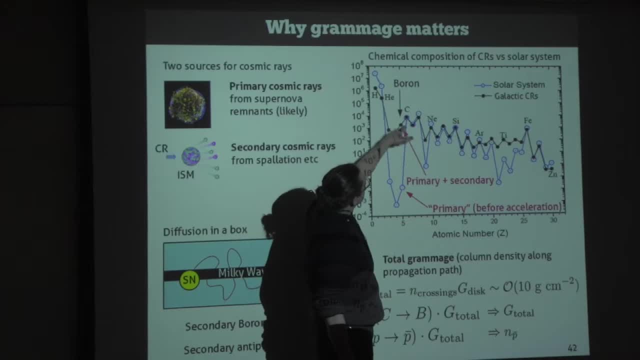 And among this you have all the cosmic rays And you have also boron. So this is the black curve actually shows the galactic cosmic rays and they have much more boron than you would naively expect. And these are basically all spallation products. 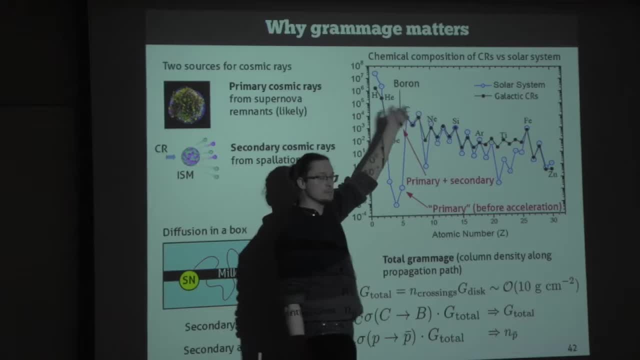 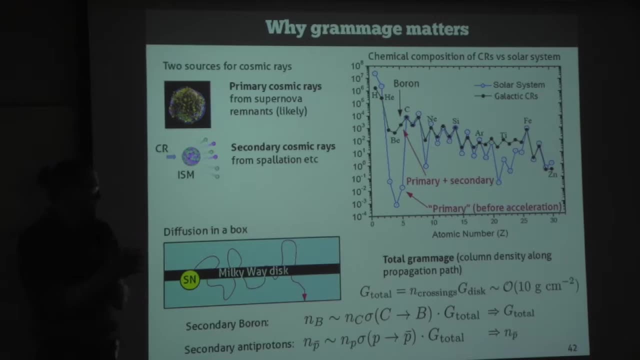 There are also spallation products contributing to carbon, but this is only a tiny fraction, so it doesn't matter too much, And the nice thing is that this now helps to actually say something about, for instance, the grammage. So what is the grammage? 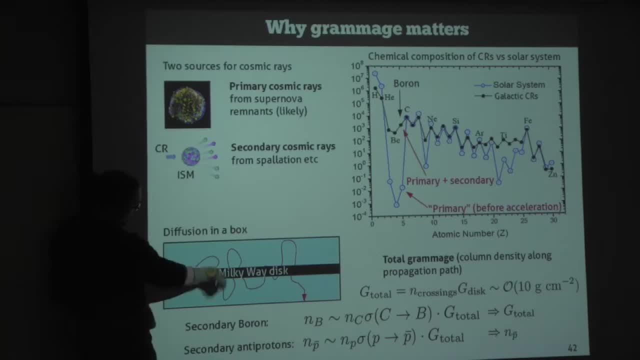 You have here supernova remnants accelerating cosmic rays, So you have the supernova remnants accelerating cosmic rays. And then you have the supernova remnants accelerating cosmic rays, So you have the supernova remnants accelerating cosmic rays. So you have the supernova remnants accelerating cosmic rays. 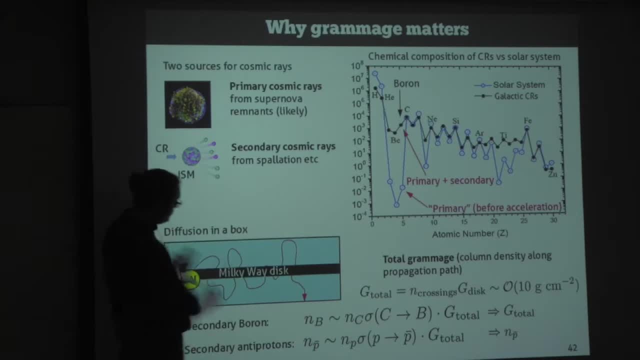 Which would go back and forth with the galaxy with a diffusive halo and then at some point escape from the diffusion zone, And in this process it would cross the disk a number of times. So let's call this number of crossings And, as I said, a bunch of slides earlier. this is universal for particles with a specific 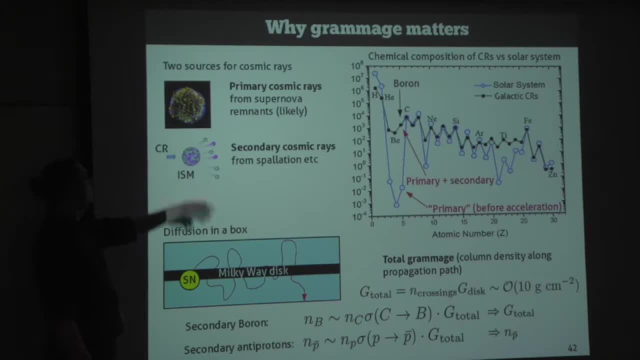 rigidity. So this could be iron nucleus or carbon or boron. If it has the same rigidity, it doesn't matter. same rigidity, it would start in the same direction at the same time. then it would have the same number of crossings. So you can learn something from the crossings that 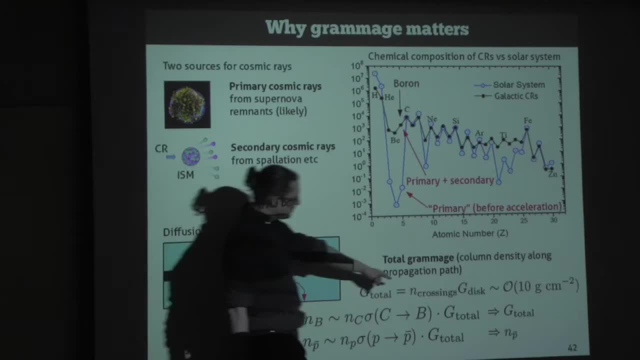 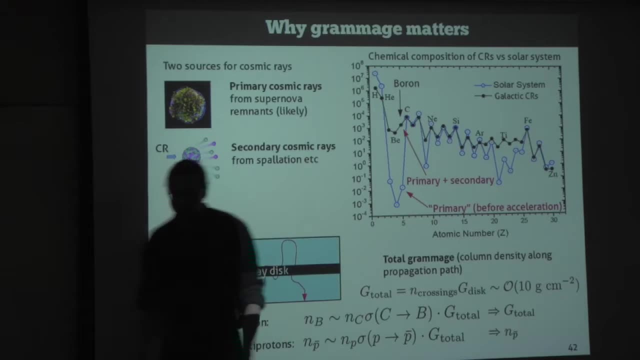 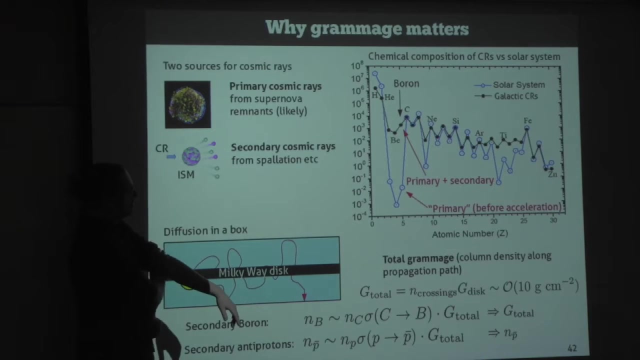 one particle has about the crossings that another particle has, And the total number of crossings times the thickness of the disk gives you something about the grammage. So this is the amount of material a cosmic ray encounters on average while it's propagating in the disk before it escapes, And that's of the order of 10 grams per square centimeter. 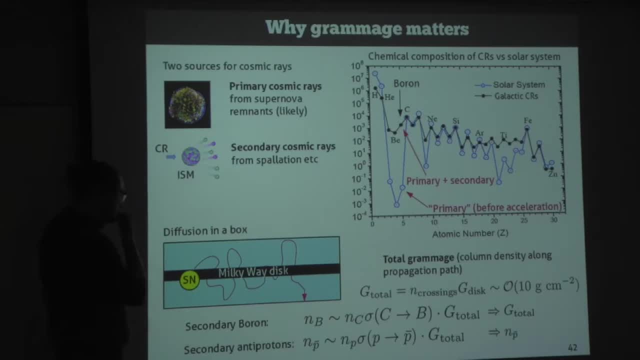 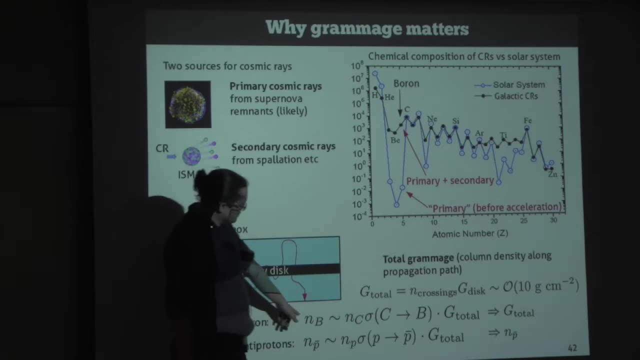 And how can we get to this 10 grams of square centimeter? Well, the trick is now we look at the density of the flux of boron cosmic rays. This, we know, is proportional to the number of carbon cosmic rays. If you ignore everything else, all the borons will be produced. 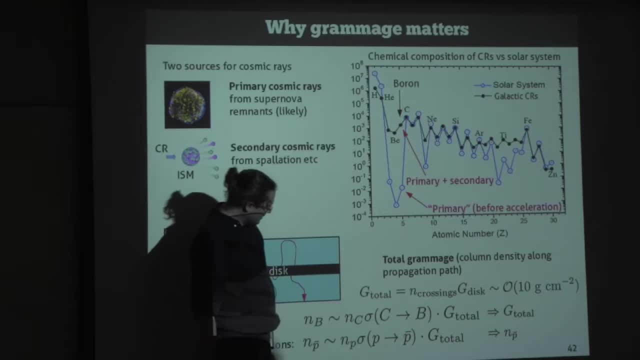 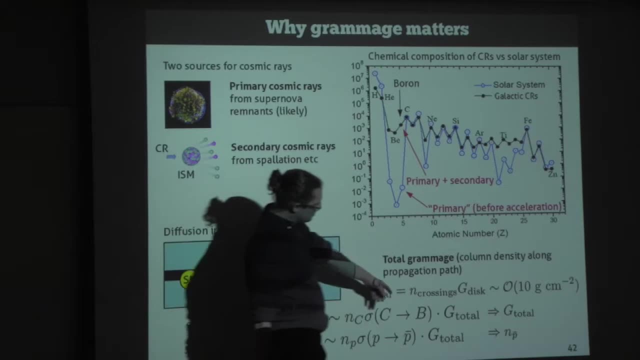 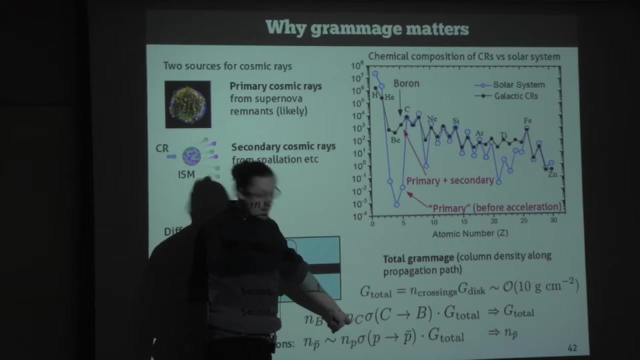 by spallation of carbon. So this is proportional to each other and it should be proportional to the production cross-section of carbon goes into boron and it should be proportional, of course, to the target material, so to the grammage And we can measure the carbon flux. 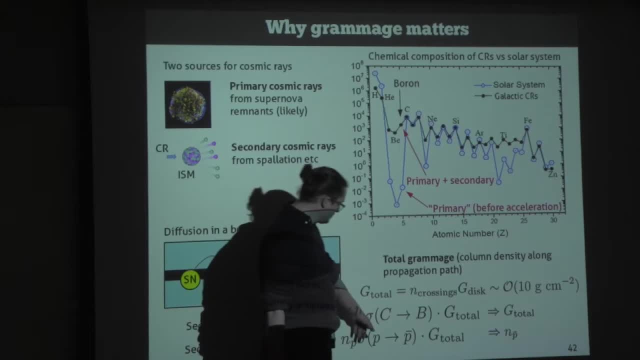 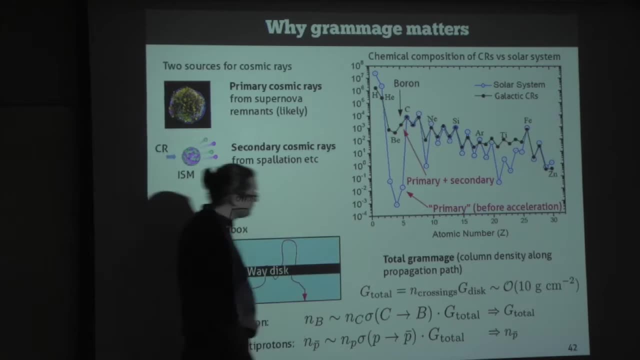 we can measure to a certain extent, or calculate or fit to experimental data the production cross section for boron from carbon, and so we can measure boron. and so if you plug this together, we learn something about the grammage. There are some pre-factors. 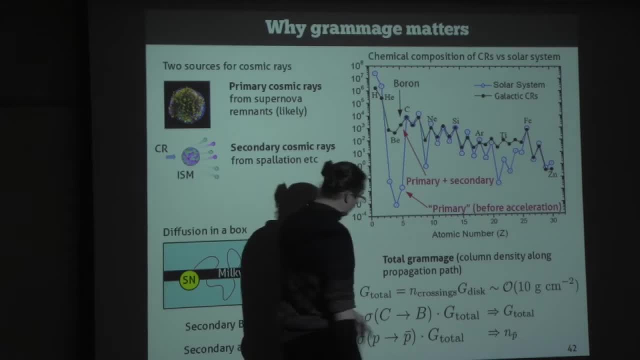 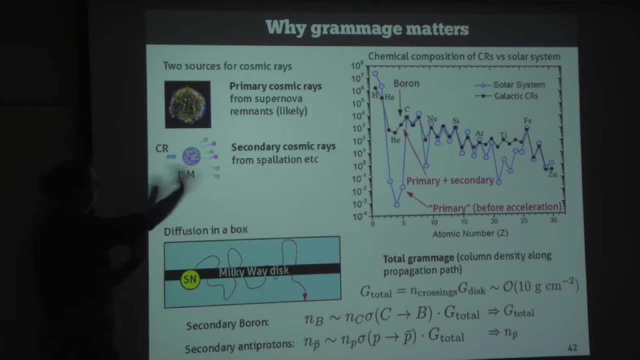 to take into account, but in this way we learn something about the grammage of particles with a specific rigidity. So again, if carbon nucleus would be disrupted and spallate, produce boron, then the boron would have the same rigidity, divided by a number of nucleons. 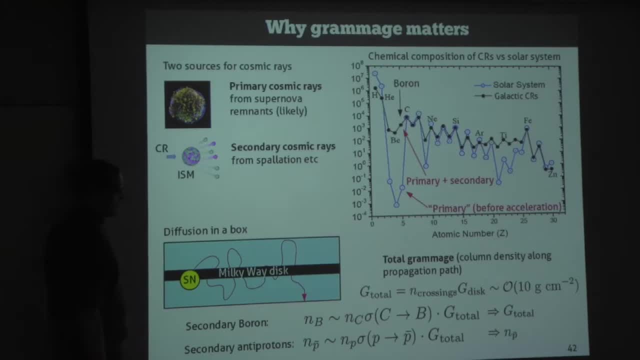 as the initial carbon nucleon had. So in this way we learn something about the grammage. so this number here It's all just conception. so the details of the numbers don't matter, but it's about the basic idea. So in this way one can 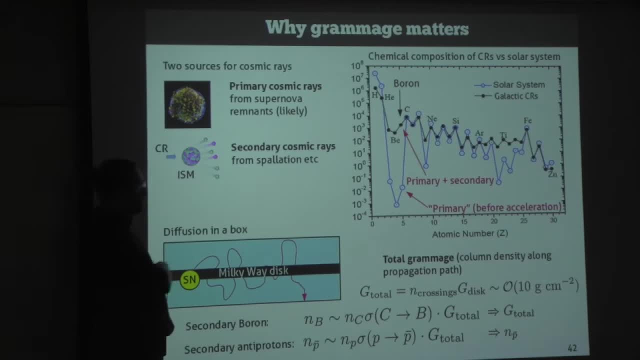 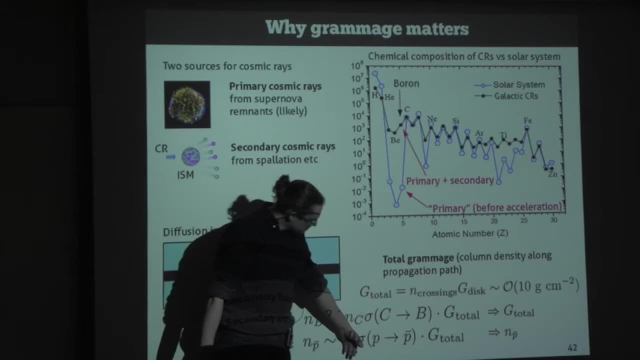 learn something about the grammage, and then one can use this to predict other things. So we have now the proton flux that we measure. we have an idea what's the proton to anti-proton cross-section. so proton hits, proton produces anti-proton. 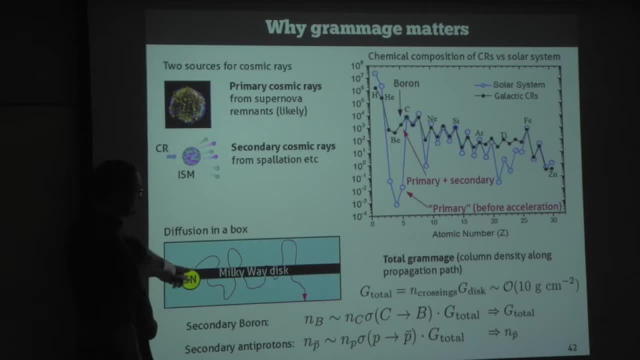 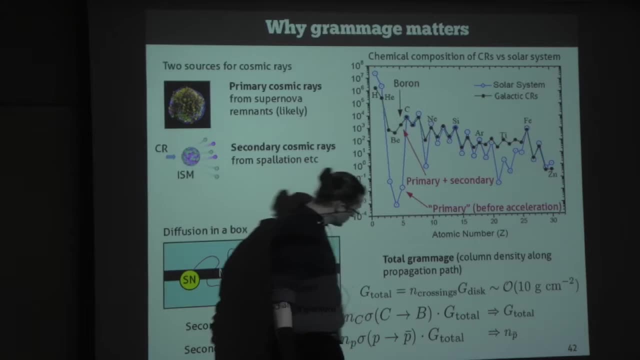 and the grammage should be the same for protons as for for carbon, as long as everything is relativistic right. So we can use the grammage that we measured from boron to carbon to predict the grammage relevant for anti-protons, and in this way we get. 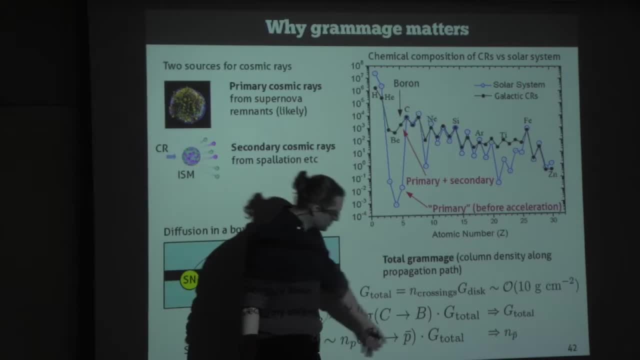 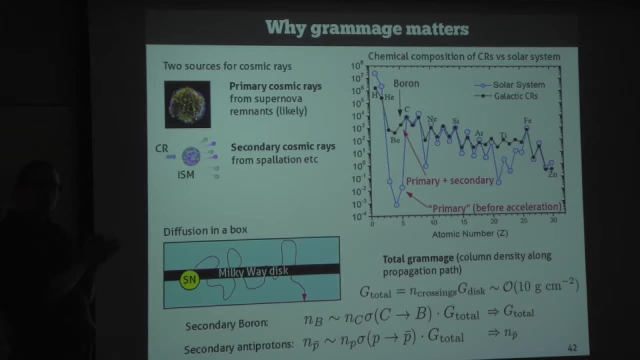 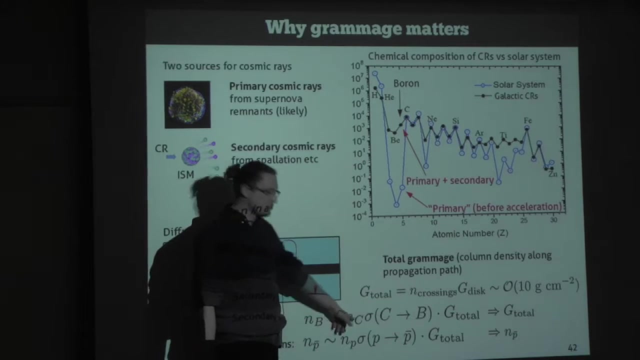 from the measured proton flux, the production cross-section and the grammage prediction for the anti-proton flux. So, in a nutshell, that's the reason why we can predict anti-protons by looking at at the boron to carbon ratio. So the entire trick is now to measure cosmic rays. 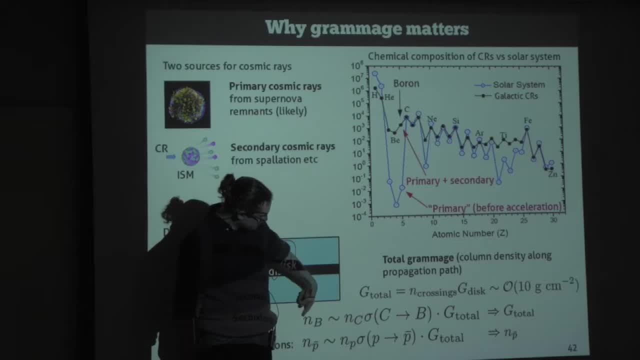 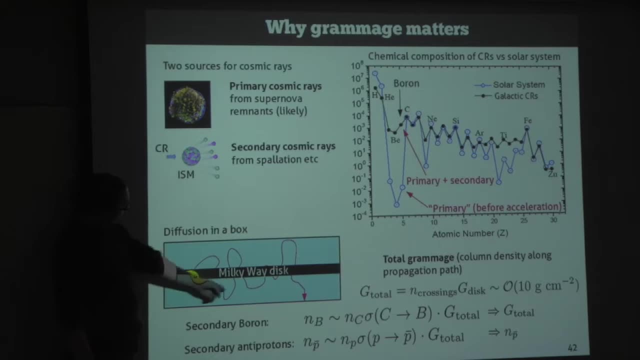 as functional for different atomic numbers and then just plot the number as the boron flux over carbon flux, adjust your model that models how cosmic rays propagate through the disk and how they scatter, to match the boron to carbon ratio and then magically you get a prediction. 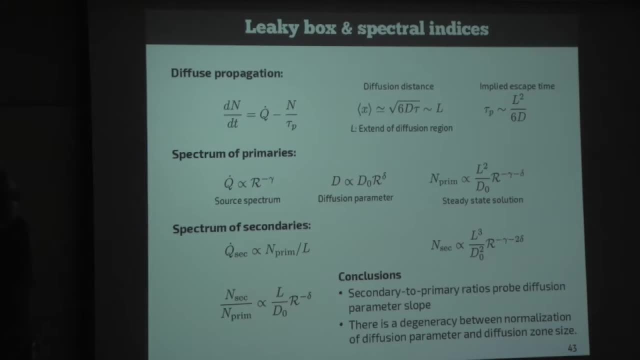 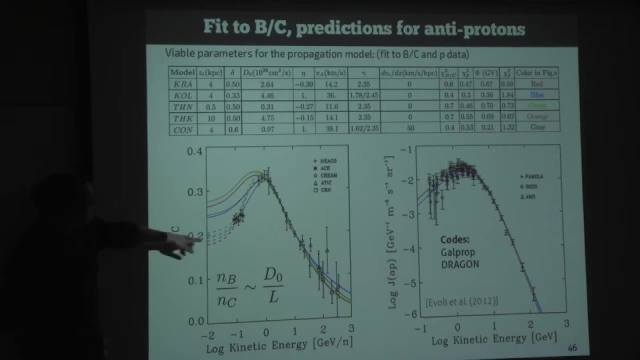 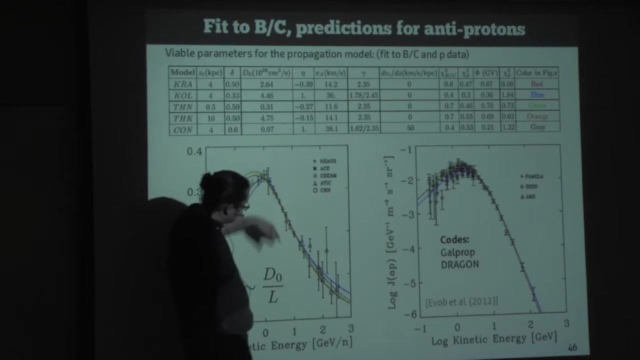 for anti-protons And this works pretty well. I'll just show you first that this works pretty well. So this is a fit to boron over carbon. You can get like differences here where you don't have much data, but as soon as you have a model that fits this, 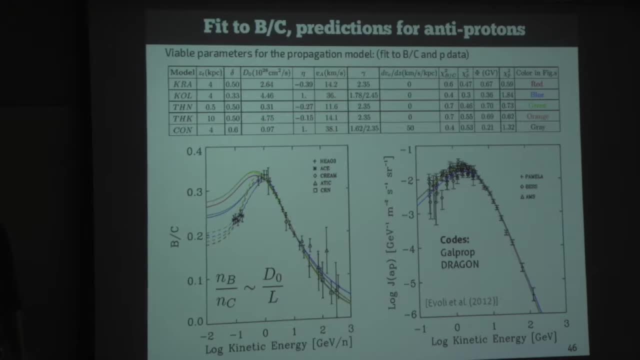 you get actually pretty good prediction for anti-protons. Does this imply that all the secondaries are produced outside the secondaries? What about if you have some I don't know envelope, something I don't know? you know, in this source, you would have secondaries produced in the source. 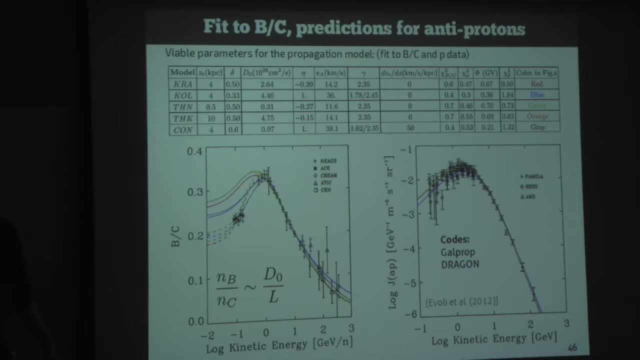 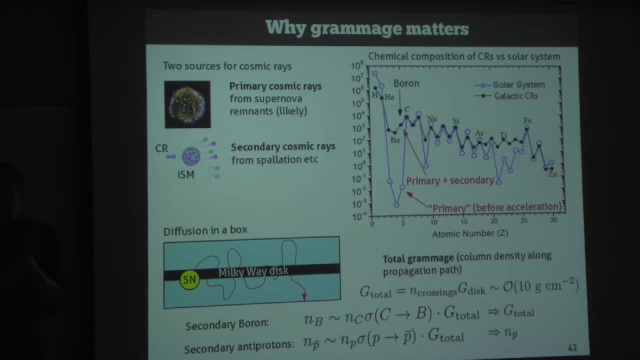 That's true. yeah, So this is like the. So you're assuming that the sources for the boron and anti-protons are the same, or? Yeah, that's exactly the. Is that an assumption or That's an assumption? It's an assumption. 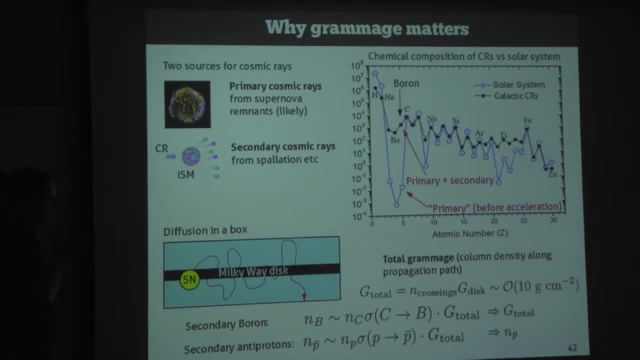 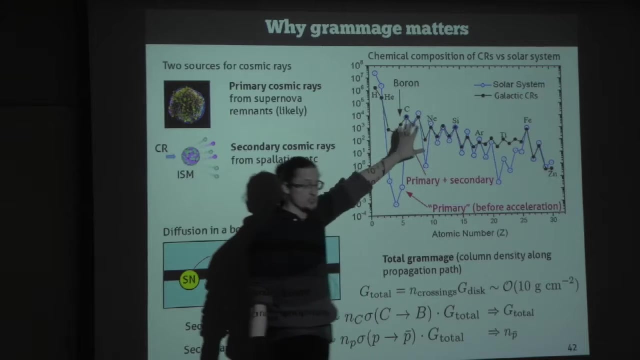 But they cannot hear. Yeah, I will repeat. So the comment was yes. so an important assumption is here that what happens in the primary sources is that that the chemical composition of particles in the industrial medium is not changed, They are just accelerated. 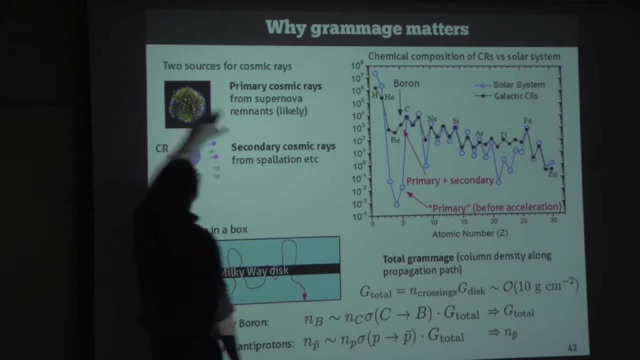 But still you don't produce borons. What still can happen is, now that there is enough target material in the supernova, remnant or surrounding that you already produce a significant amount of secondary particles in this initial step. This would change the entire picture. 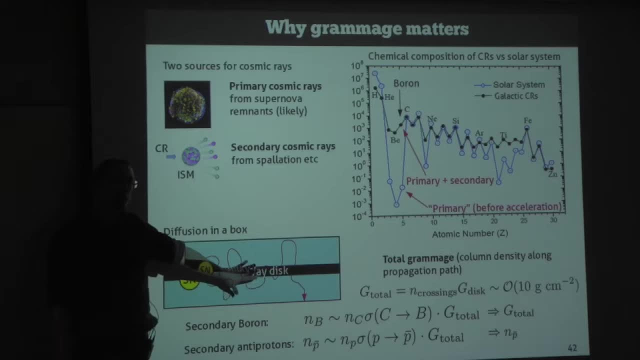 So then the simple explanation and connection wouldn't work. These are actually models that are also discussed and can be compared to data. But I mean, this here is the standard law And then if you see something that deviates from the predictions that you get here, 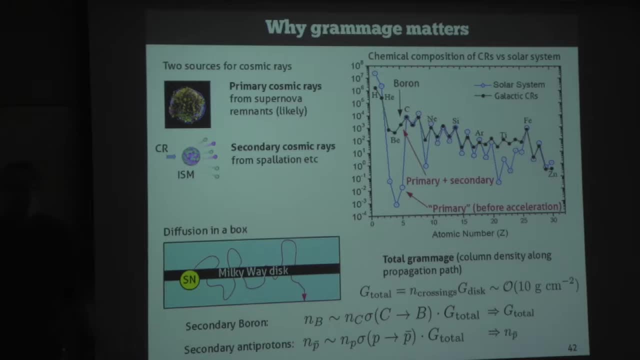 then what you were saying is a possible explanation under some circumstances, And this only applies for galactic cosmic rays, right? This only applies for galactic. Can you repeat the question? Yes, So this is a discussion about galactic cosmic rays. 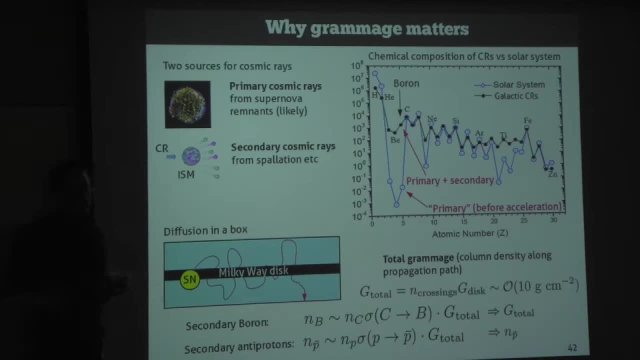 So the extragalactic ones are thought to kick in at much higher energy usually. So this is something that is only concerning galactic dynamics. Yeah, I think maybe you could repeat just part of your explanation here. I'm wondering why the solar system? 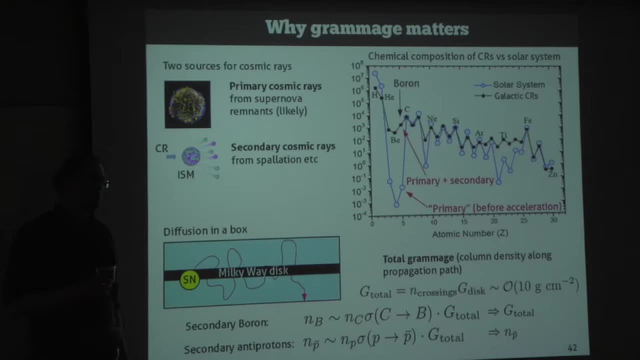 Why would you see primary cosmic rays in the solar system if they're presumably produced outside, Like? why would the galactic cosmic rays take half the secondary, the secondaries, where the primaries would be in the solar system, when I feel like the supernovas are outside? 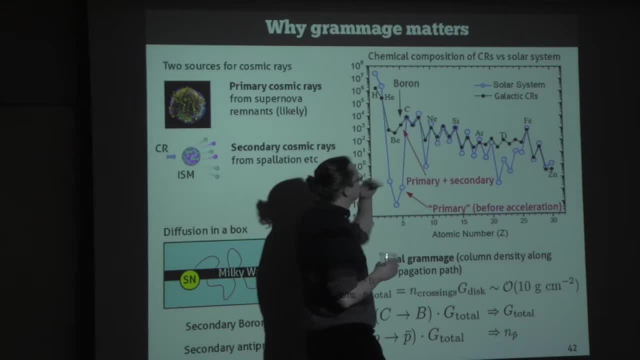 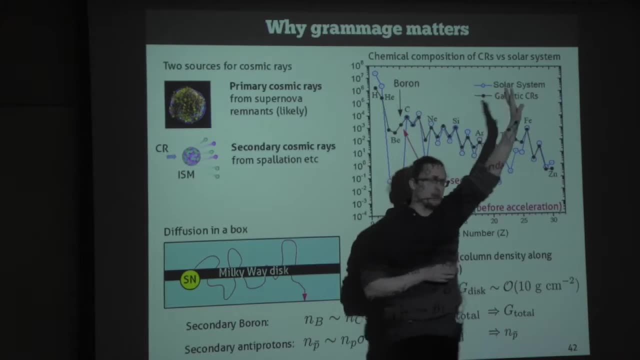 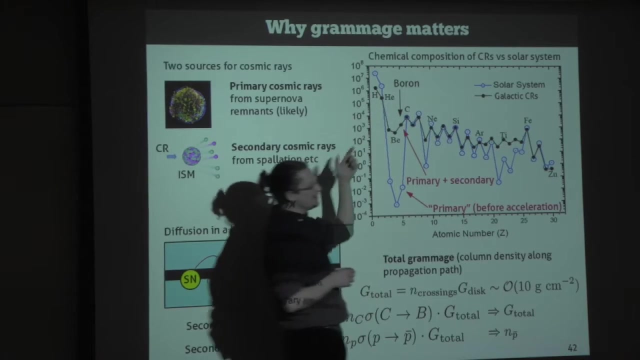 I feel like I'm just confused. Okay, So the reason why? One more question, please. Okay, So the reason why The question was, I think, why solar system abundances matter for the primary cosmic rays, right, This is simply because solar system abundances are tracing to a reasonable extent. 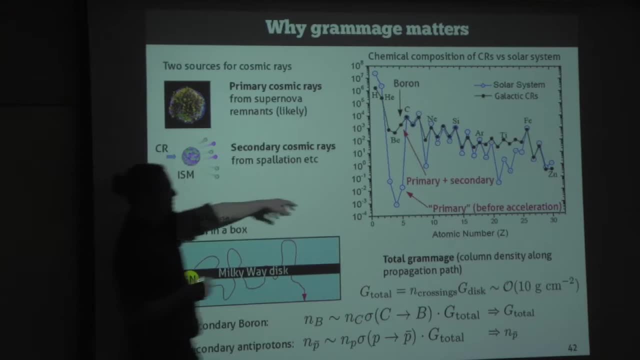 the abundances in the interstellar medium. So this is a statement about the interstellar mediums. Boron is not just very prominent in the interstellar medium and hence also cannot be accelerated if it's not there, But it's much more prominent in the cosmic rays. 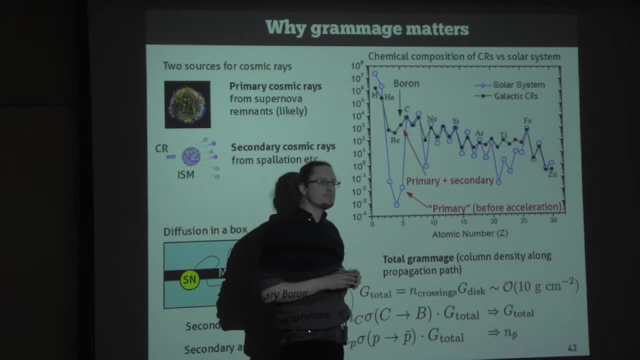 So that's the entire logic. So if you measure solar system abundances, they look like this blue curve where boron doesn't play any role. If you measure cosmic ray composition, you measure much more. Now the assumption is simply that, okay, maybe in the interstellar medium. 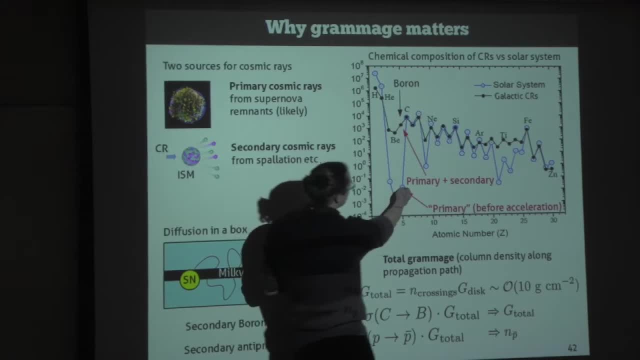 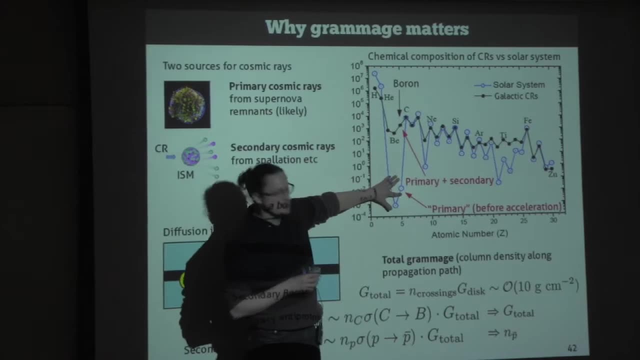 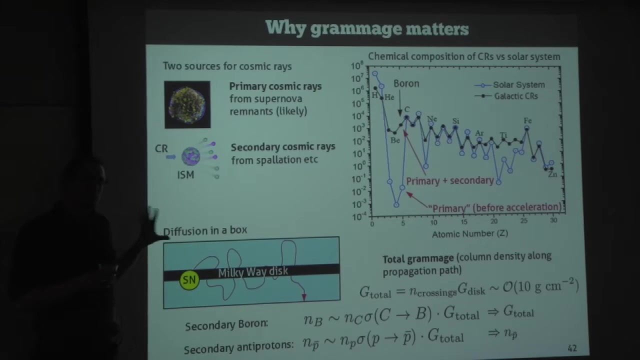 the distribution will be somewhat different from the solar system, but probably boron will not be abundant by five or six orders of magnitude more abundant, And if there is a small difference here this doesn't matter. This doesn't change the argument, And again I should emphasize that this is like the easiest possible explanation of the entire story. 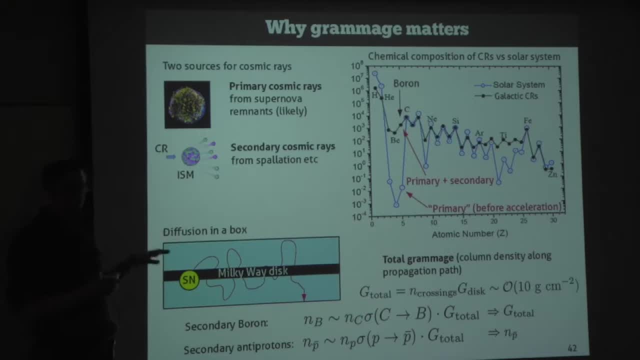 So there are lots of caveats, But I wanted to get to the bottom of why it works at all. I mean, then there are lots of reasons with concerns and caveats to this, But it's useful to understand the basic picture Good. 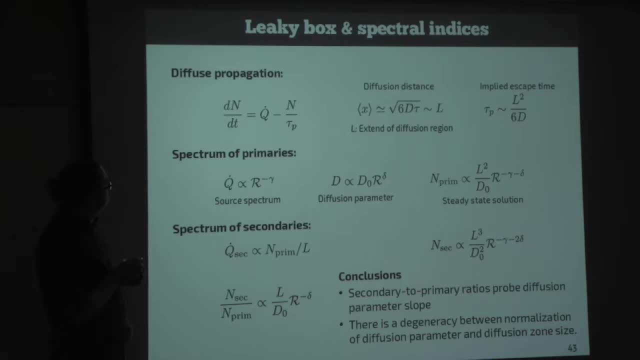 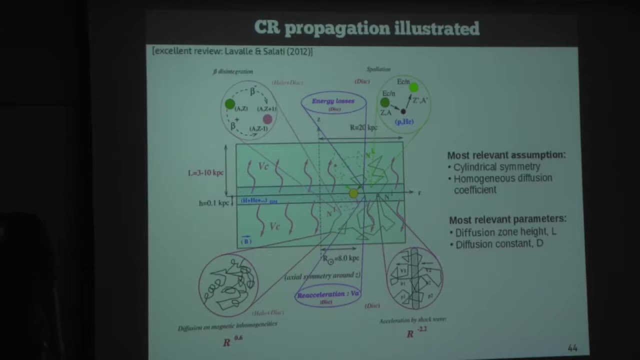 Then there is another aspect to this, Which can be very nicely understood by what is called the leaky box model. It's easier to first show this slide, actually. So now what is actually done is, instead of just playing with numbers, one can write down a complete model for cosmic ray propagation. 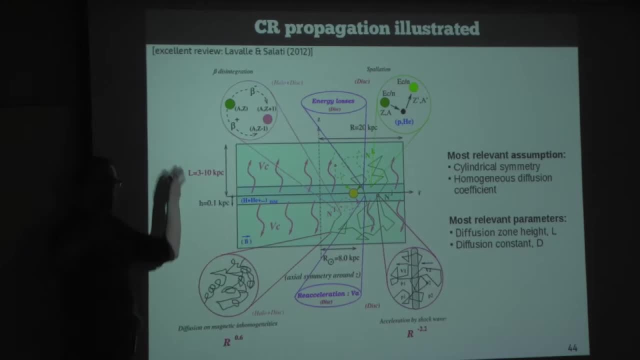 which would be usually- this is the traditional way how to do it- a box along the galactic disk which is here. You assume there is cosmic ray propagation happening inside and then free escape outside, And then cosmic rays can interact, That's when they hit interstellar medium in the disk. 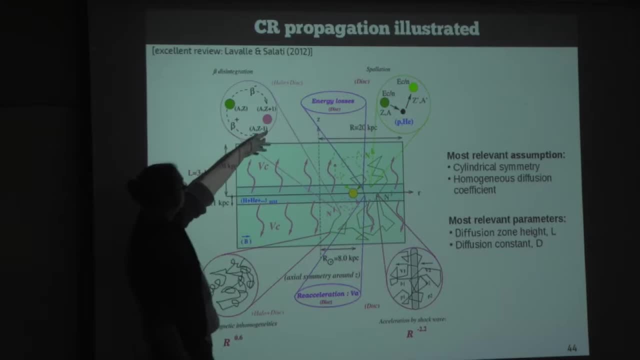 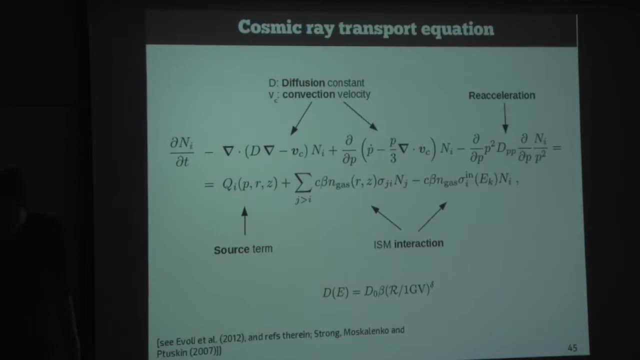 And then on top of diffusion one has to take into account energy losses, spallation processes, re-acceleration, convective winds and so on. So in the end this leads to a complicated diffusion re-acceleration equation with interstellar medium interactions and energy loss. 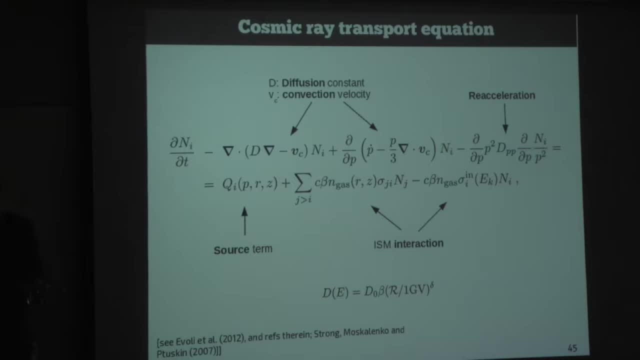 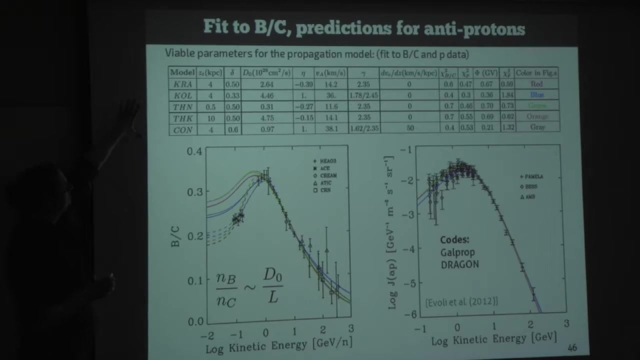 I just flashed the equation here, But you can identify individual terms like diffusion. This is the re-acceleration part, that is like a diffusion in momentum space, And this is interaction with gas. And what one can then do is one can basically fiddle around. 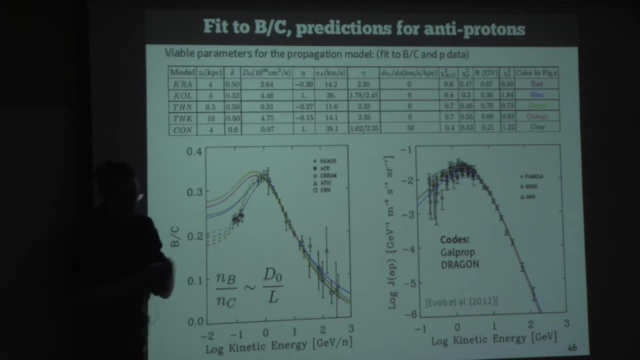 with the parameters of this diffusion equation, And this includes the height of the diffusion halo. This includes the energy dependence of the diffusion constant, the normalization of the diffusion constant and a bunch of other parameters Try to reproduce the boron to carbon ratio. 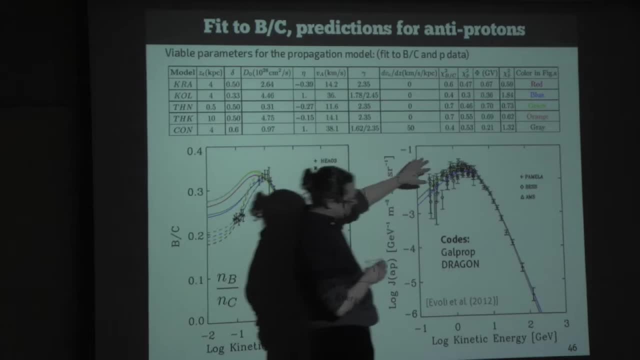 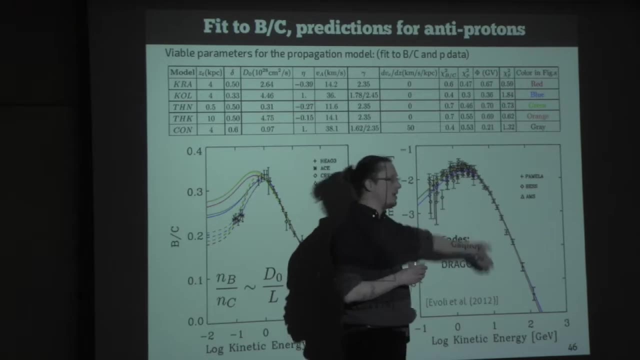 And then predict what you see in antiprotons And traditionally this worked quite well. So this is a comparison with PAMELA data And this works usually especially well, or is thought to work well, at high energies, where you have this universality in the propagation. 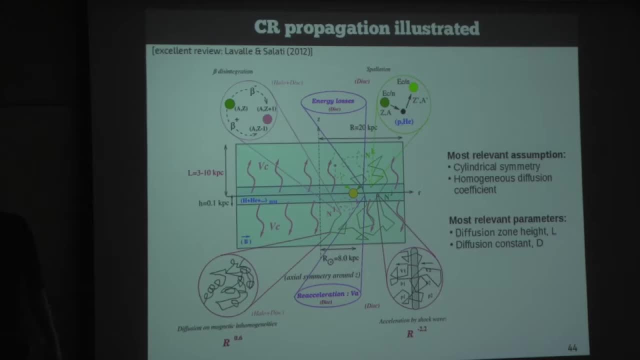 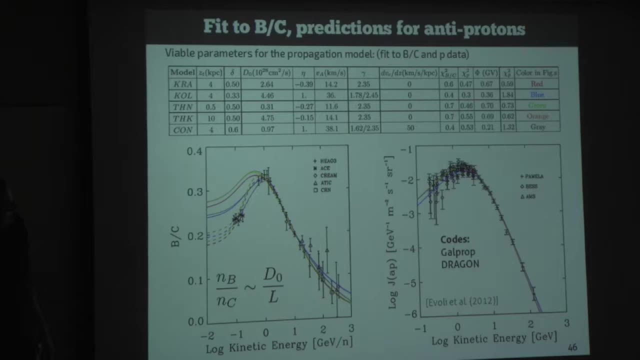 because only rigidity matters. Okay, to understand now a bit more what one can actually learn. So one interesting aspect is now: what can one actually learn from the slope here, So the boron to carbon ratio? Because the slope that you see here tells you something. 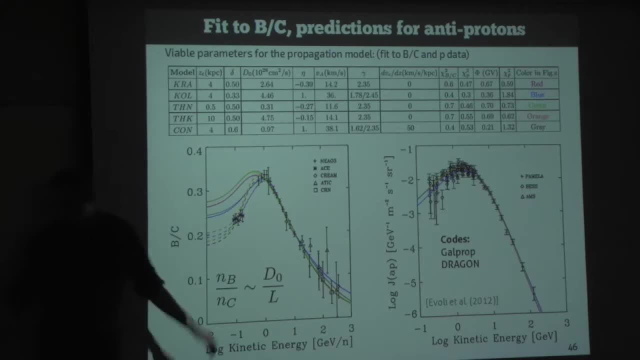 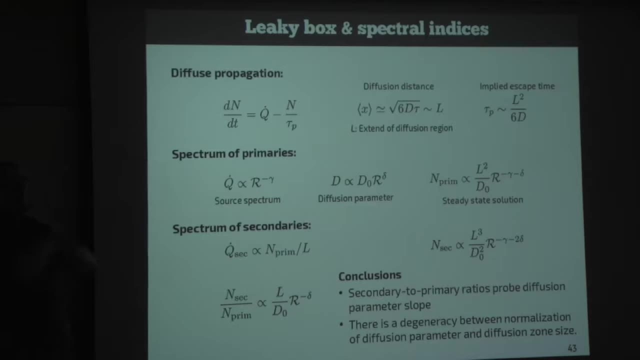 about the diffusion constant. I will just guide you through this leaky box model and then we go back to the full example. So now let's consider again an extremely simple scenario. So just a box, okay, Box with number of particles inside. 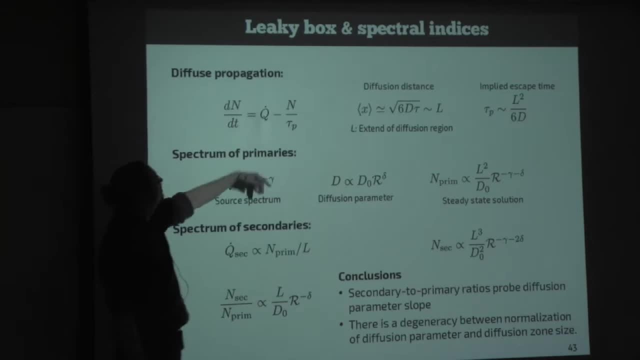 There's a source term. This is just the number of particles produced per time, And then there is an escape term. So this is the number of particles in the box And this is the lifetime of the box, And this is the lifetime of these particles. 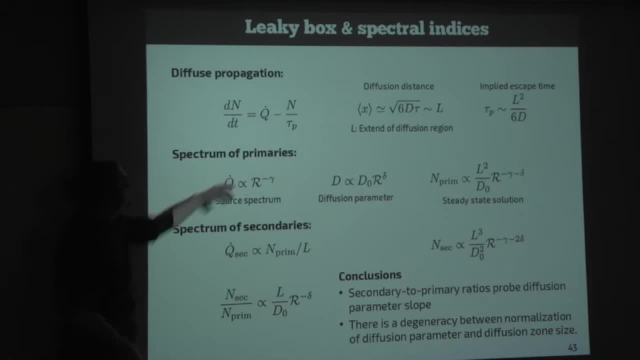 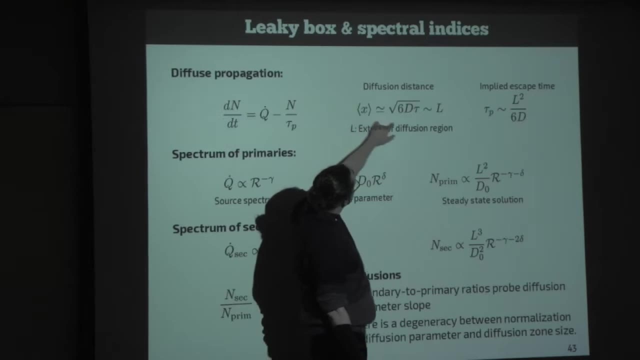 or the escape time, And that's a leaky box because they can leak out the particles And we can connect this to diffusion parameters as follows. So this here would be: if you have a diffusion process with a diffusion constant d, just a constant with the correct units. 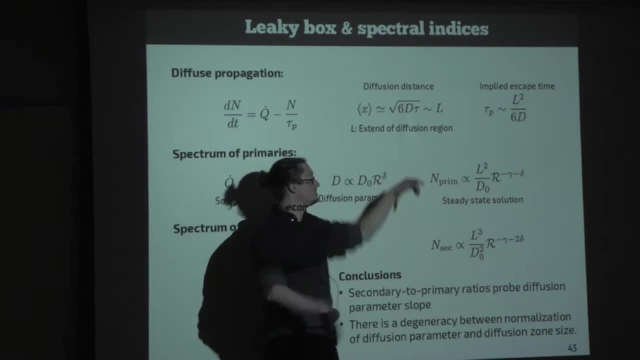 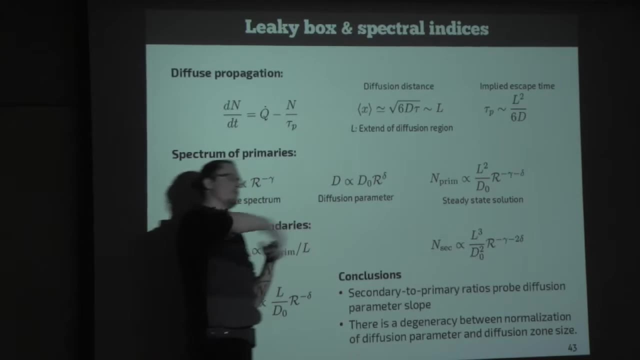 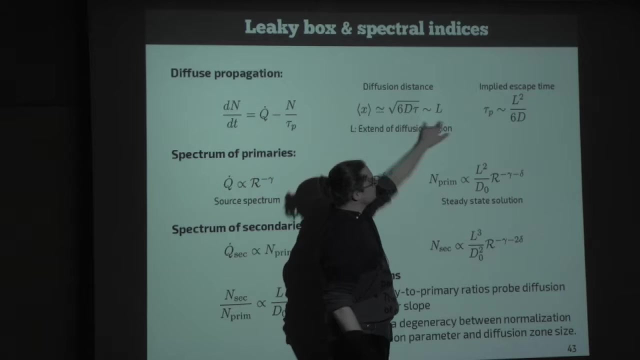 and some time tau, where the particles diffuse. they have diffused on average a distance x, So it's just given by this expression. They diffuse with the square root of time, basically, And then we can identify x with the extent of the box. 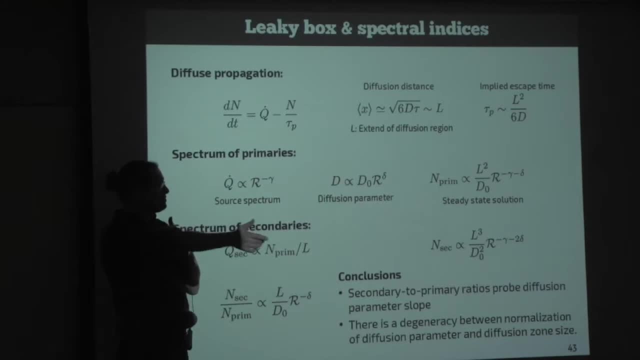 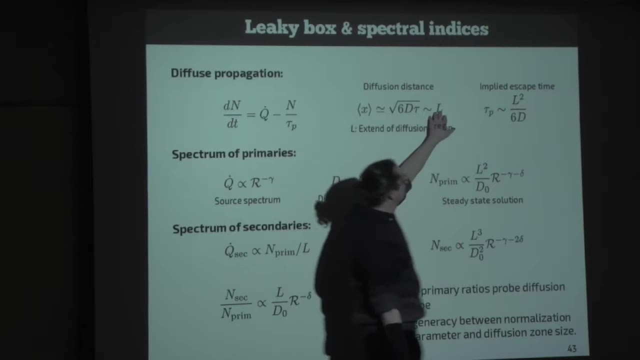 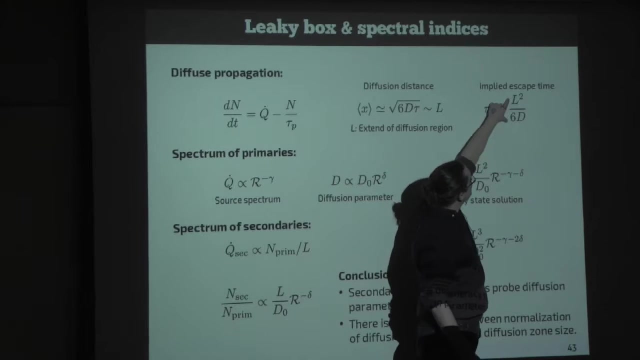 So let's say the box has a height, l and width and depth l, So we can identify l with this diffusion length and say, okay, the particle escaped when it hits the boundary on average. So this implied escape time is something like box size squared. 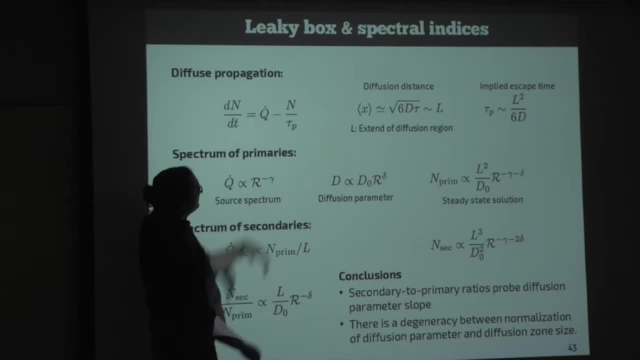 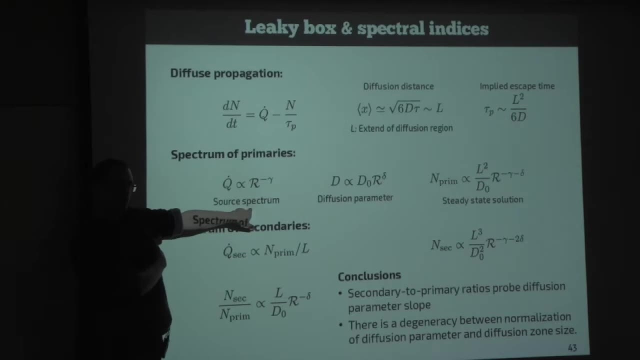 divided by diffusion constant, And then we plug this in here. We can do this And we plug a few other things in First source spectrum. So now we assume that the source, actually, that this is actually an equation that depends on energy. 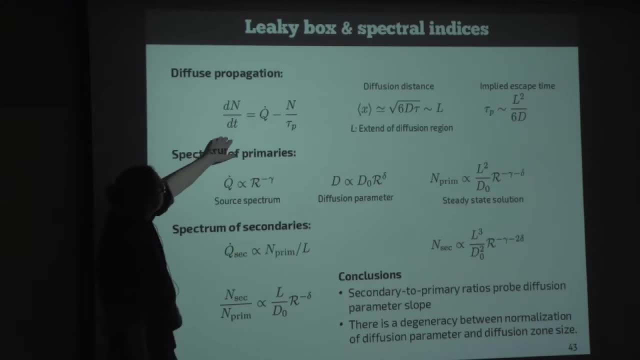 Energy losses don't play a role. So the only thing that plays a role is that the equation has different solutions for different energies Or, in this case, for different rigidities. So we assume the source spectrum is somehow proportional to rigidity, to the power minus gamma. 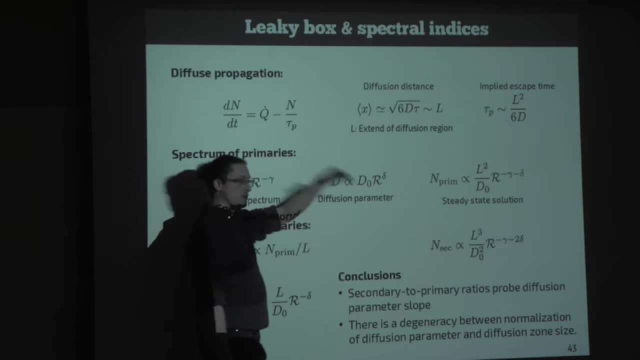 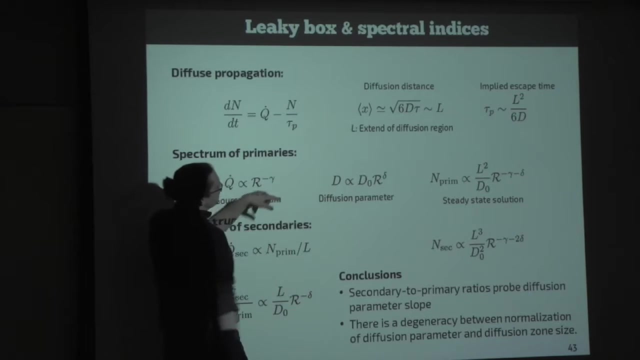 So it's just a power law, That the diffusion parameter is also a power law. So this is just a constant pre-factor And then something that grows with energy or with rigidity, And then we can just plug this in here and solve for steady state. 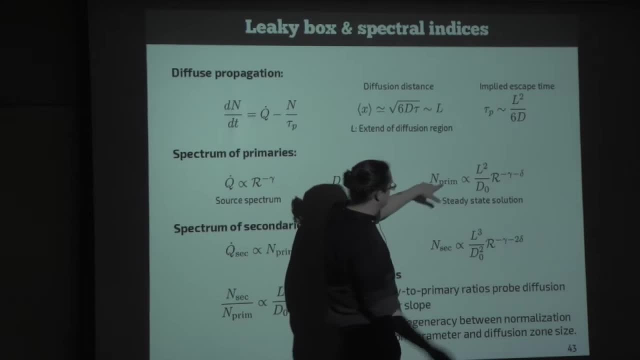 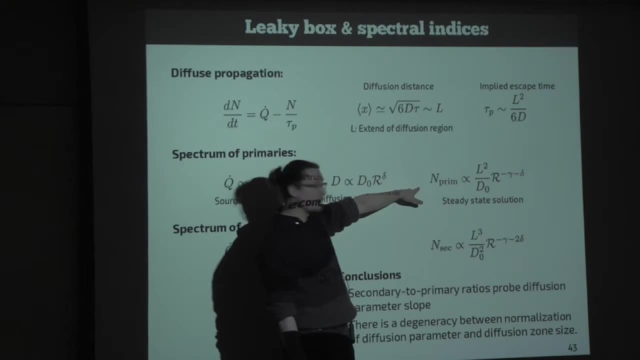 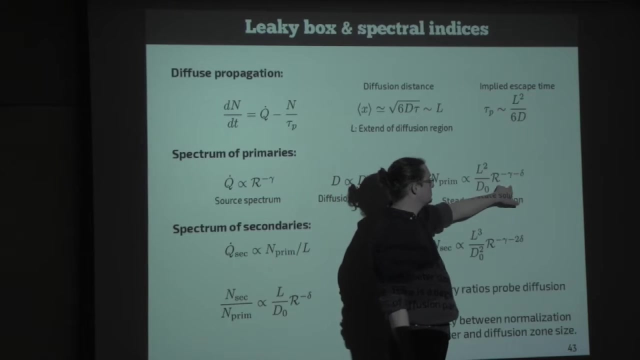 So set this to zero And then just move around some numbers And then we get the steady state solution. So the primary cosmic ray flux will depend on L squared divided by D times, and it will have this spectrum. So it will have the spectrum of the initial sources. 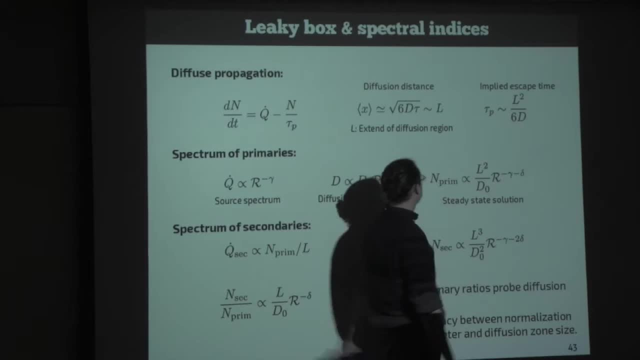 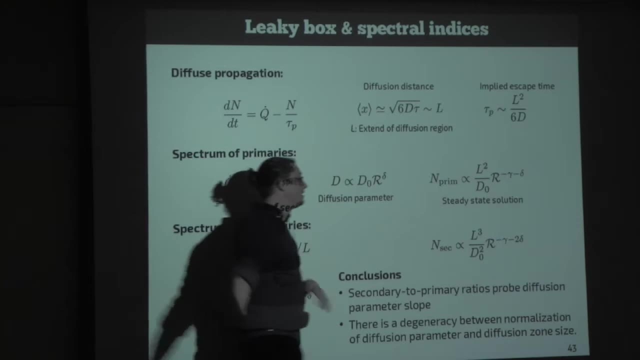 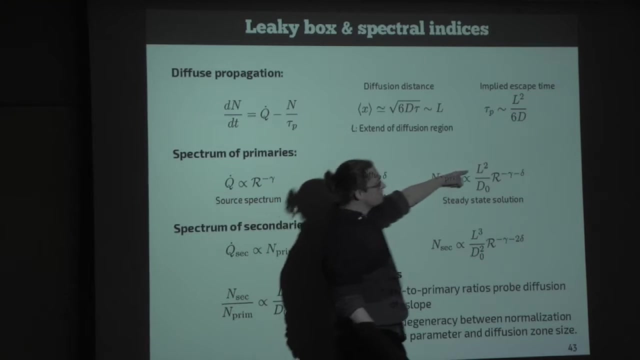 modified by the energy dependence of the diffusion constant. And that's not a surprise, because if higher energetic particles diffuse, faster they are lost faster, They escape faster, So you would expect to see less of them in the primary cosmic rays. Furthermore, if the box is larger, 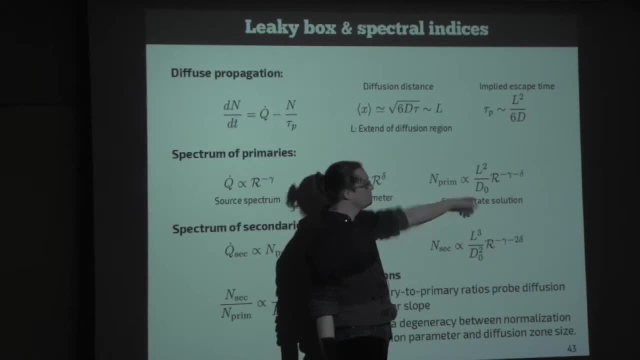 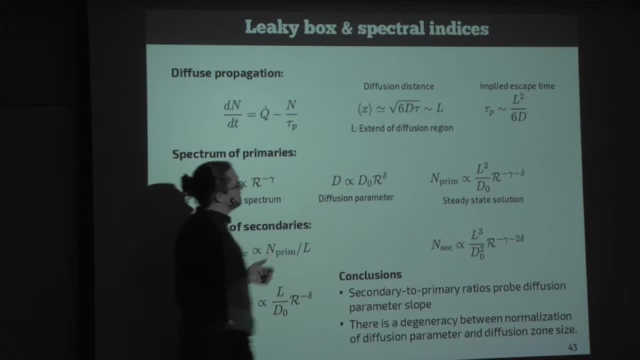 they will stay longer in. So you would expect more. If the diffusion constant is larger, again they can. So if the constant is larger, the pre-factor, again they can escape faster. So you expect less primary cosmic rays. So that's now a statement about the spectrum of the primary cosmic rays. 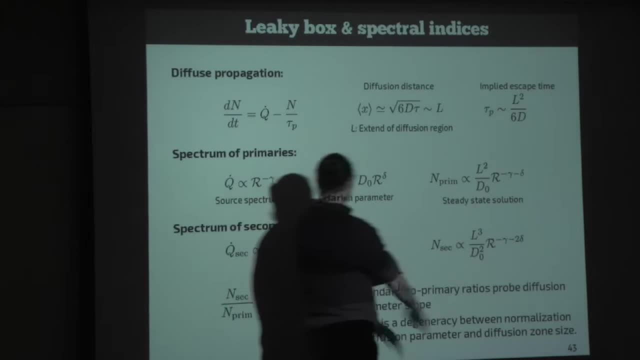 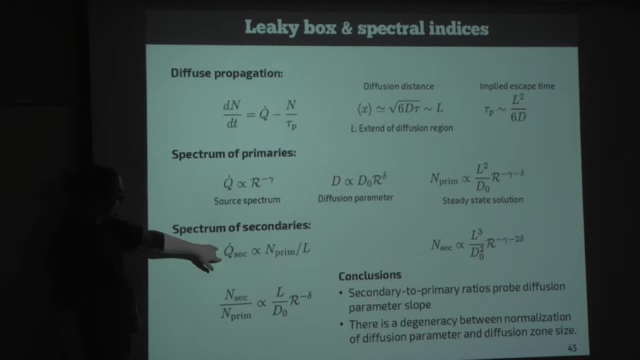 That doesn't help you much if you don't know gamma. But now what you can do is actually also look at secondaries. So the source for secondaries would be proportional to the primary cosmic rays. Right, You need primaries to generate secondaries. 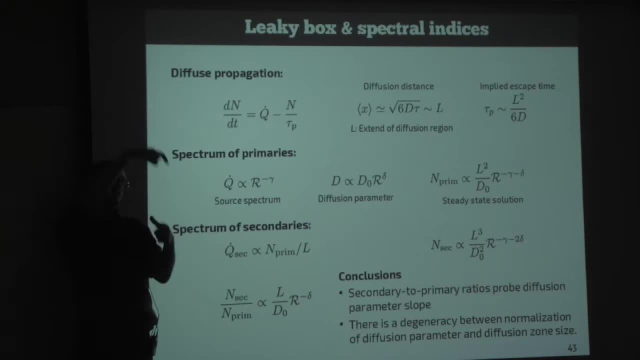 Divided by L, because we have this box And the probability that the particles, the fraction of primary particles that would be in a disk-like intersection in the box, compared to the probability to be anywhere else, is basically L. So that's the source term of secondaries. 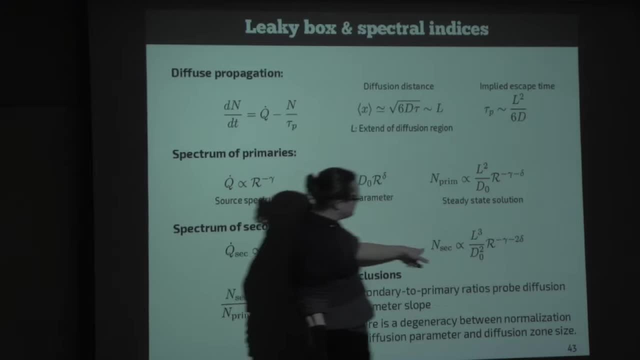 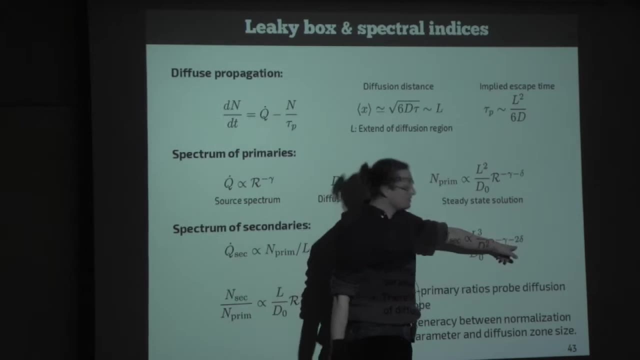 And then we can just plug this in again and do the same calculation and we end up with this here. So this is now the number density of secondaries, And you see that we start now with this spectrum and diffusion kicked in a second time. 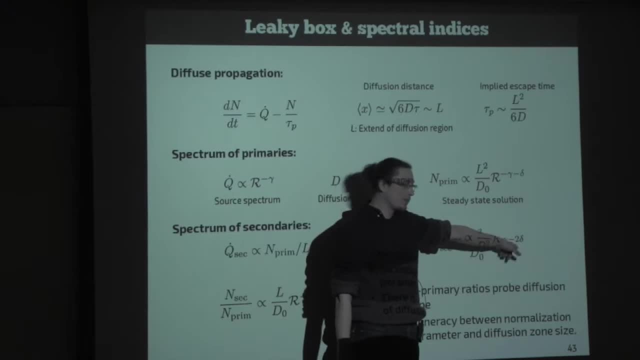 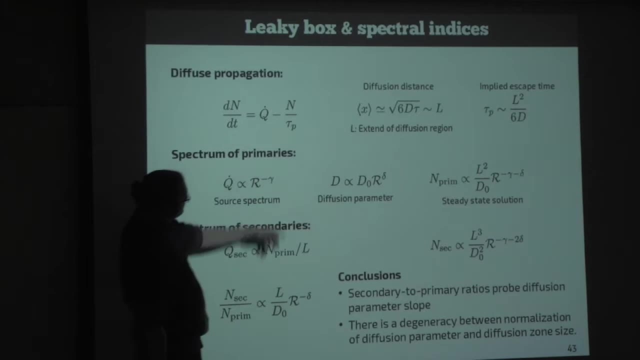 So now actually the spectrum depends on the source spectrum and then twice the diffusion effect. And if you now just write secondary divided by primary ratio, what disappears is the injection spectrum. So the primary spectrum doesn't matter, But what matters still is the effect of the diffusion. 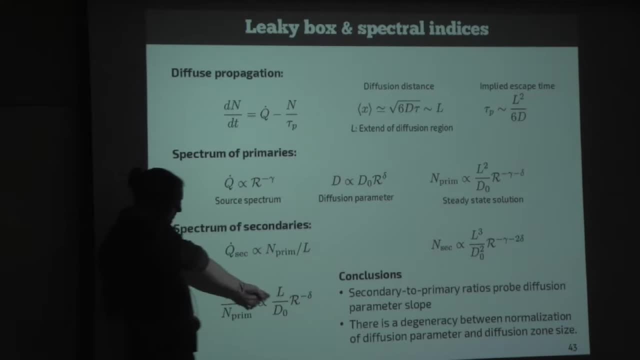 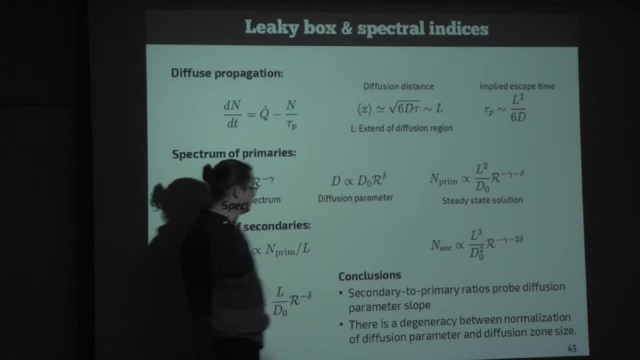 So secondary to primary ratio becomes proportional to rigidity, to the power minus energy dependence or rigidity dependence of the diffusion parameter. And on top of that we see that the normalization actually depends not only on L or D, but on both, on the ratio. 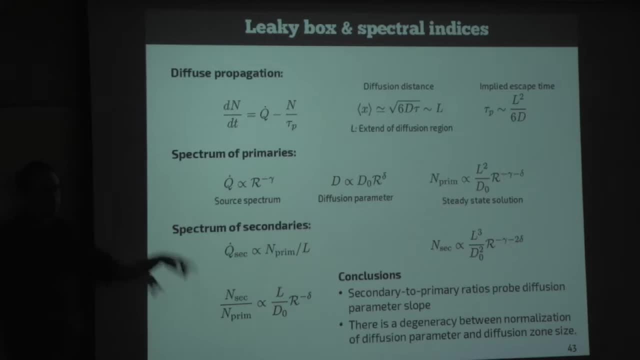 So, by measuring secondary to primary ratio, what one can measure is the slope of the diffusion parameter and this funny combination of the diffusion zone- height, basically- and the diffusion constant. I have a question. Yeah, Sorry, because I think it's very simple. 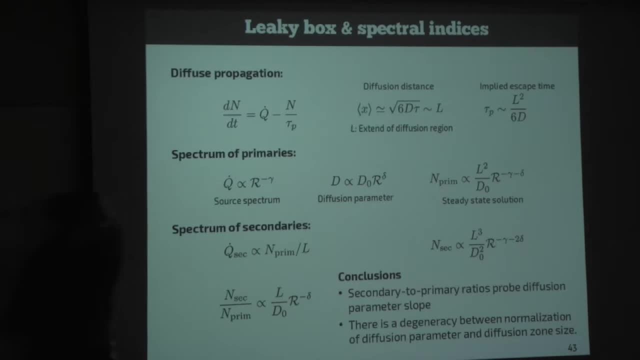 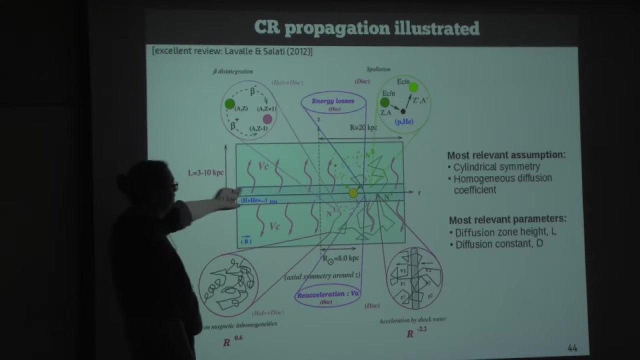 The diffusion? are we diffusing through this magnetic field or diffusing through other particles? So the question was where the diffusion happens. So the diffusion happens basically in this imaginary box. So the idea is that there is a region around the galactic disk. 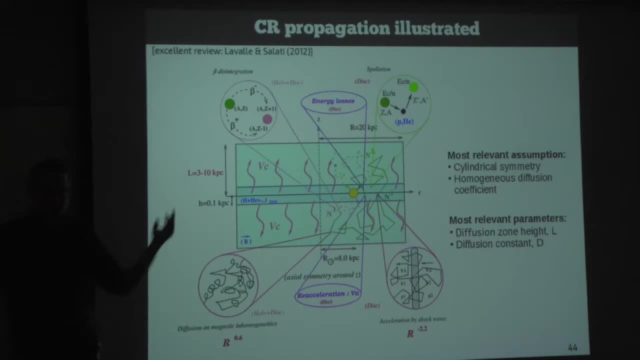 where the magnetic field is still turned, It's still turbulent And there diffusion happens, And then at some point this stops, So at some point particles can escape freely. So it's diffusing through a magnetic field. It's diffusing through a magnetic field, yeah. 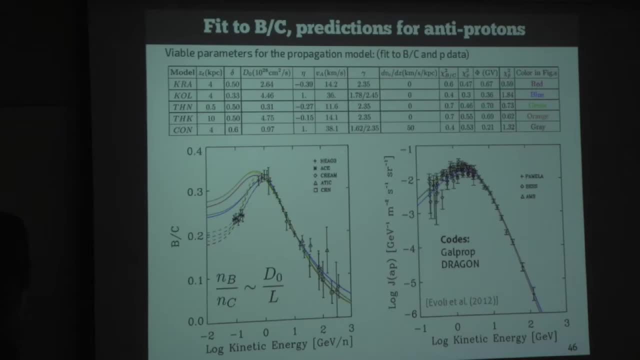 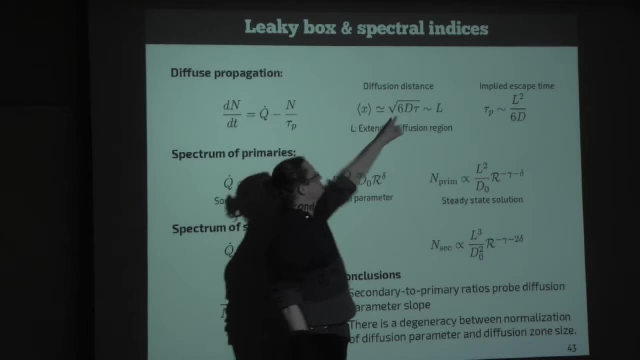 So when there's a factor of six in the equation, that sounds like maybe translation to the rotation. It sounds like I think this factor of six, if I remember correctly, just comes from the fact that this is a 3D thing and how you define the diffusion constant. 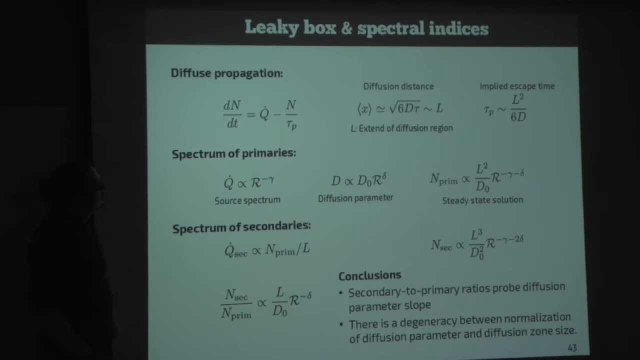 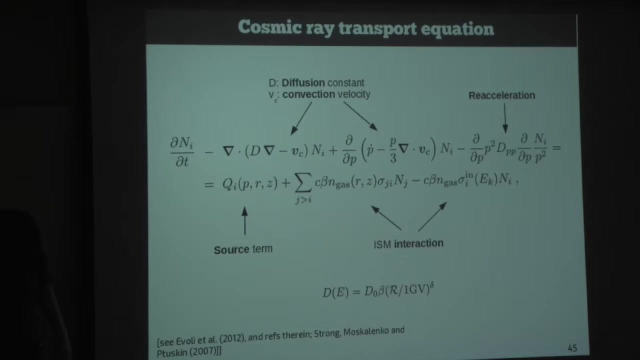 So you could also absorb it, OK. So questions about this. It's a very simple, nice story. If you have to think about the indices and powers again, it's worth it because this explains you already a lot. It tells you a lot about what you can easily measure. 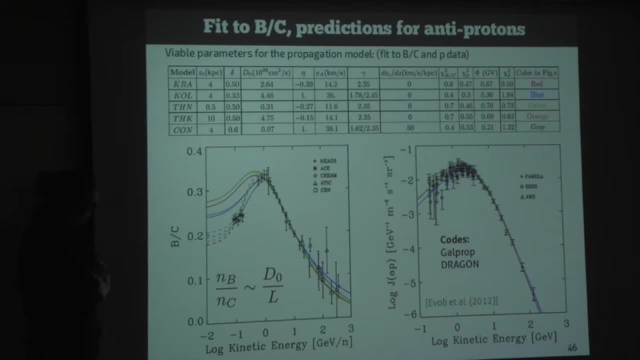 and what you can't easily measure in cosmic rays. But OK, The story is now we have boron to carbon. This tells us something about the slope and this ratio, But in particular it doesn't tell us anything about the height of the diffusion zone. 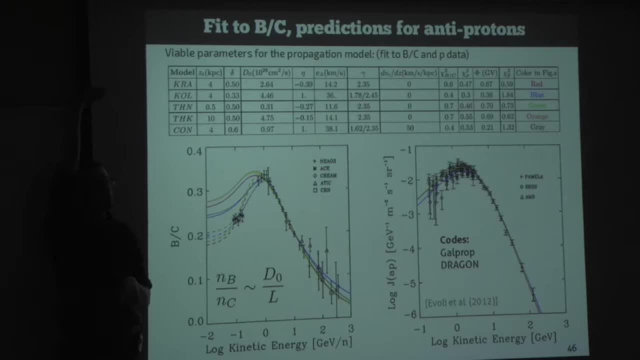 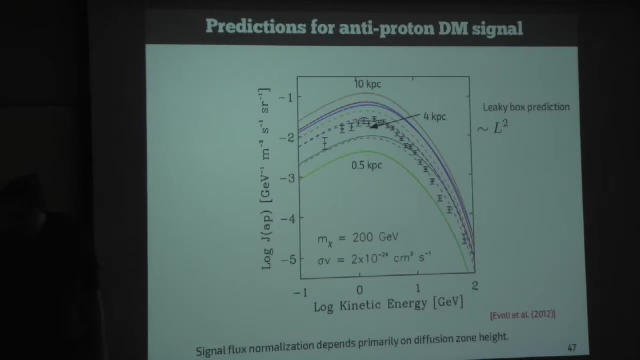 So the height can be like tiny in principle, or it can be huge, And on top of that we get the nice prediction for antiprotons. So one problem is now that the signal flux actually of dark matter wouldn't be that well constrained. 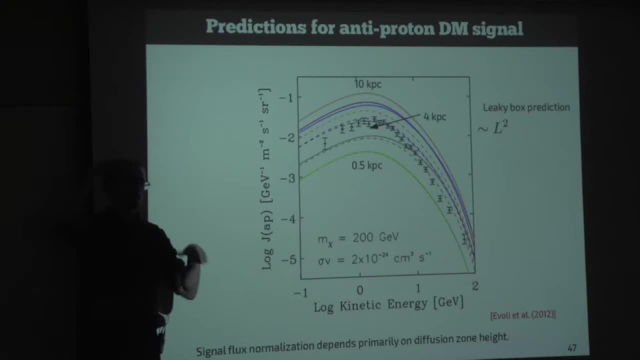 for the very reason that the diffusion zone height is not constrained. But dark matter is not just produced in the inner part of the disk, but it would be produced in the halo. So it would be produced anywhere within the disk, It would be produced anywhere within the diffusion zone. 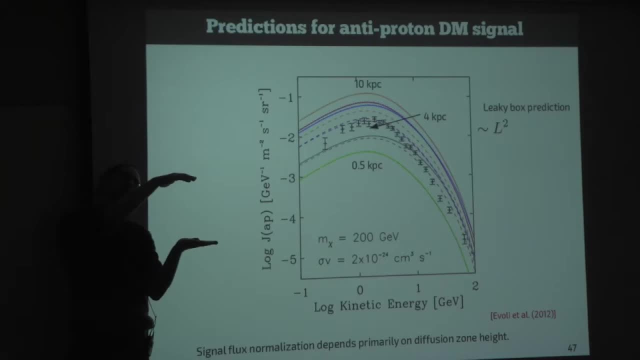 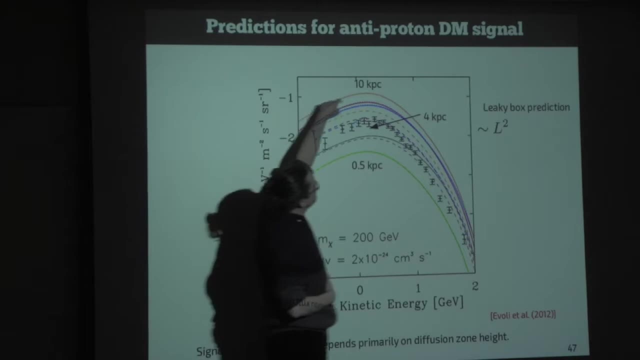 And somehow the region in which particles would produce is basically what diffuses the region where these dark matter annihilation products would be captured. So the larger the diffusion zone, the larger the expected flux And a long time it was not really clear. 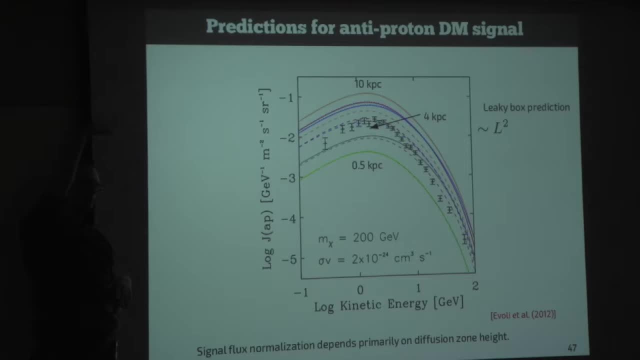 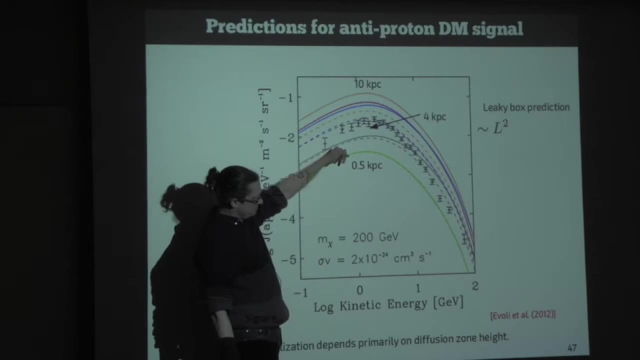 what are the limits on the diffusion zone? There are now more and more reasons to believe that it goes up quite high. But if you wanted to have a very thin diffusion zone- 0.5 kiloparsec- the flux would have been very low. 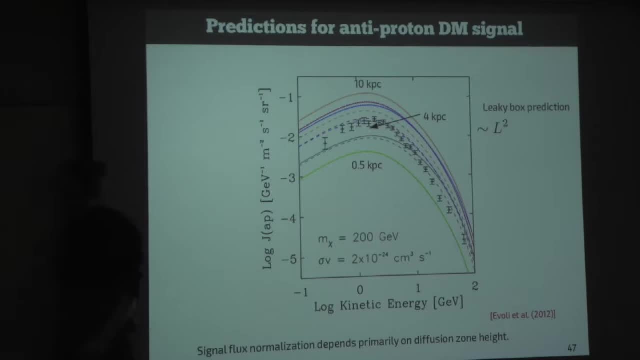 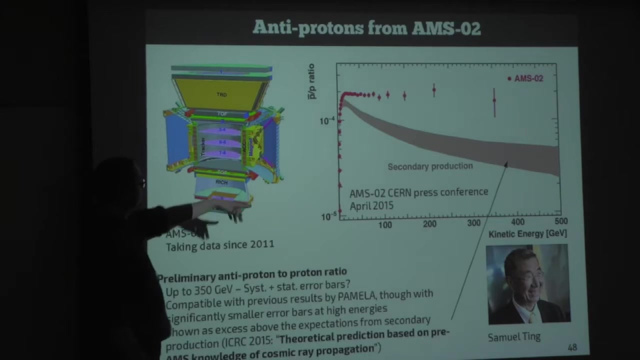 So that's just to illustrate that signal fluxes are much more sensitive to propagation details than actual background fluxes. So now AMS released their measurements in April 2015 of the antiproton to proton ratio And they had this impressive picture where they showed that they have a gigantic excess. 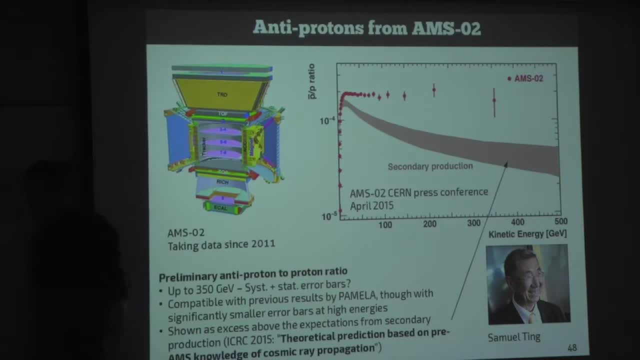 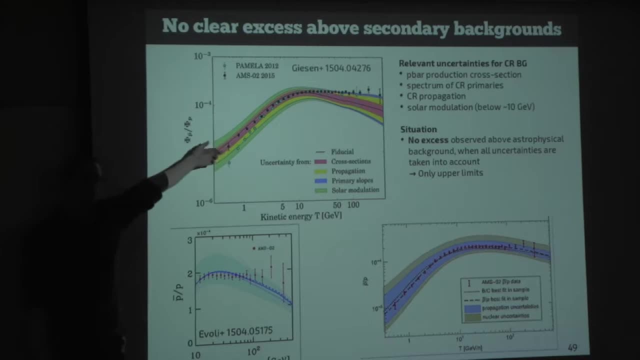 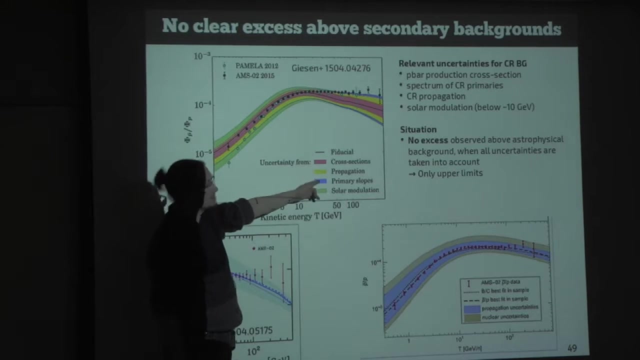 above the expected background. Fortunately, colleagues were very fast. They were correcting this to a certain extent. So this was a paper that was literally on the day on the next morning was in the archive. Well, they show, if you include various uncertainties. 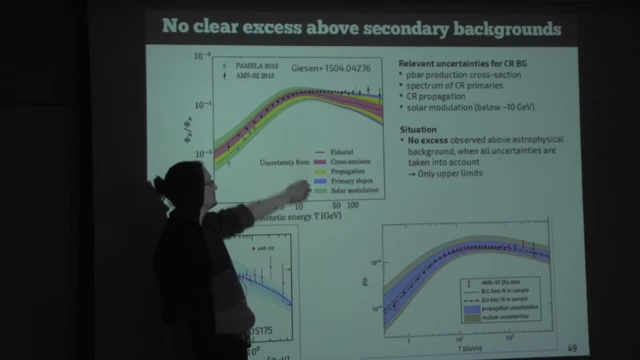 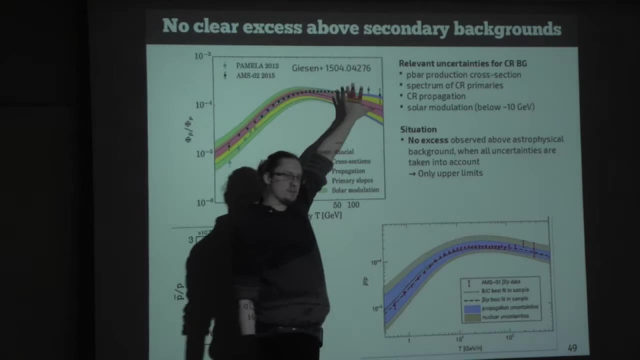 in the predictions for the backgrounds like cross-sectional uncertainties, propagation uncertainties, uncertainties in the primary slopes and solar modulation, which plays a role in low energies, then actually the excess is probably not that big in the first place. It's still obviously harder than what one would have expected naively. 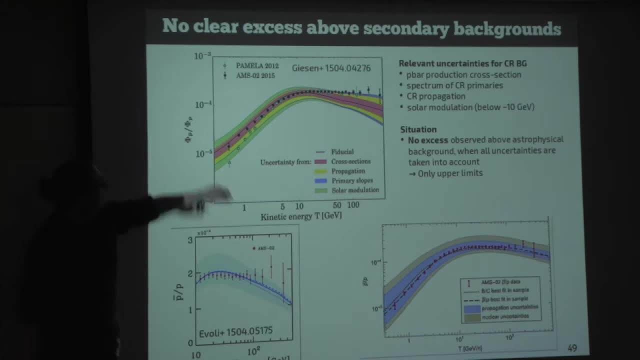 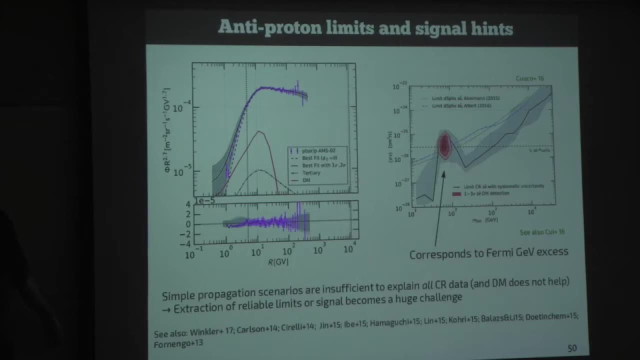 if one fits boron to carbon, But it's not clear whether you should call this necessarily an excess. I will come to that a bit later more, but I want to go fast through this. There were also some discussions that maybe there is nothing. 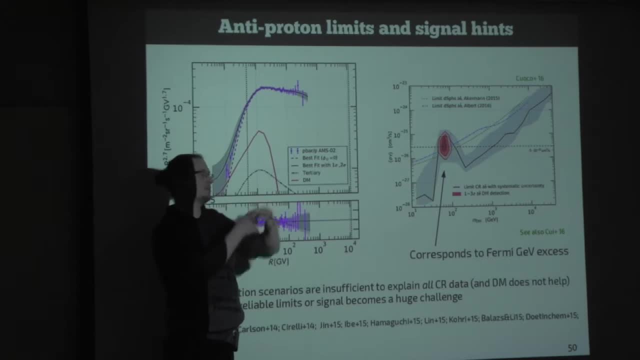 at high energies. There are quite some details about how to fit the data, So sometimes you can include boron to carbon. Other people don't include boron to carbon in their fits, and so on and so forth. So this group here only fitted. 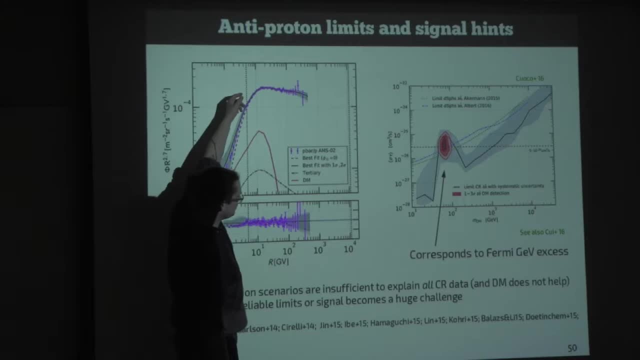 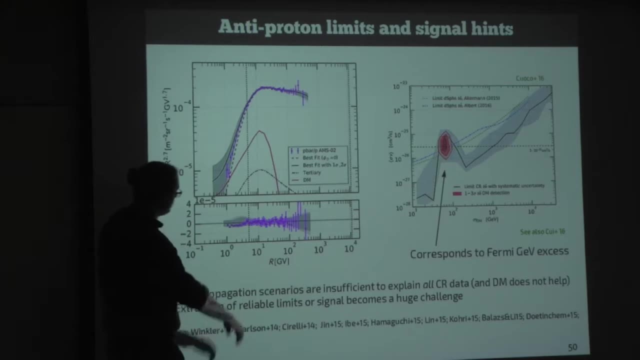 light particles and they found last year- I think this was also two years ago- that there might be an excess actually in this turnaround region. So like at one, at 10 GeV, it's hot, You wouldn't see it. 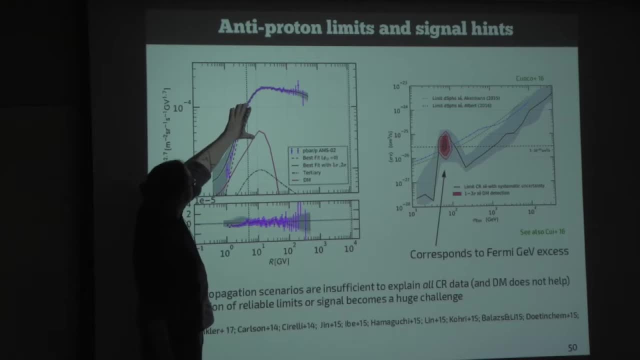 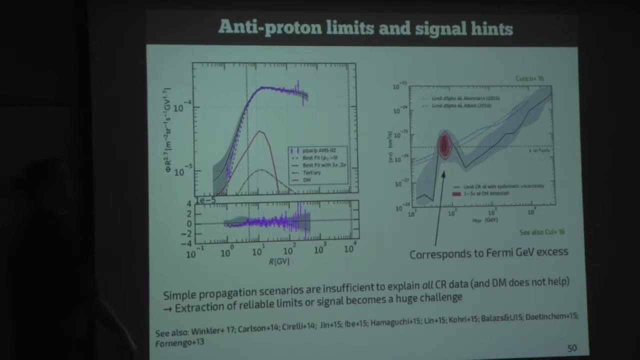 So it's like a couple of maybe 5% contribution to the fluxes that one sees here in this turnaround And this actually has stuck. So there are quite a few papers that found similar excess in the emission. I mean excess because it's really hard to identify. 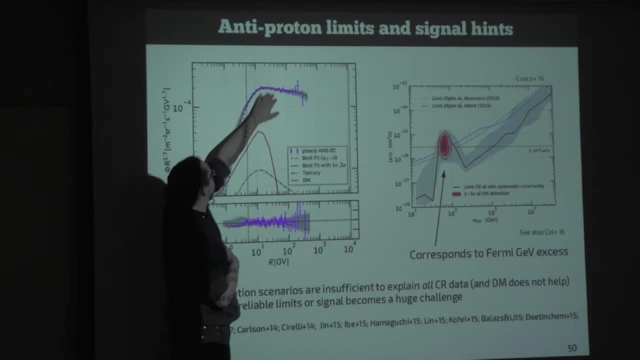 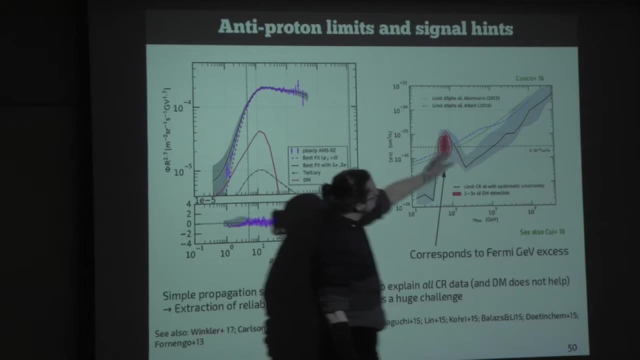 It's a very, very tiny residual that you see on top of a function that curves exactly where you see the excess. Nevertheless, the fun thing was that if one fits this, if one says okay, there is a dark matter, contribution, then actually the best fit values that one gets for this. 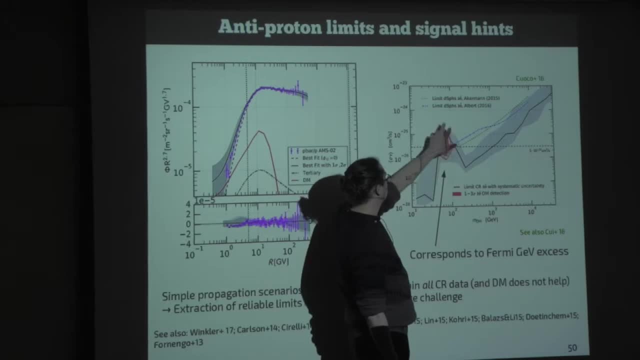 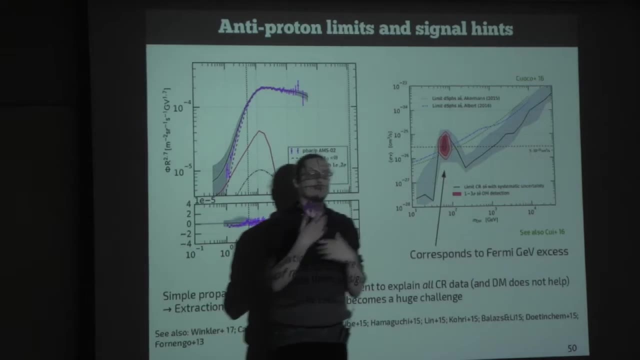 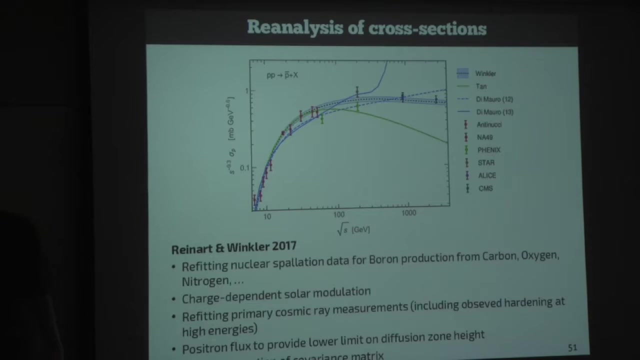 are around 80 GeV or something and annihilation cross-section consistent with thermal annihilation, which happens to be also pretty consistent with what you need to explain the firm GeV excess and gamma ray data. So this made it certainly interesting. Yeah, I could go into more details. 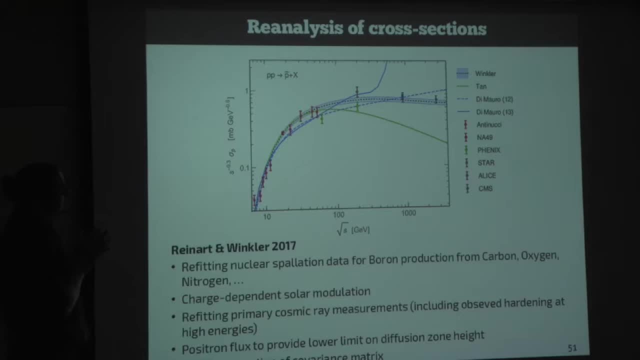 but one thing I want to say here is there have been various analysis afterwards. The nicest probably is from later last year. They basically analyzed the data again, but taking into account a large number of uncertainties by certain, uncertainties in the nuclear spallation data. 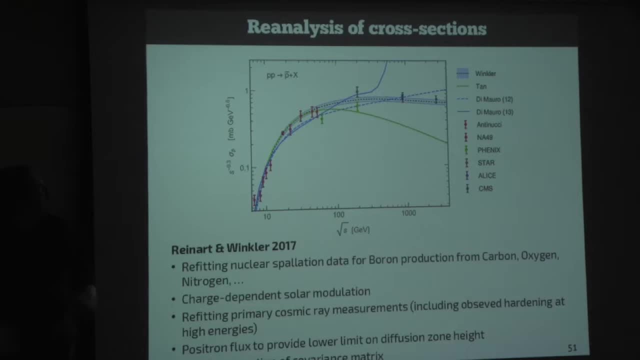 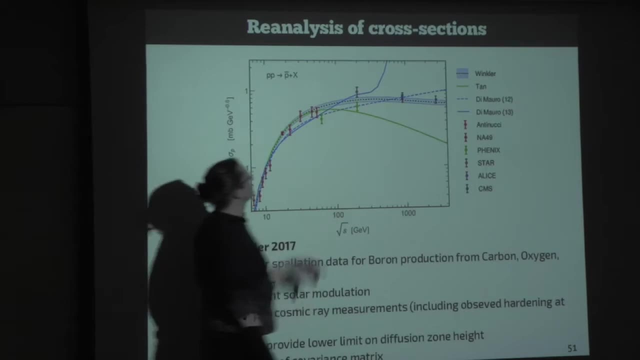 for boron production. So actually they refitted experimental data. this is here experimental data. This is their fit, You see, if various other curves that have been used, extrapolation curves in the literature, and they derived a covariance matrix for this. They derived a covariance matrix for solar modulation. 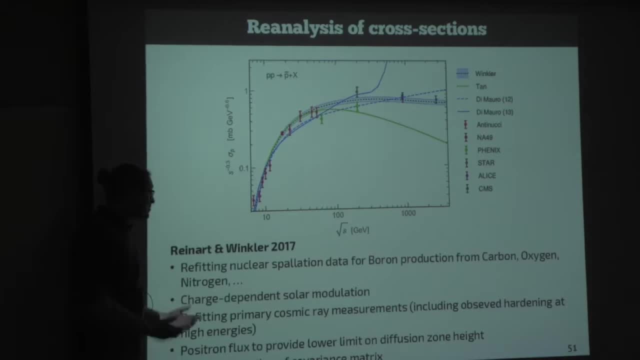 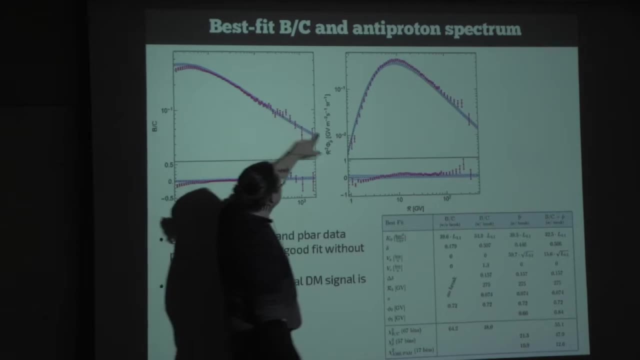 for the cosmic rays that are measured and so on and so forth, and refitted the data and found that then you can actually explain boron to carbon and proton to the anti-proton flux reasonably well with these two models, which look with this one model. 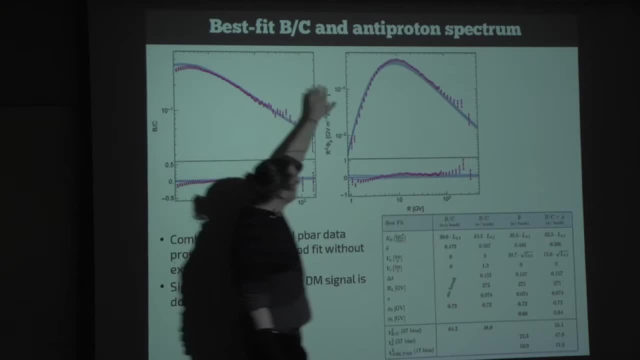 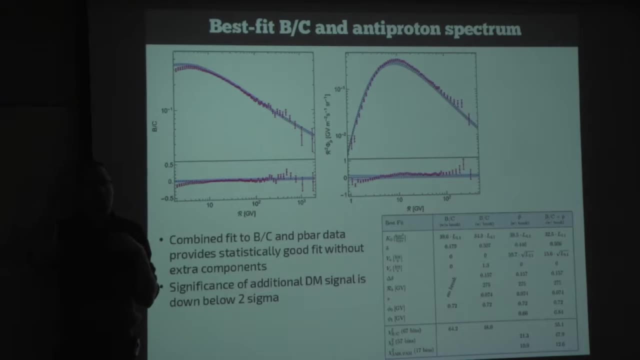 which doesn't look like it goes through all the data points very nicely, but it still gives a good fit to the data, for the simple reason that what these guys included is actually the covariance of the error. So this band here just shows the one sigma: uncertainty. 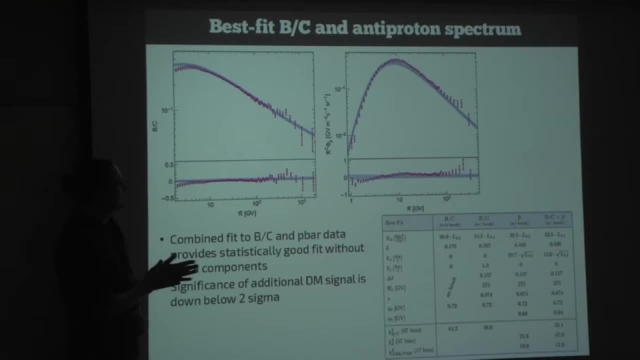 but the entire curve can move to accommodate the data and apparently it works. So apparently they have a reason model. But you see that there are correlated residuals and they found: yes, if you put a dark matter signal in in this range here, it improves the fit. 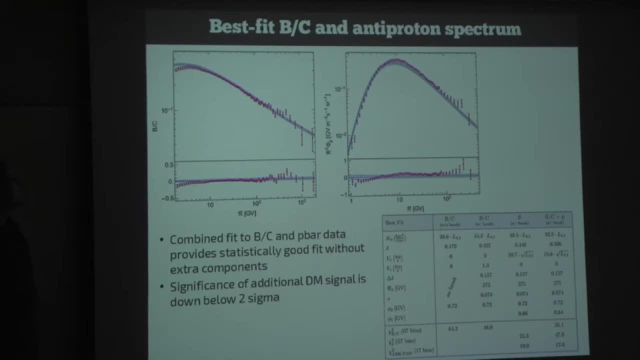 but only by one or two sigma. So taking into account correlated uncertainties is hard, obviously, but it's probably the thing one has to do in the future for any kind of cosmic ray analysis. On top of that one should also include correlated uncertainties. 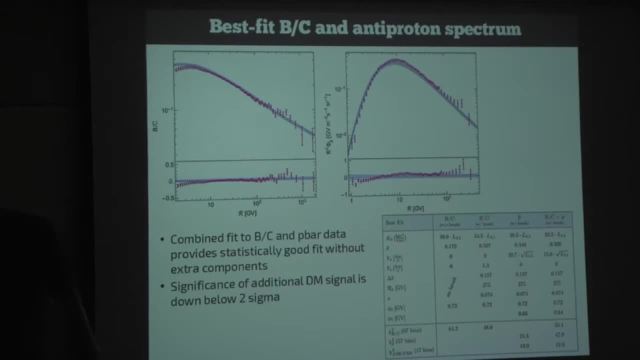 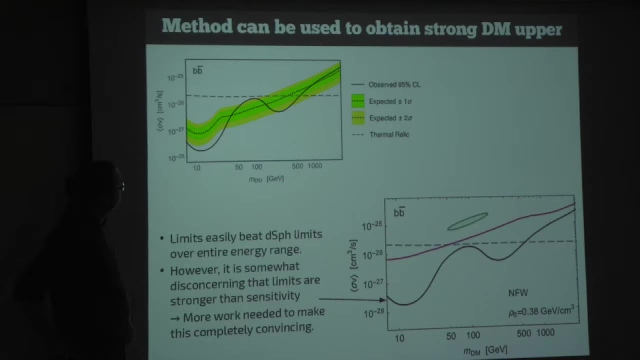 for the experimental uncertainties which nobody really knows. So that will remain a caveat. What's nice with this anti-proton story is, however, that one can in principle get limits that are stronger than the dwarf limits. So you do get this hint for a signal in this regime here. 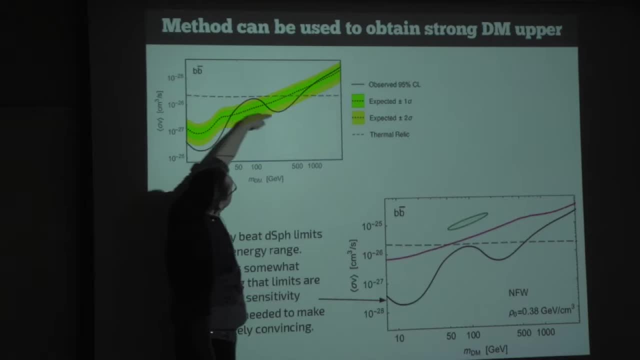 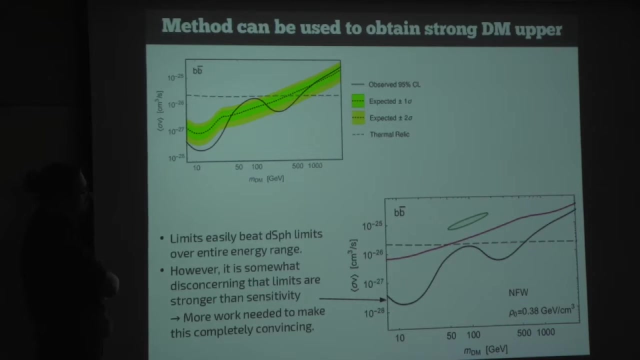 This is still from the Winkler paper, But you also get everywhere else pretty strong limits that happen to be stronger than the limits from Fermi dwarfs, as you can see here everywhere, And this is not something they only found, but basically every recent analysis found. 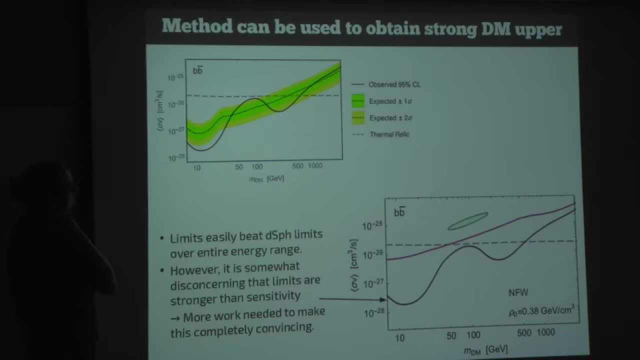 based on AMS data. What's still a bit disconcerting is that the limits seem to be sometimes much stronger than the expected limits, so that's a bit hard to make sense of, But I think if one wants to talk about getting limits stronger faster than probably doing it with anti-protons- 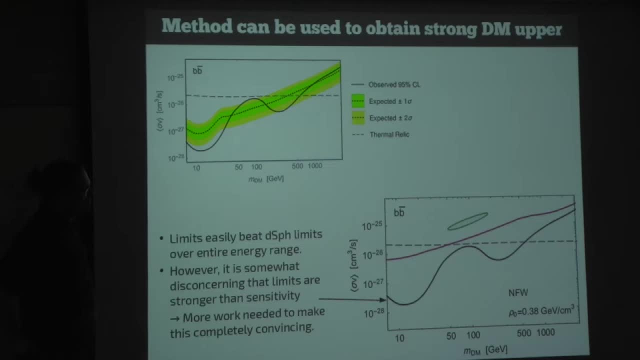 it's better than doing it, or easier than with dwarfs in the mid-term future, simply because the data is already there, It seems to be very strong. One just has to make a convincing analysis that keeps all the systematics in check. 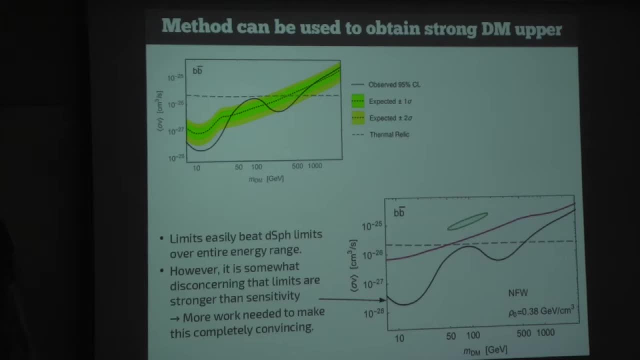 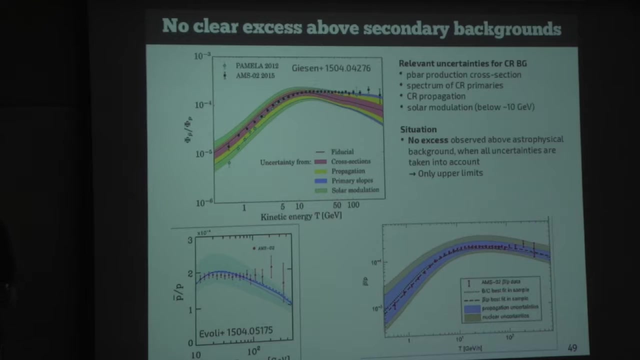 So that's anti-protons Questions Otherwise: Yep In number 39,. why data from and disagree at low energies? Can you repeat the question? Yes, I will. So a very good question is: why does data between different experiments disagree? 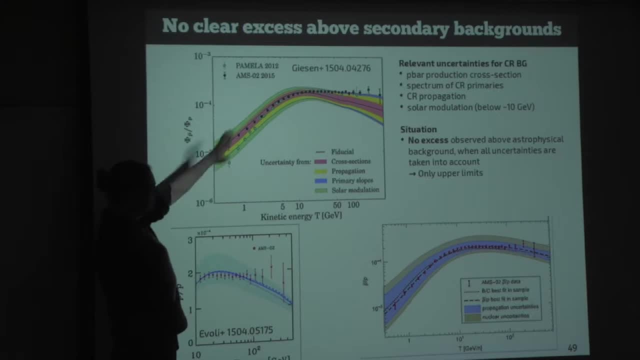 and nobody I mean. usually in talks like this this is completely glanced over, And the reason is it's a time-dependent effect. So this is solar modulation. So basically what happens is the sun has a solar wind. So basically these are charged particles. that are blown out in some complicated magnetic configuration, And the particles to cosmic rays have to reach Earth while going through the solar wind. So the less energy they already have from the start, the more relevant is this effect, And so this effect usually starts to matter, apparently. 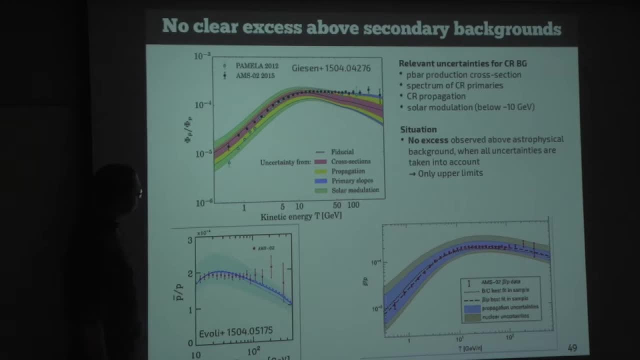 for energies around 10 GeV. I mean, this is what is observed in the data And it's a time-dependent effect, So it depends on the strength on this solar wind and also the sun has a cycle of 11 years or so. 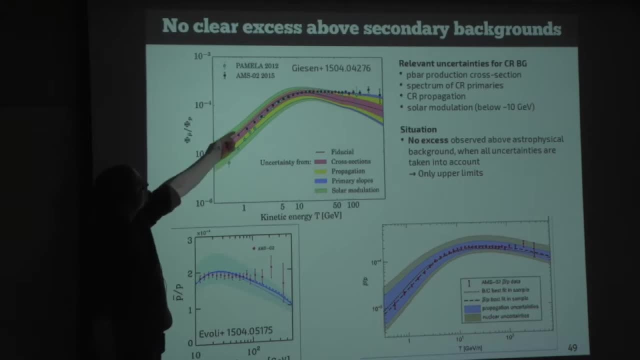 where it flips polarity, And to a certain degree it's also a charge-dependent effect. So there are differences, but there are also now quite a few nice papers where this is a bit analyzed in more detail And for instance, this charge-dependent effects are taken into account. 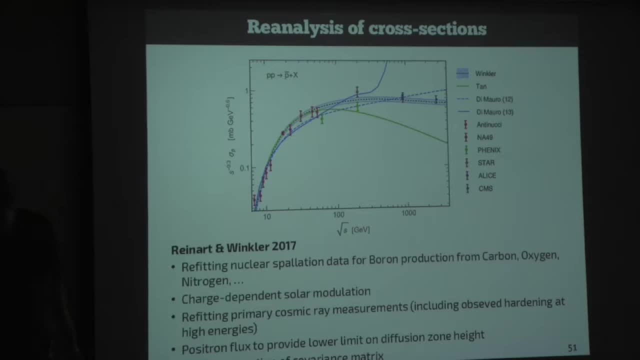 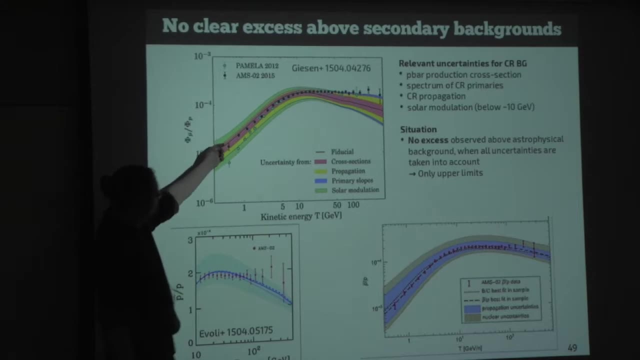 in this Winkler analysis. So that's the reason why there is a difference between different measurements, But usually there will be. for instance, if you would- I am not talking about this here- but if you look at the positron flux, that is measured. 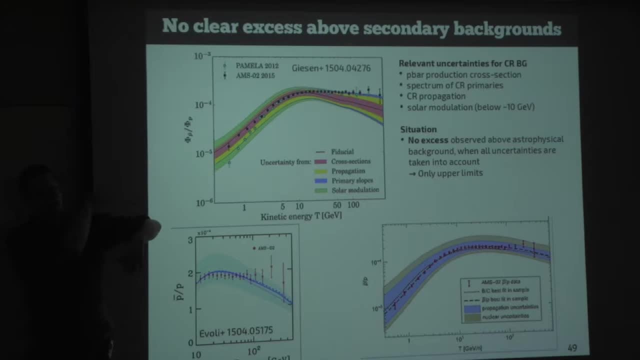 and compared to this with theoretical predictions also, usually there is a- I mean this is different- at high energies and at low energies. At low energies because of solar modulation and at high energies because of probably additional primary sources or additional primary sources most likely. 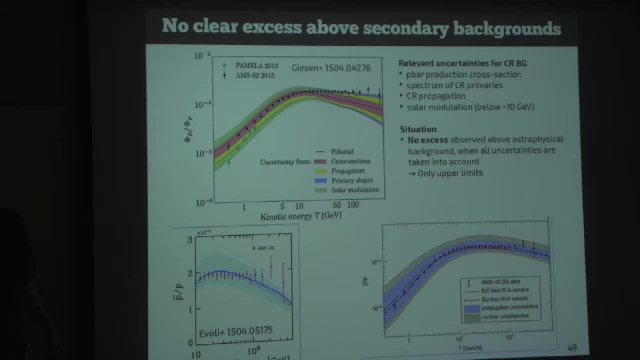 Does that mean that PAMELA and AMS2 or if they were in different? I don't know anything about these. This is mostly because of different measurement times. So the AMS data was taken, I mean until recently, but I think that these data 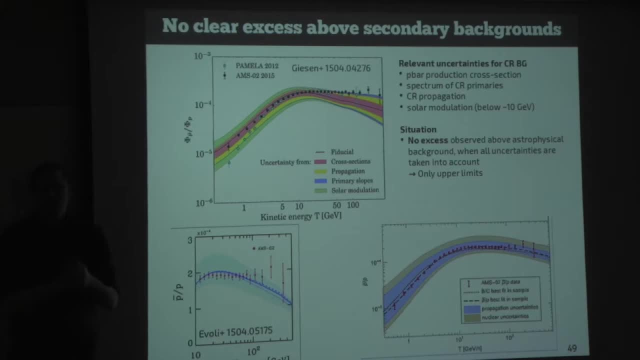 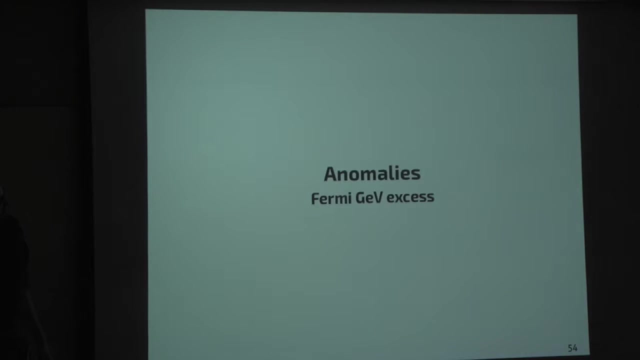 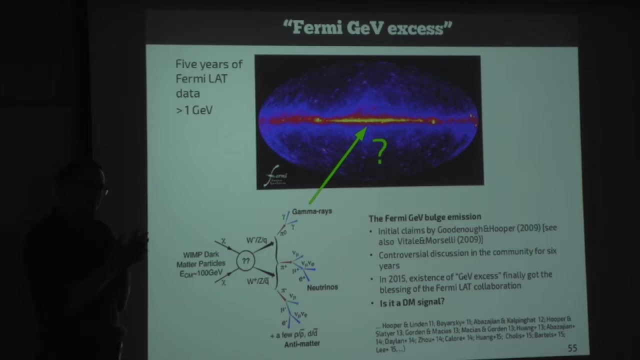 points are probably between 2014 and 2016 or something, And so PAMELA data was before And so this is affected differently. More questions, Otherwise, I will go on with the Fermi-GeV access. So who has not heard about the Fermi-GeV access? 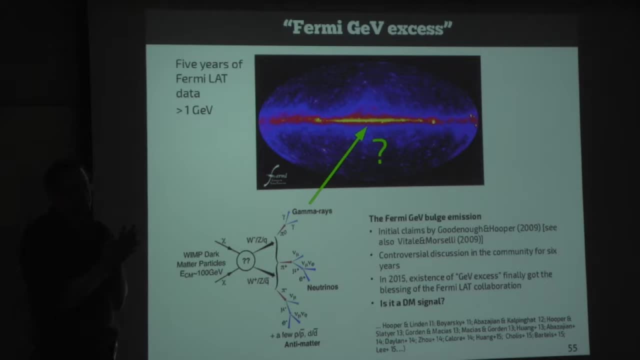 It's not embarrassing. It's not embarrassing, It's supposed to be embarrassing. I guess everybody has heard about it because it I think it is. Yeah, yeah, But probably we all I would Different things. Yes, yeah. 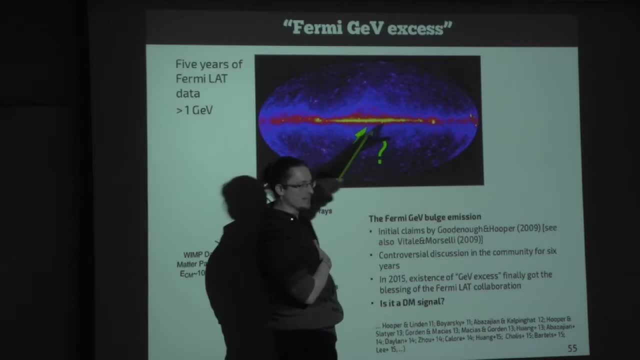 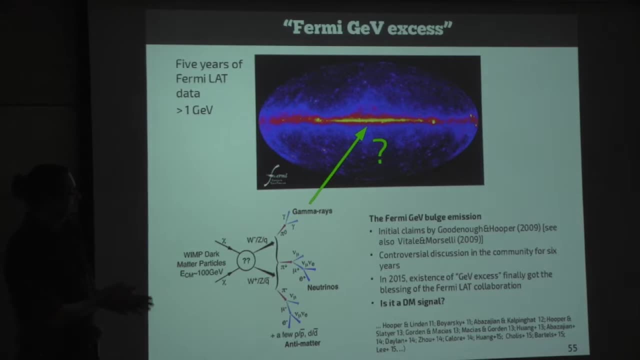 So the basic idea is: if you take Fermi data, look at the galactic center, make something complicated, you find an access that peaks around 2 GeV or something that happens to look like a dark matter signal, So that's pretty cool. 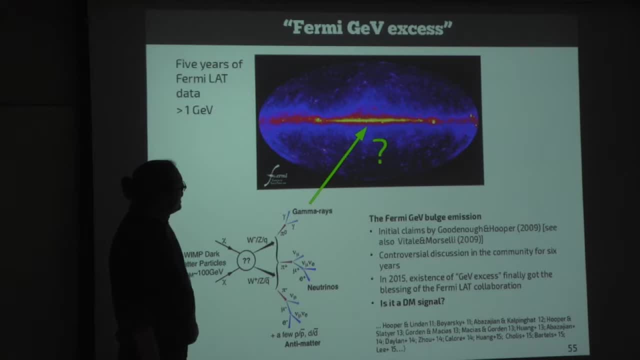 because of course, we would like to find dark matter signals And it's probably from my perspective, since I'm working on this stuff the most. I mean, if you want to have something that looks like a dark matter signal. 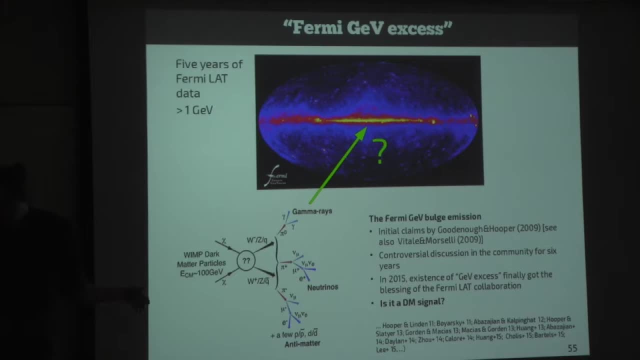 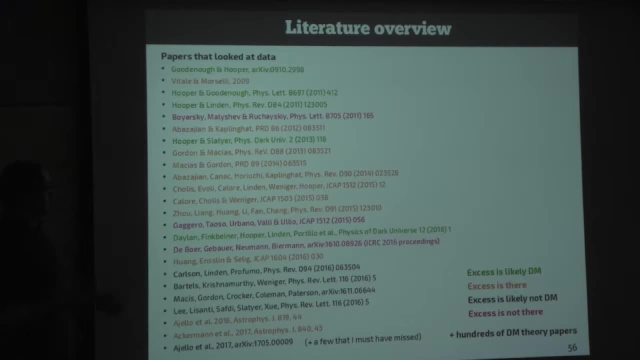 or if you want a dark matter signal that's like the vanilla thing you are looking for, that doesn't mean it's a dark matter signal And I have. I will explain this a bit more, But it could have been And it would have been a nice one. 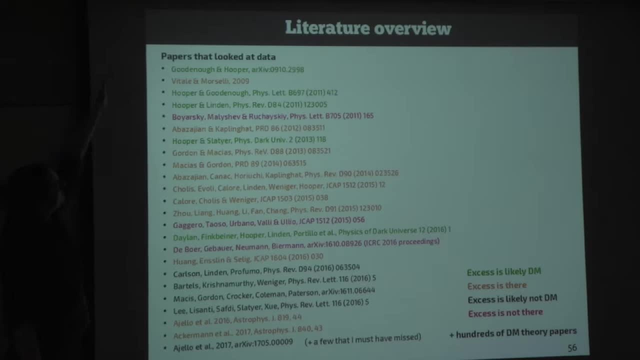 Anyway, And we still don't know. So this is a literature overview, Just the papers that looked at data. There are like hundreds of papers that built models for this. You see, the green ones are all about, like it's dark matter most likely. 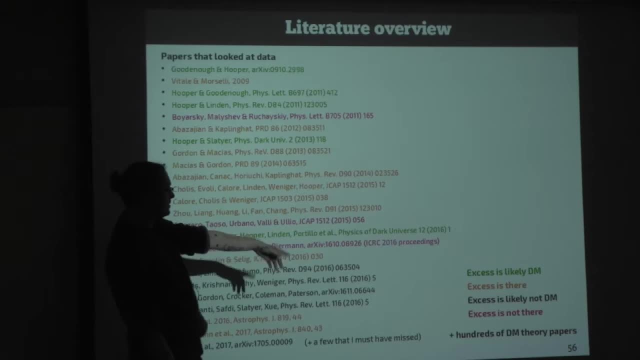 Then excess is there. It's the yellow ones. The black ones are, It's probably not there, And the red one No. The excess is likely not dark matter. The black ones and the red ones are Okay. Actually, it's not there in the first place. 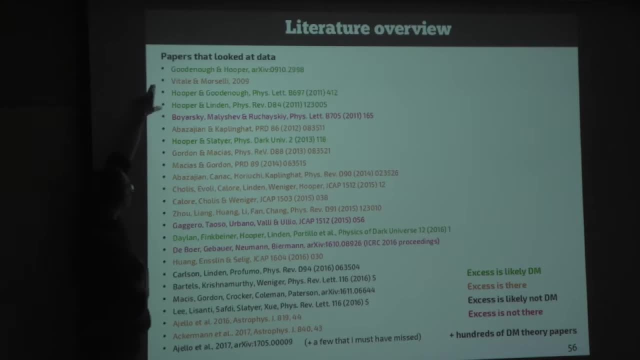 So what are you talking about? And you see, the green ones are all with Dan Hooper. He was a huge advocate, But I The point is, I think the entire story wouldn't have started without him. So it looks like this excess is there. 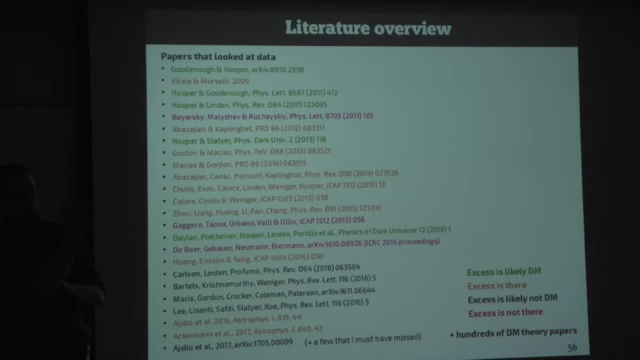 It's an interesting thing to understand what's going on, And he He's the guy who pointed to it, So All the credit to him. But yeah, we simply have to figure out what's going on there, And it looks pretty cool. 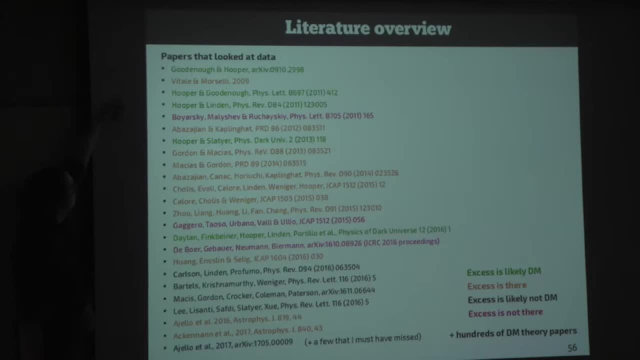 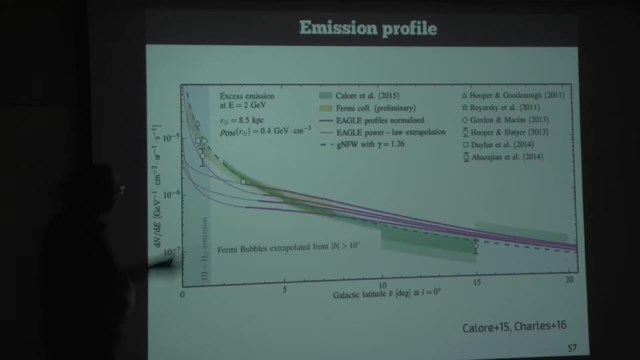 So Good. There were many papers. I will mostly talk about my own. But Okay, Emission profile: This is what people tend to agree on to a certain extent. So there's, If you measure the excess emission. So I should say: 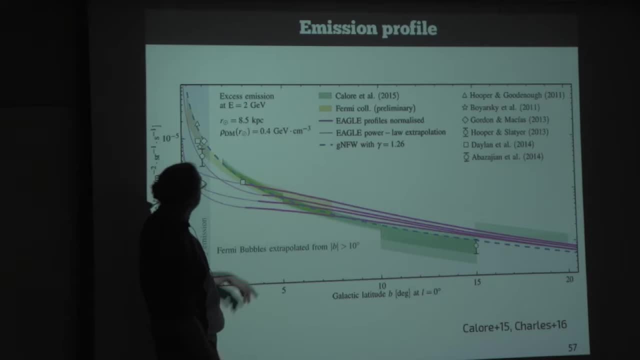 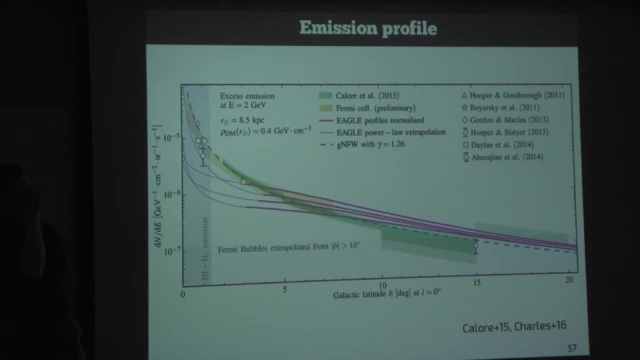 what's the spectrum? So the spectrum is compatible to a certain extent with dark matter annulation, with mass emission. So there's, If you measure the excess emission, So I should say it's around 50,, 60,, 70 GeV. 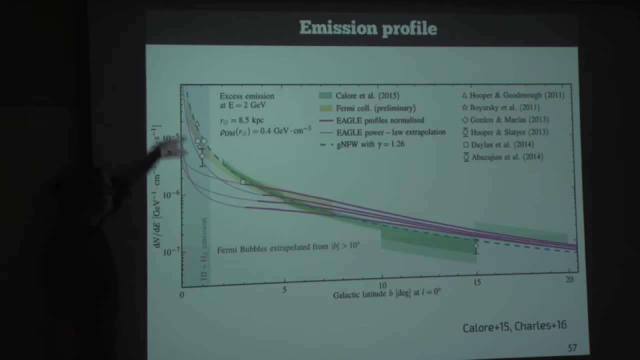 or something into BB bar And it has a profile that seems to be a bit steeper than what you get from So And a bit steeper than just the NFW. So this year's comparison with actually simulations, So antibody simulation results: 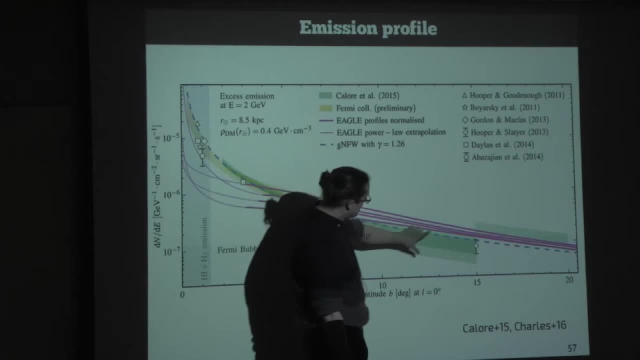 And the profile was measured by various groups. We made this These regions here, the green ones, Other groups around Tracy, Slatyr and also Dan found similar error bars. So this excess emission seems to be something that peaks towards the center and then goes up. 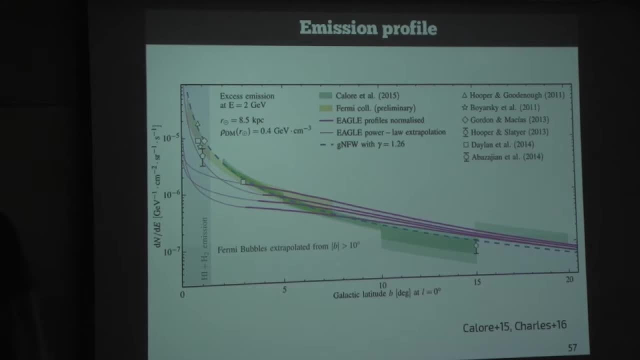 to 10 degrees, probably even higher, Although it becomes increasingly hard and more just like mixed with the Fermi bubbles at very high latitudes. But the sweet spot where you can say something about the excess is basically a couple degrees away from the galactic. 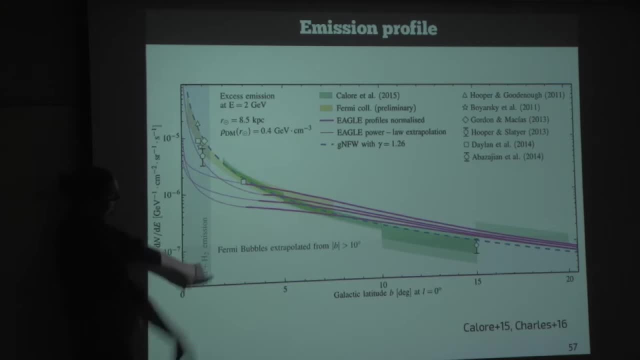 disc or center, because there the gas emission does play less role, in the Fermi bubbles at least if you assume they are flat. So I should say the Fermi bubbles have huge extended bubble-like features around below and above the galactic plane which are very hard. 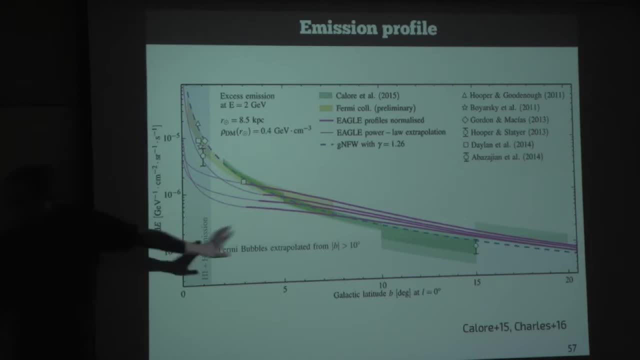 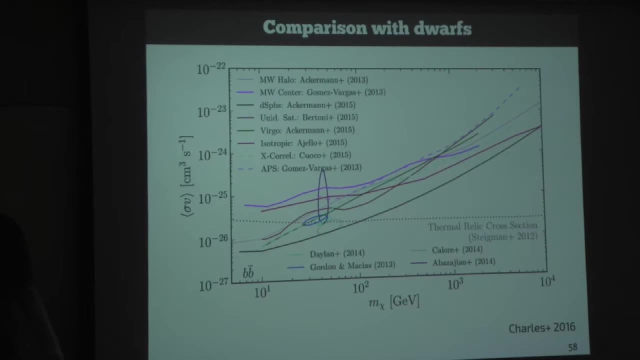 to model. So they are always a concern in this game. But one can hope that they maybe don't play a major role in this inner part here and don't affect much the excess discussion. Okay, So these are best fit values for the Fermi-GEV excess. 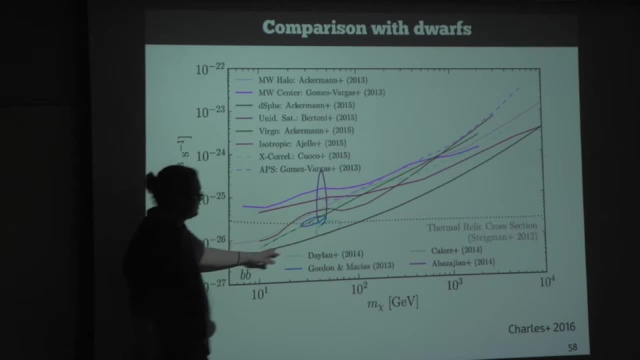 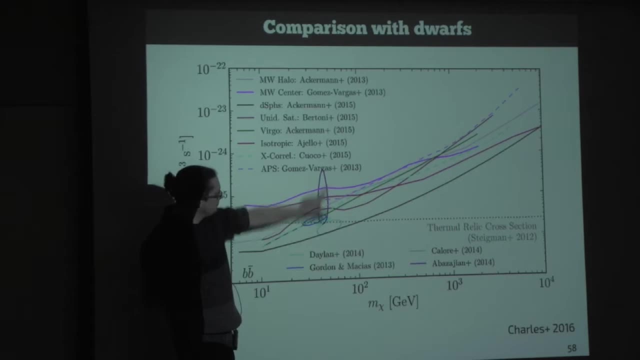 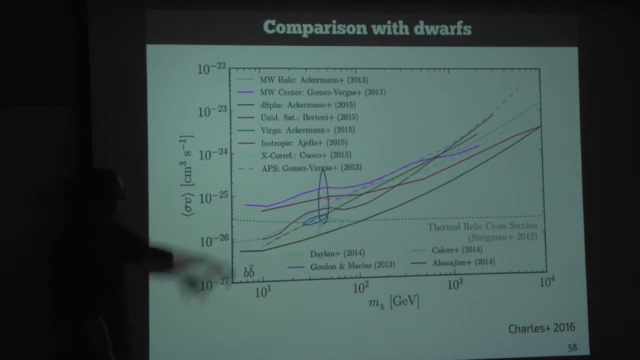 And the black curve is the dwarf upper limits, which seems to exclude most of these measurements, But they are still. for the galactic center excess there's probably a wiggle room of a factor of five or four or whatever, So maybe we underestimate the dark matter density. 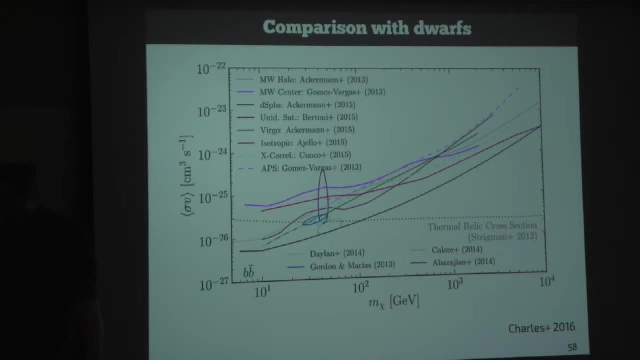 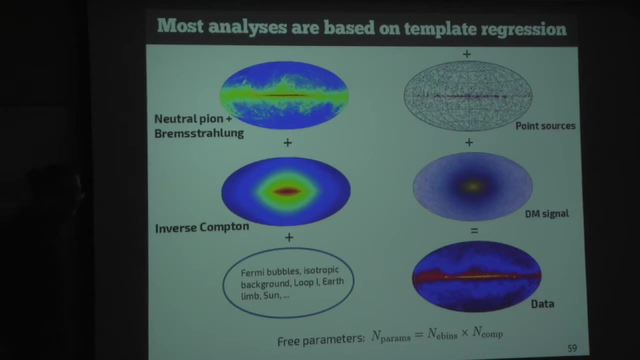 there. So this would move down and the dwarf limits also have some uncertainty. So this is not a killer argument, But it certainly would have been nice if it were a dark matter signal, if it would have shown up in the dwarfs. So what I want 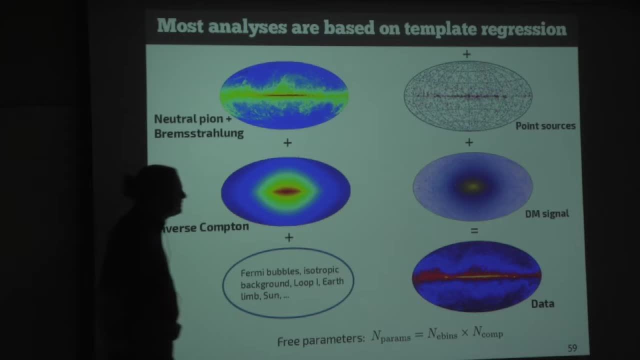 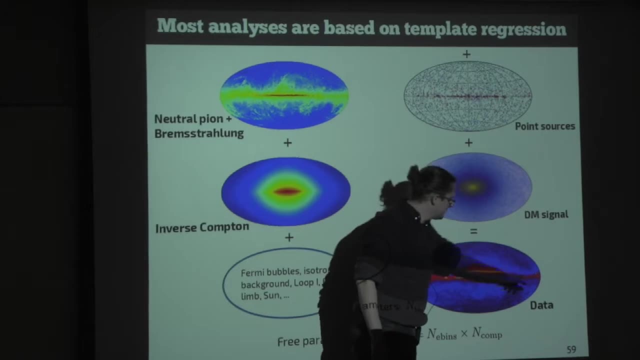 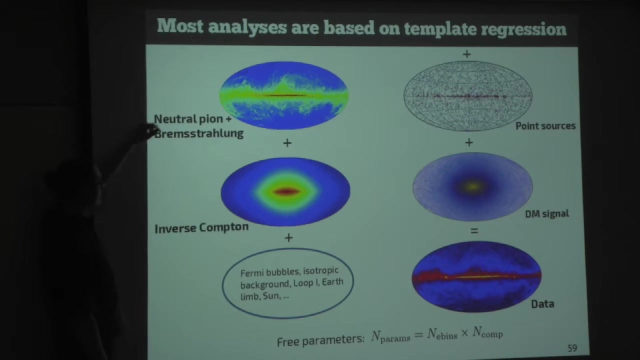 to talk about a bit is how these analysis techniques actually work. So I'm going to start with the galactic center and the rest, And then you try to model it with the various components that play a role. One is inverse emission. I already 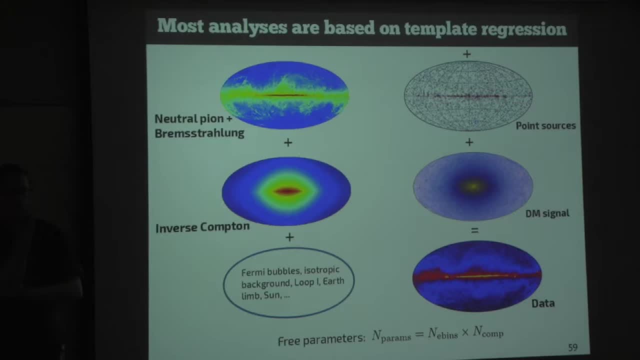 mentioned this. So this is produced by cosmic ray electrons scattering on starlight or the CMB, or dust emission, thermal dust emission, And this is basically tracing the interstellar radiation field to a certain extent and the distribution of cosmic ray electrons. So it looks. 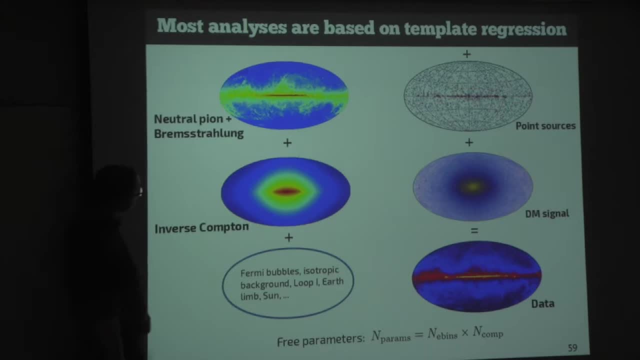 pretty smooth. Then there is cosmic ray interaction, So mostly proton-proton and proton-helium and proton-neutral interactions. So this would be neutral and this produces neutral pions which give rise to the interstellar medium And this traces the interstellar 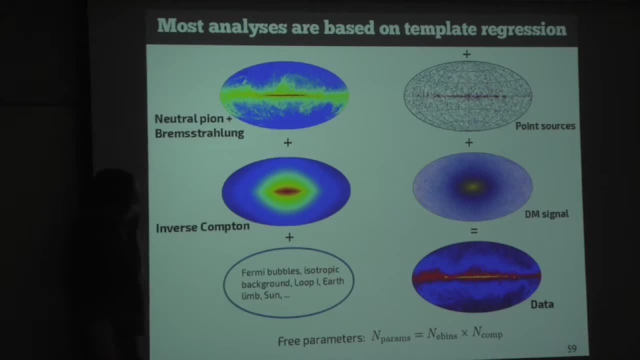 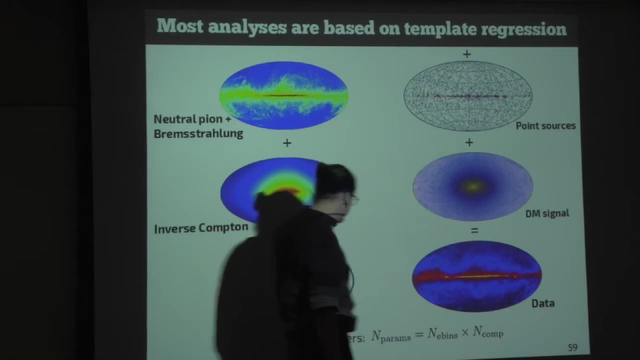 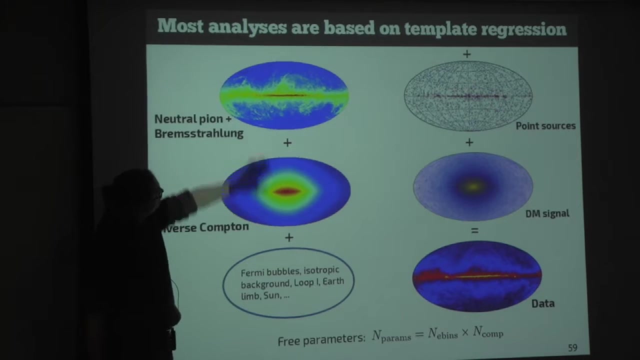 medium. So this would be this cloud-like structure. Basically, what you see here is the distribution of gas, And on top of that there are a couple of thousand point sources and maybe some dark metal signal, and then you try to fit it to the data. 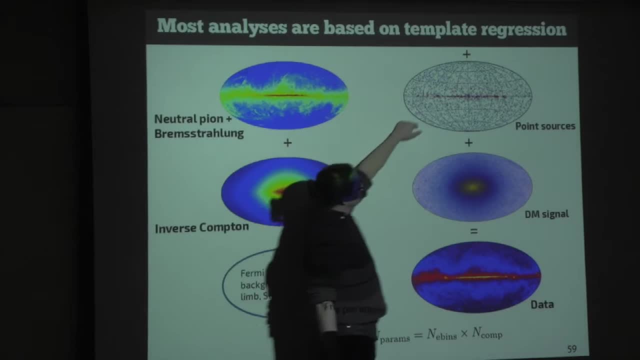 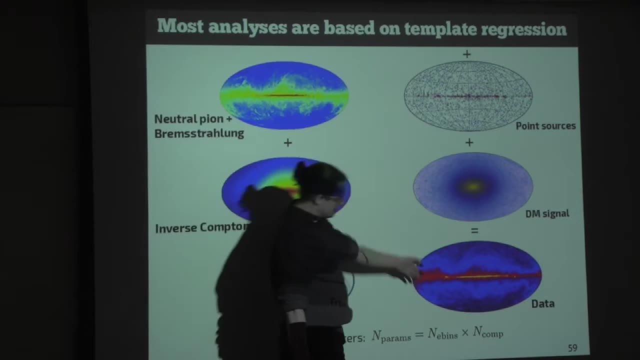 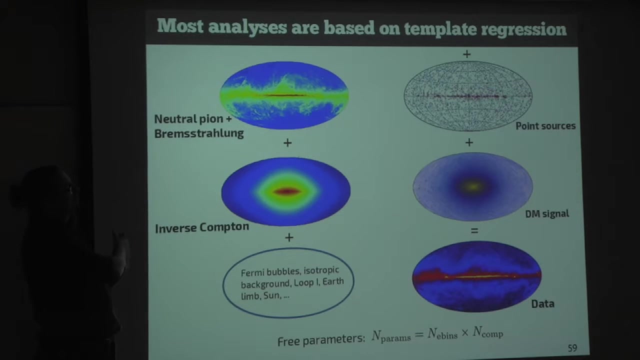 And usually the numbers come in and then lots of point sources. ideally you just mask them plus some dark metal thing And then you fit it to the data and so this. but you do it energy bin by energy bin, So you can split up the entire. 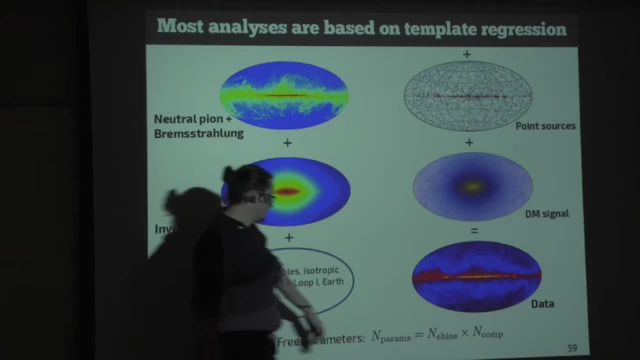 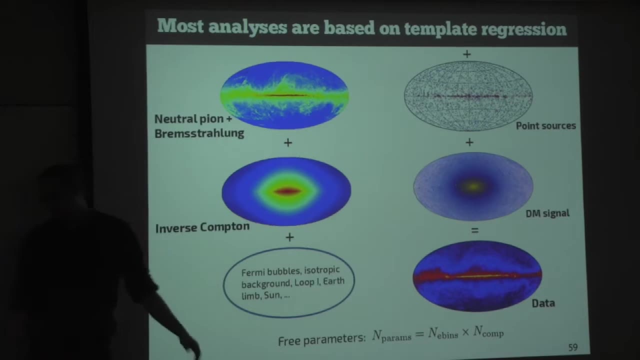 problem in like 30, whatever energy bins between. this is basically the number of energy bins that you have and the number of components. So this is called template fitting So for the mutual pylon. and have they based on data or simulation? No, So the 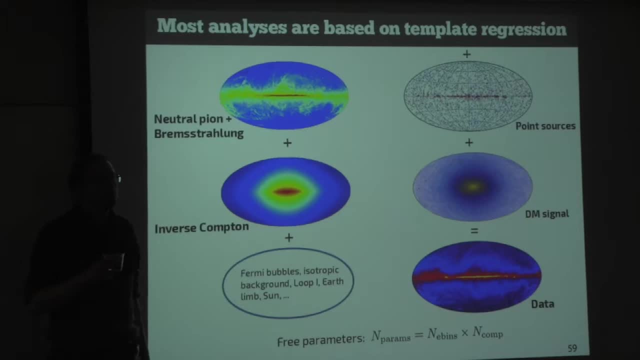 question was: where does anyone do it? where they forward model the gamma ray spectrum, so they, In a certain extent- this is like whatever version of okay. the question was- and I will come to this in a second as well- whether people do forward modeling in the sense of 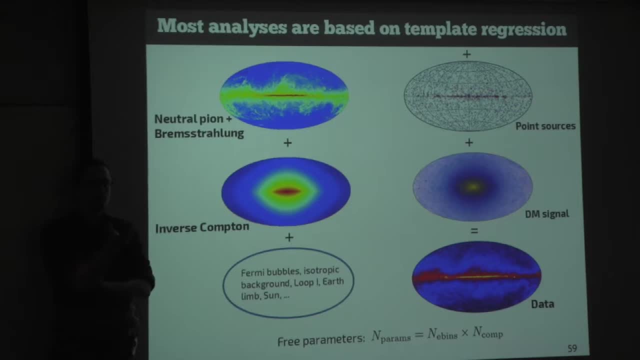 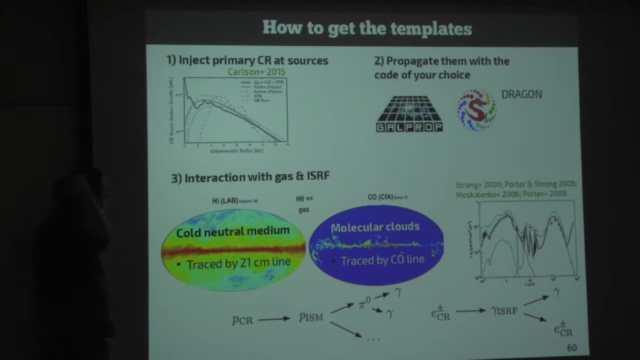 instead of just starting with templates and whatever I guess and then fit this to the data. this is what should be probably done, but nobody has done it in this complete way because it's like a crazy amount of work. So usually actually one does this in multiple. 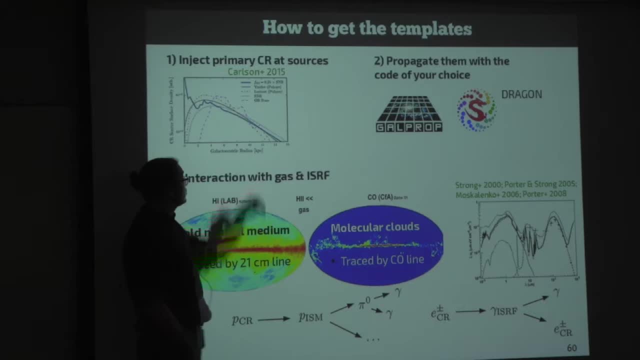 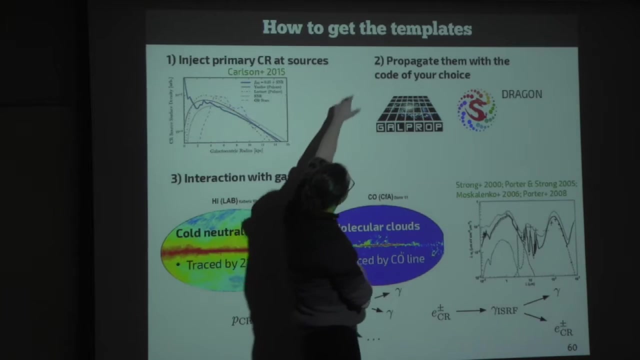 steps up to now. So if you want to do this, you can do this in multiple steps, and you can do this in multiple steps, and you can do this in multiple steps, and so there's just nothing really happening in the inner galaxy in this analysis. 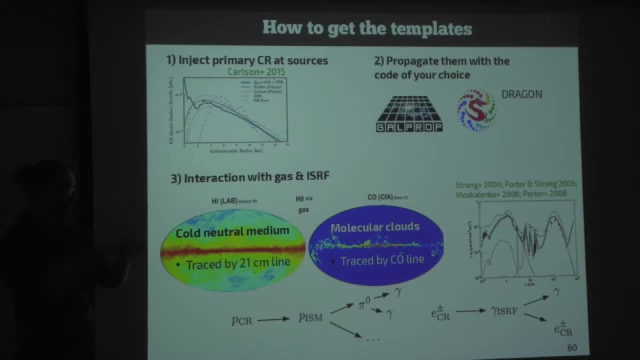 And then you propagate the cosmic rays with propagation codes that calculates their interaction with the interstellar medium and energy losses for the various spatial morphologies, which you can then put back here into this model. There are lots of caveats to that, but I will come to. 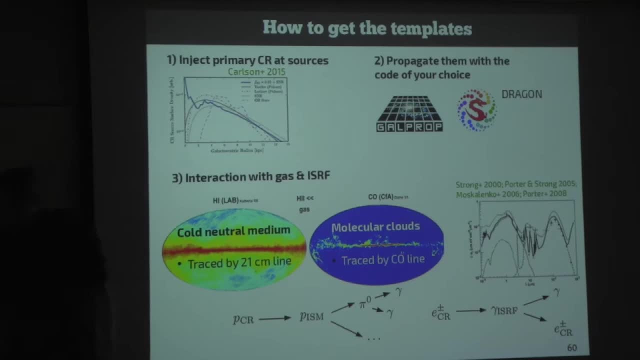 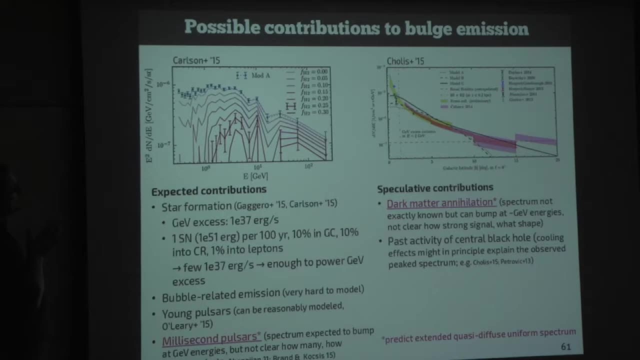 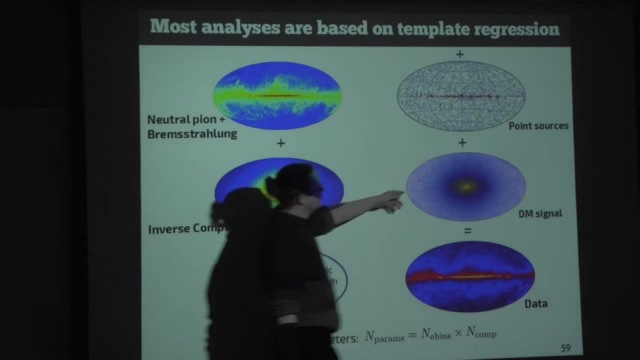 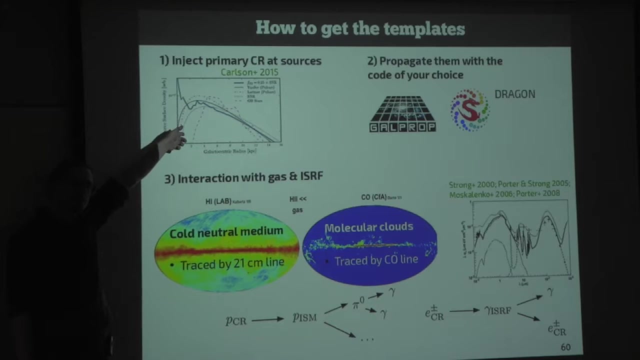 this in a second. So what you need for this is obviously the gas maps, and you also need a model for the galactic center emission. So what you need is this extra component in the inner galaxy. but, as I said, usually actually this extra component is 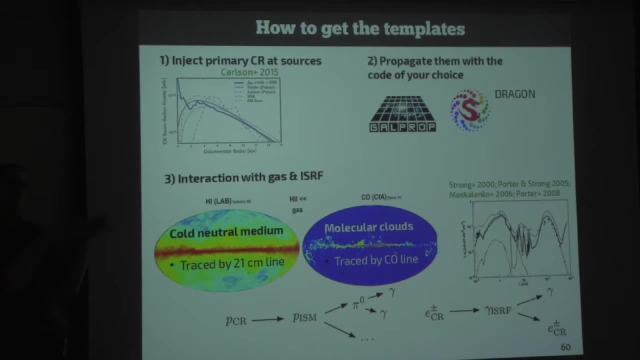 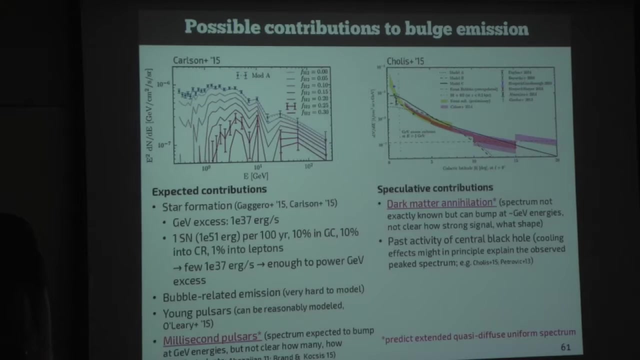 identified above. models that inject don't have all these analysis- not all- but what many of the analysis do is subtract foreground. so you subtract the galactic disk, you subtract anything along the line of sight, but many of the analysis didn't have the galactic center. so 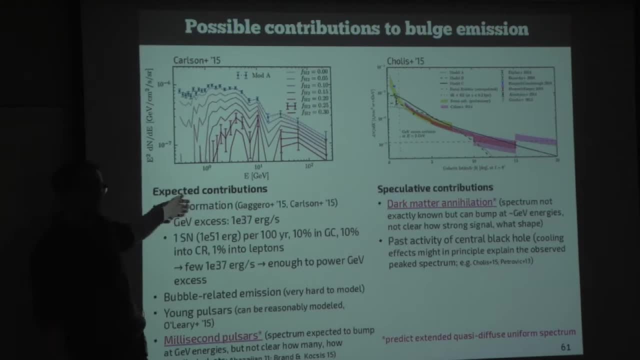 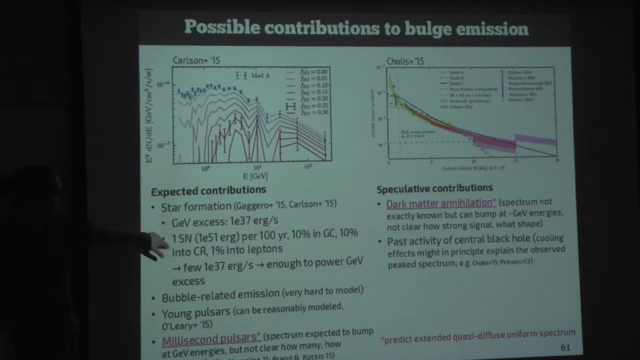 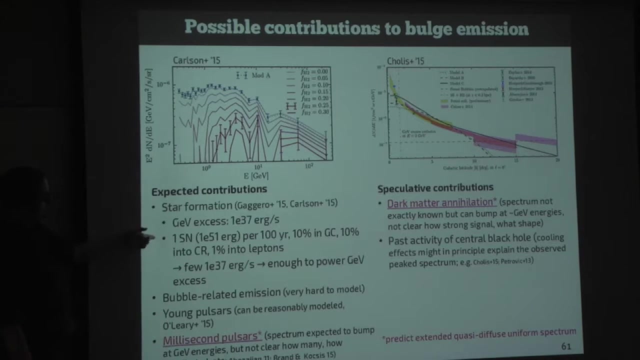 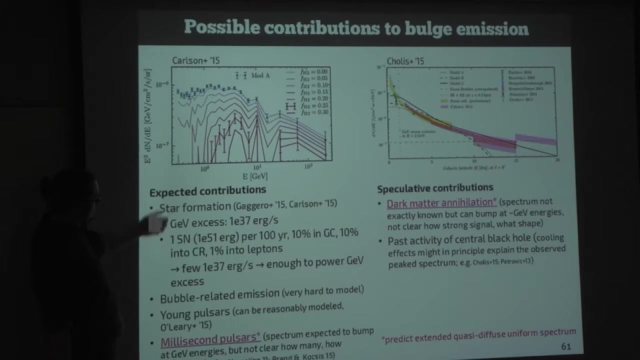 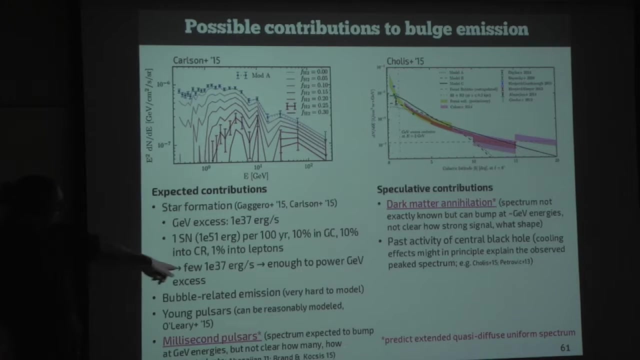 you can actually see some of the galactic center, which is the center of the galactic center. so you can see the galactic center and the galactic center is the galactic center of the galactic center. so you get the galactic center if you. 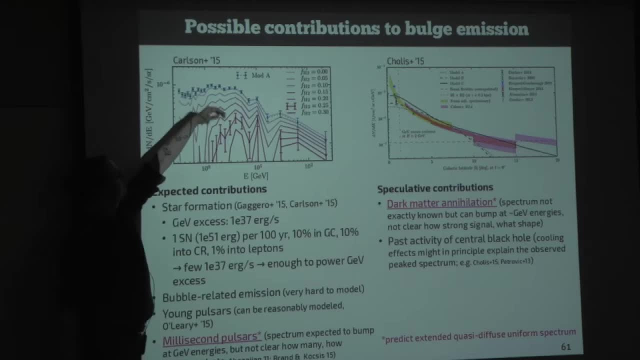 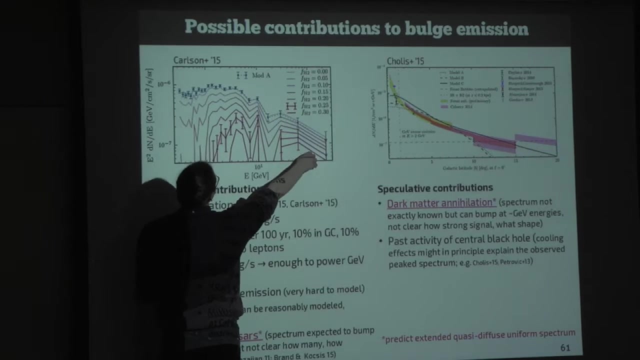 want to draw in a galactic center, so you can. problem is I should have put a spectrum for the. the GVX has a spectrum like this something and star and inverse common usually just looks much softer at low energy. So if you try to explain the GVXS here, 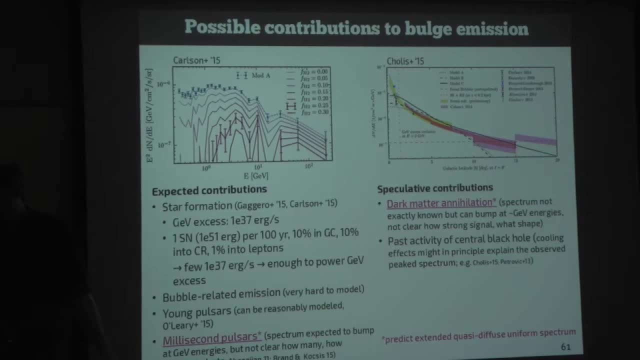 you over-subtract here And that's a universal property of everything I've seen that people did with star formation up to now. There might be ways around, but it's not easy, So you usually get the spectrum wrong. Then there might be bubble-related emissions. so 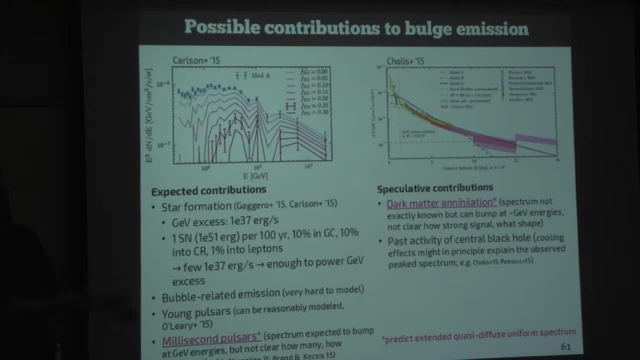 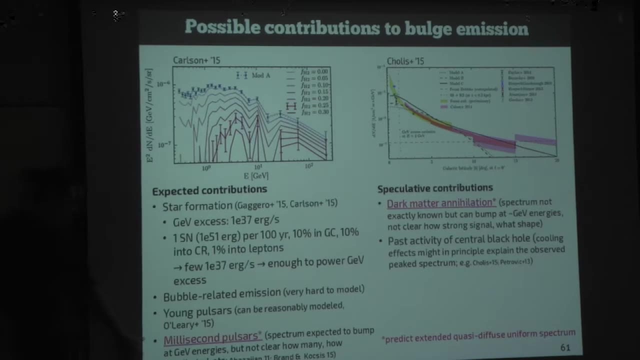 emission to these Fermi bubbles, but who knows? Then again, the question would be: how does it produce something like the GVXS? There might be young piles that could contribute, or millisecond piles, and we'll come to this in a second. 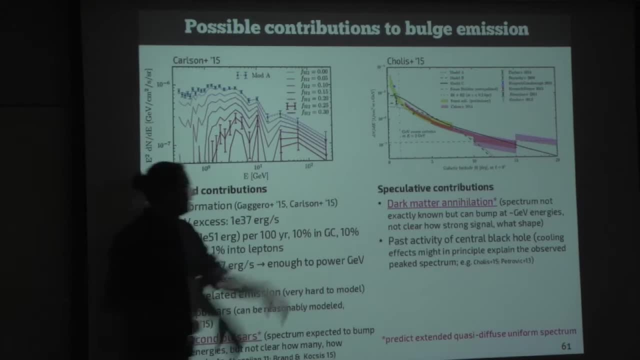 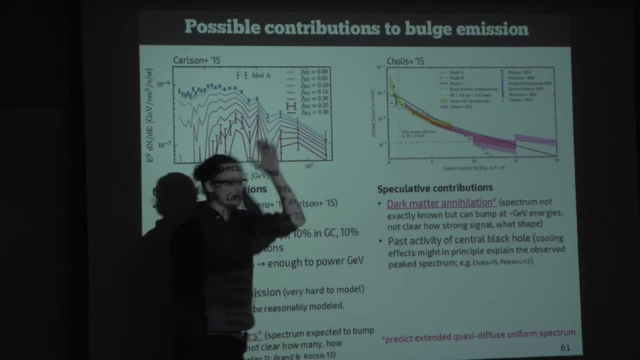 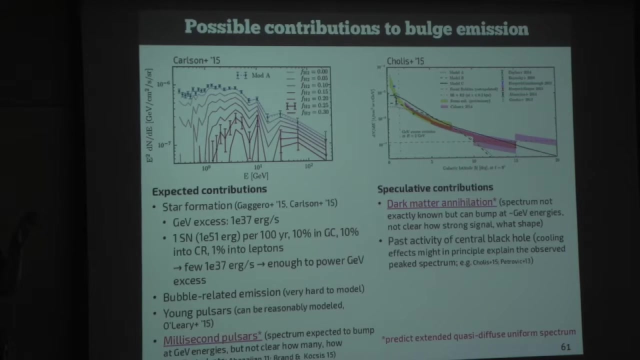 And then, on the speculative side, dark matter, obviously, which seems to work very well. So dark matter, as I said, explains the excess. What's remarkable with the excess? and I deleted these slides- but what's interesting is, if one looks, 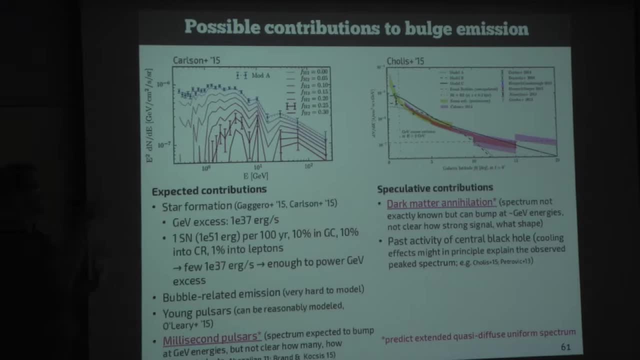 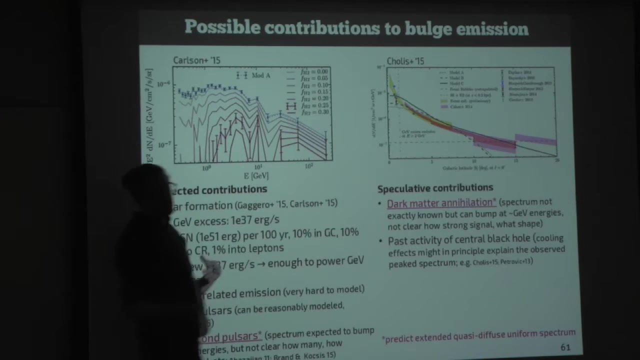 at different regions around the center region of the galaxy. the spectrum of this excess emission seems to be very similar. So you get a peak at a couple of GEV. So this suggests this is compatible with dark matter annulation, because you would expect to see the same. spectrum everywhere. It's also compatible with a large number of unresolved sources that on average look the same in different regions of the sky. It's not so much compatible with inverse quantum emission, because energy losses actually would produce different spectra at different distances from the galactic center. 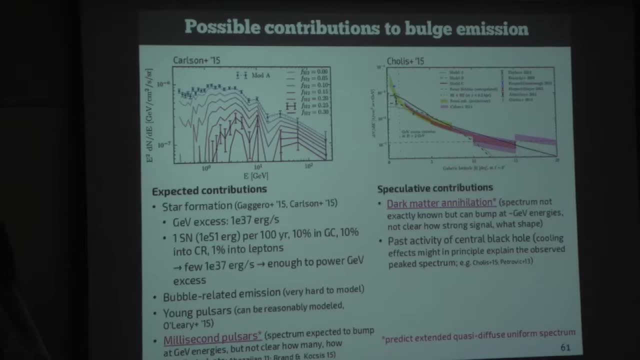 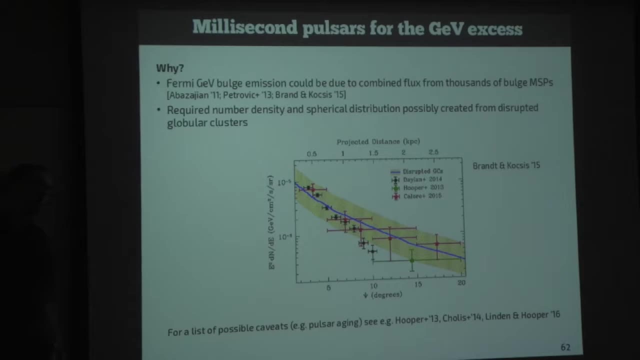 So this is why I find inverse Compton-related explanations not very compelling, although inverse Compton emission related to star formation should play a role, but probably not the role of expanding the GEV excess. So, millisecond piles, why are they interesting? 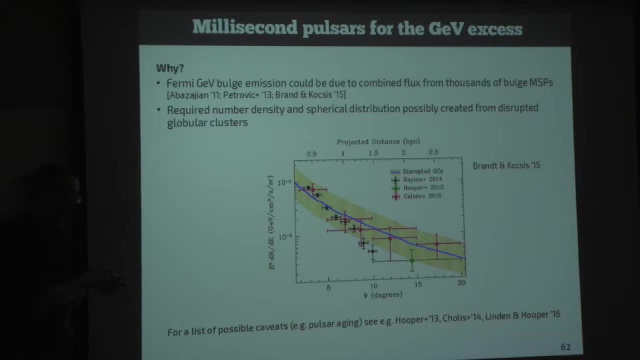 First, to expand the GEV excess with millisecond piles, one needs a couple of thousand of them At least. how do they get the bulge? Well, there's one idea which is okay: how do you produce millisecond? piles. First you need a pulsar, a binary system that then starts creating material from the companion star to spin up, and then you get a millisecond pulsar in the best case. So you need dense enough stellar systems to have enough binary systems to make this happen. 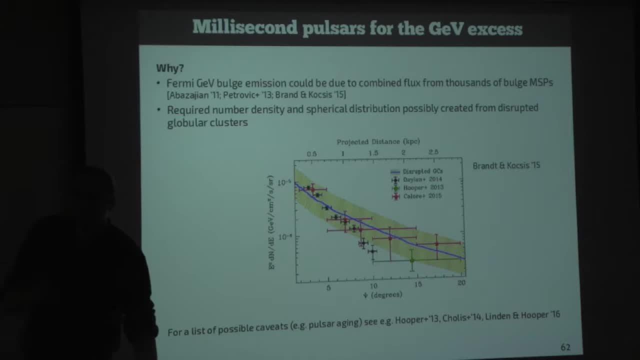 At least that's not necessary. How do you make the pulsar in the emission? Ah, the pulsar might be just a remnant of the supernova explosion. Okay, so you do not necessarily need dense stellar systems for this, but it can help. 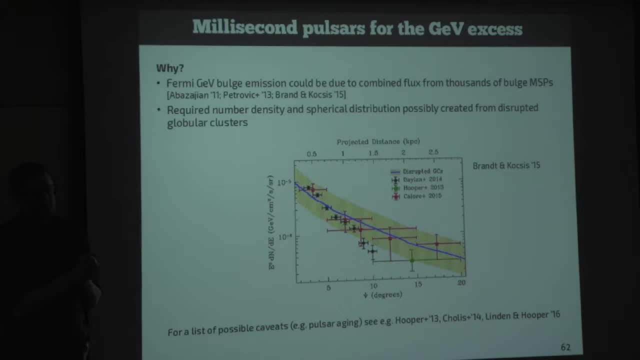 So one idea was globular clusters, which are very dense stellar systems and they are known to harbor lots of millisecond pulsars. So we see globular clusters and there is this effect that globular clusters are disrupted by tidal forces and then the debris 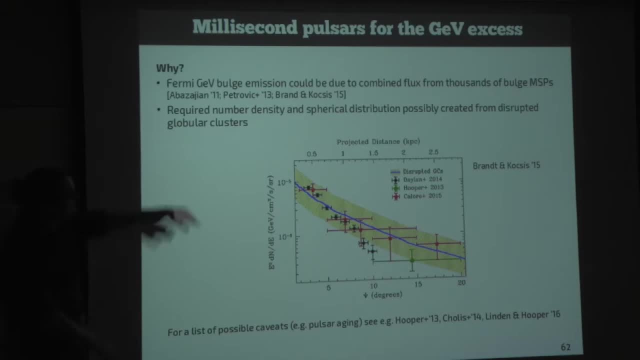 is redistributed in the inner galaxy. And it happens to be redistributed in a way- at least this is according to one model in one paper, and that matches pretty well the morphology of the GEV access. So one could imagine that millisecond pulsars. 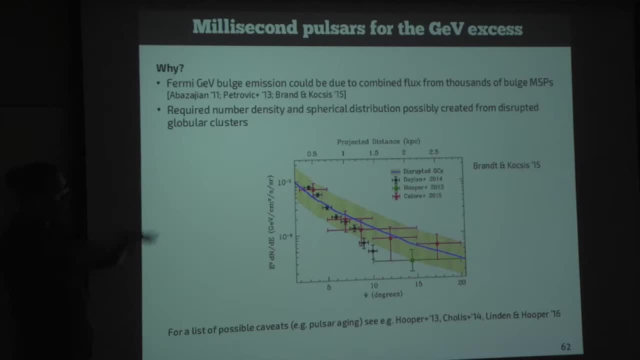 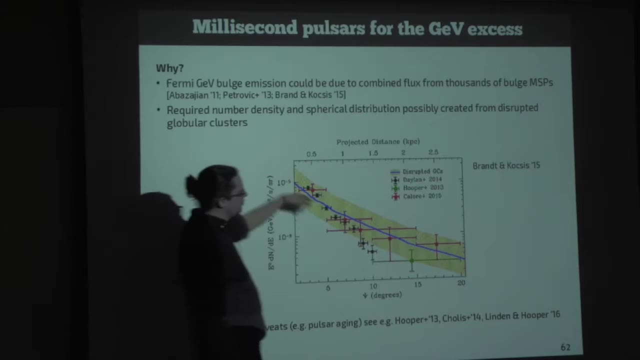 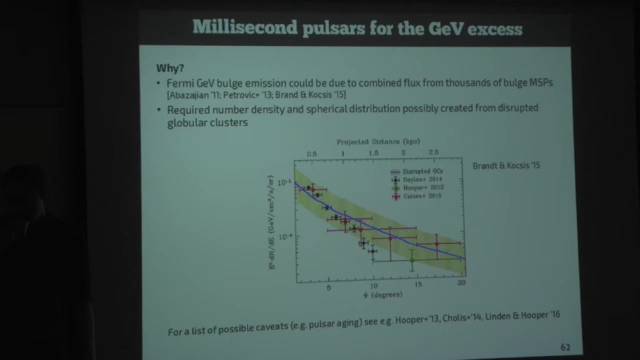 are produced in globular clusters, they are disrupted and the debris is redistributed in the inner galaxy. and millisecond pulsars can live billions of years in principle, and this would be one way how to Do. you need accretion always to generate a millisecond to speed up. Yes, you need the accretion of material Always, So they have to be born in a binary. Yes, so millisecond pulsars are always born in binary systems because regular pulsars have. I don't have the plot here. 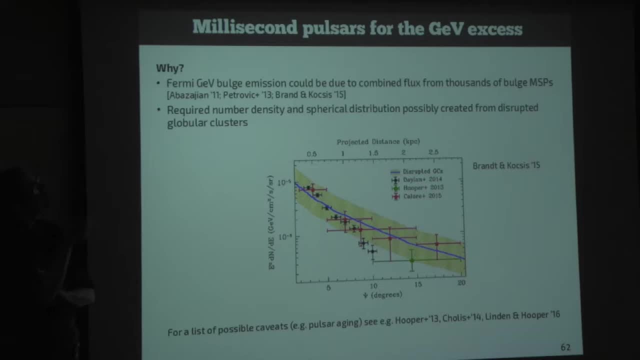 but their rotation frequency goes down to seconds or maybe below seconds, 0.1 seconds or whatever, but you don't get down to milliseconds. Millisecond is only for accretion, Yes, But they are surprisingly common. so Fermi found many more. 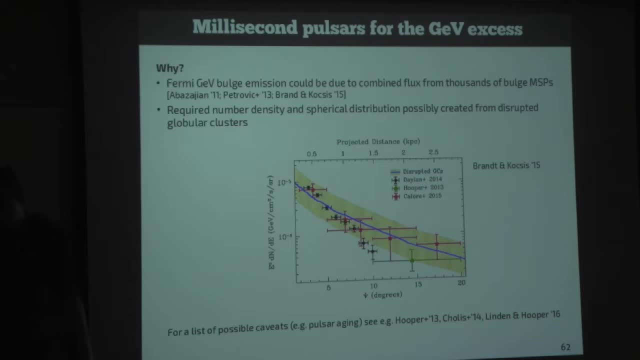 than they initially expected, in gamma rays, for instance. But you don't see them far away, right? Yeah, I'll come to this in a second. So you don't see them far away. up to now, that's true, But yeah, we'll discuss this a bit later. 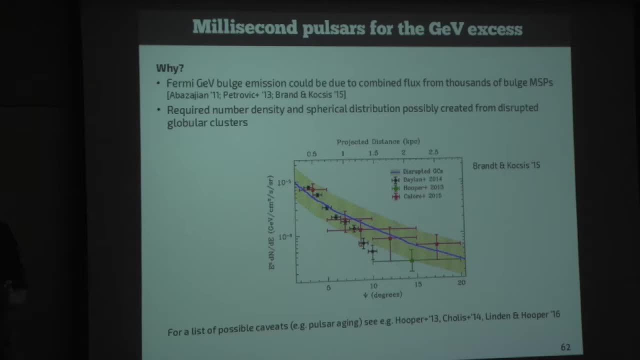 So all this thing about this is just Speculation? Yes, But it's, I think, promising speculation, and I will come to. I will explain how to. Is it good speculation or is it just? It's a testable model and we will test it very soon. 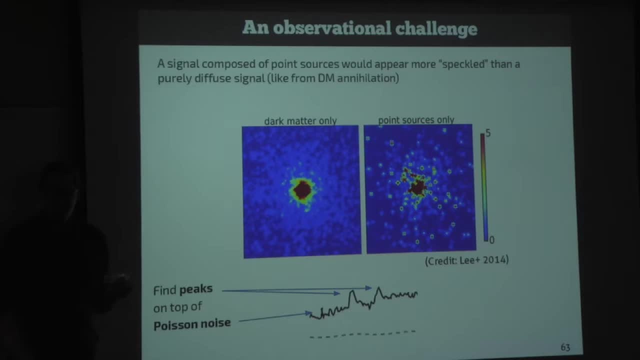 and I think it's the best explanation and I I would bet some money on it's right, but that's maybe wrong anyway, But it's testable and I will explain it in a second. I bet a lot of time on it. 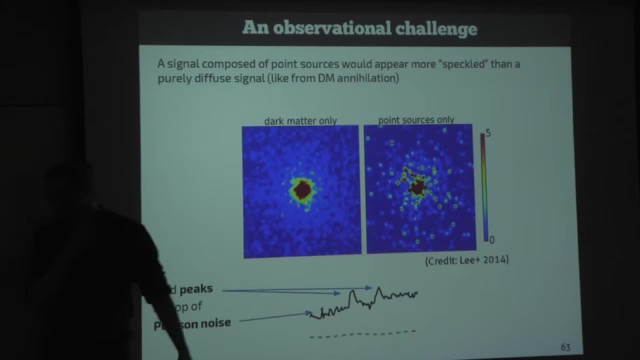 A lot of time. Yes, I don't know how much my time is worth, but I mean it's Anyway. So an observational challenge Right On the gamma ray side. actually, the problem is that dark matter would look pretty much like points. 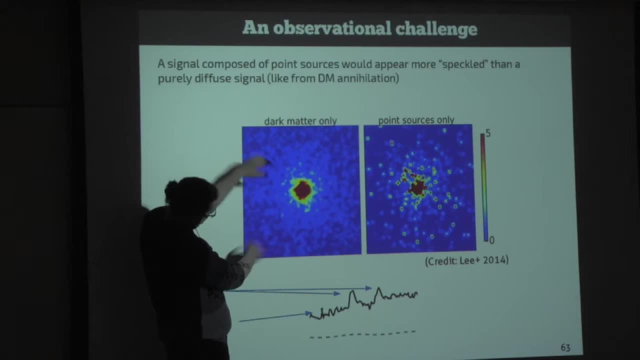 Yeah, Dark matter would look like this, with noise on top of that where, as if it's point sources, it would look like more speckled And to say whether it's this or that, one basically has to find non-Polsonian peaks on top of Poisson noise. 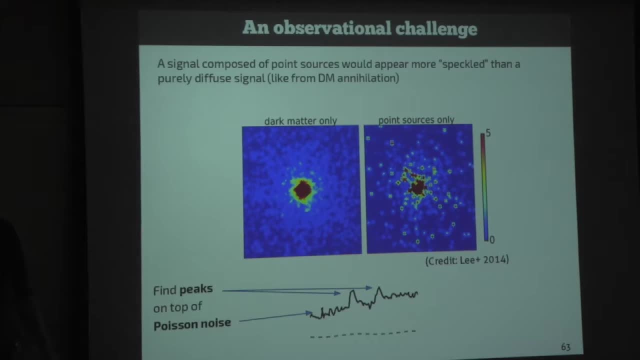 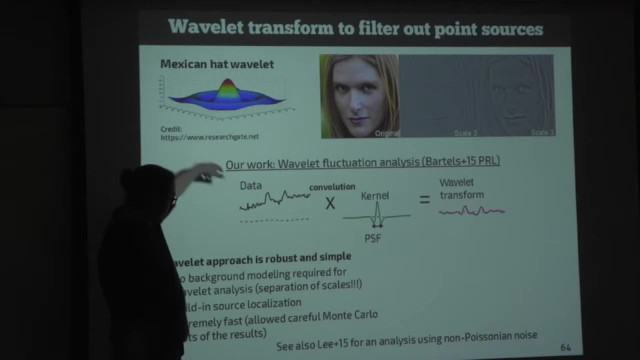 The problem is that if it's millisecond passes, then even the brightest ones would be just bright enough to be detected by Fermi. So that's hard. So what we did a couple of years ago- I'll just go quickly over this- is just taking. 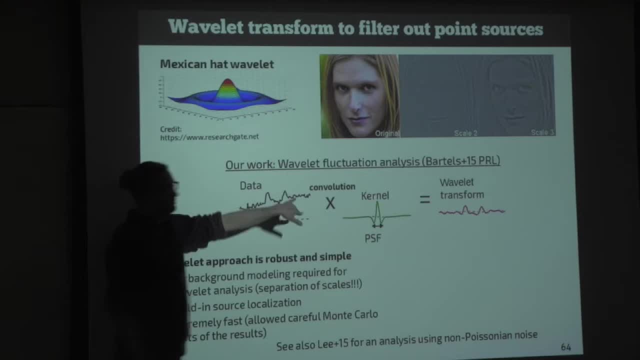 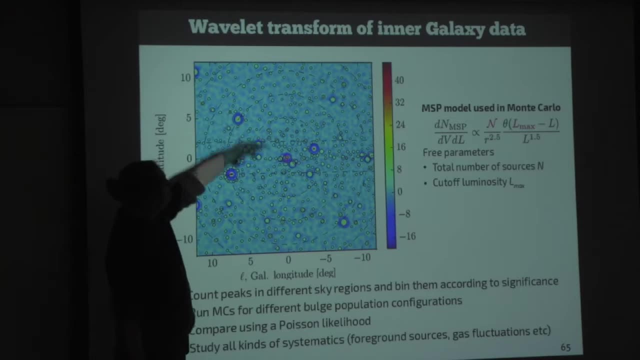 the data and then use like a wavelength analysis to pick out wannabe point sources at the three, four sigma level, And then one can do a Monte Carlo. So these are the wannabe point sources. Some of them are real point sources identified by Fermi. but there's also lots of noise. 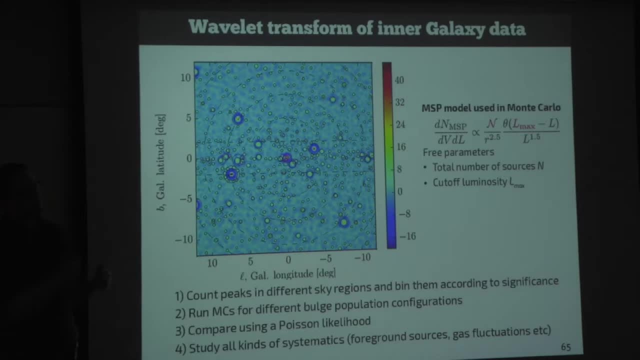 And then some might be actually millisecond passes that are not bright enough to make it into the Fermi point source catalog. But one can just Monte Carlo how many of these peaks one would see if there are no millisecond passes and how many one would see if there are millisecond passes. 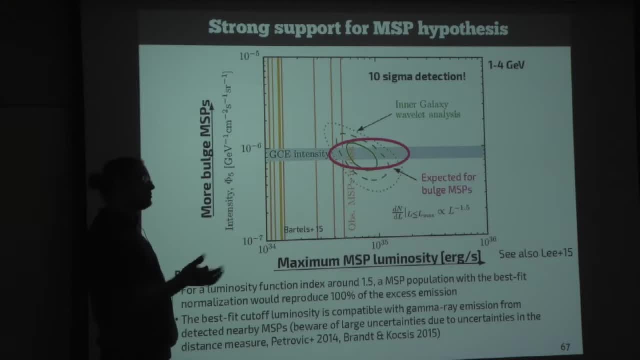 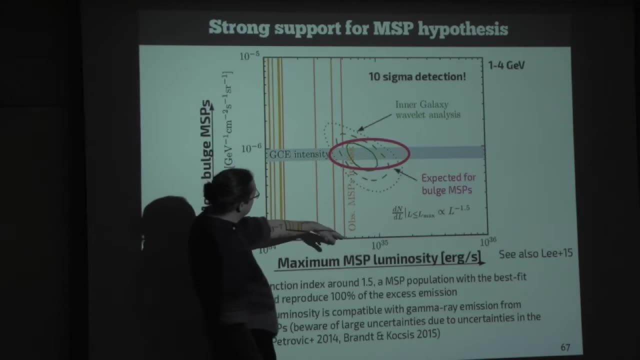 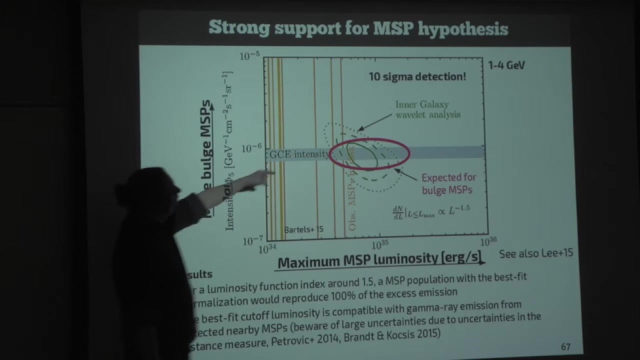 And it turns out that we first had a quite significant detection, so deviation basically from what you would expect just from Poisson noise, And that the best fit values that we had for the density of these sources and for the maximum luminosities that these sources have agrees pretty well with what one would expect from. 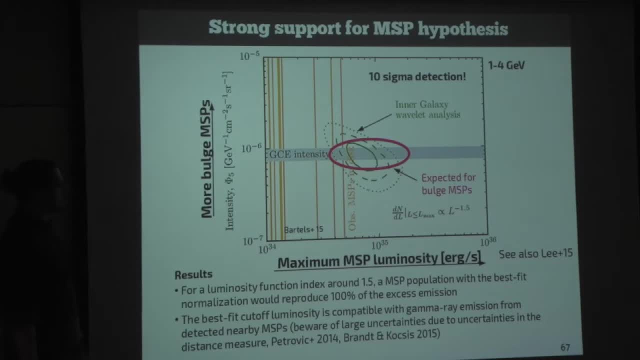 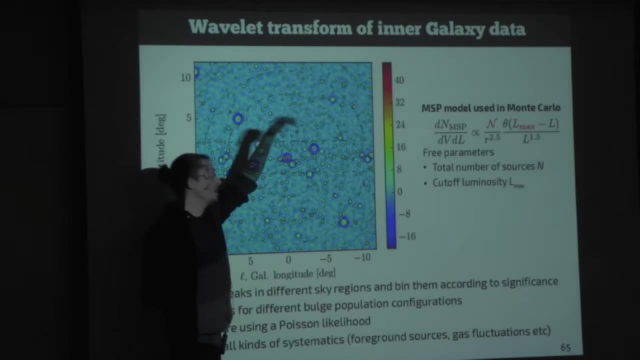 millisecond passes explaining 100% of the GEV excess. So basically, what we did is we counted the number of peaks- one sigma, two sigma, three sigma, four sigma, five sigma peaks- and compared it with a simple model where we have the number. 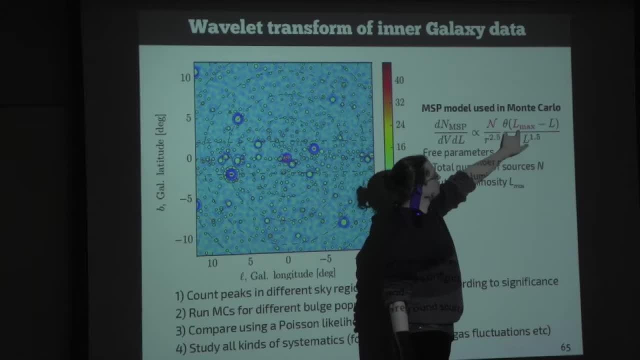 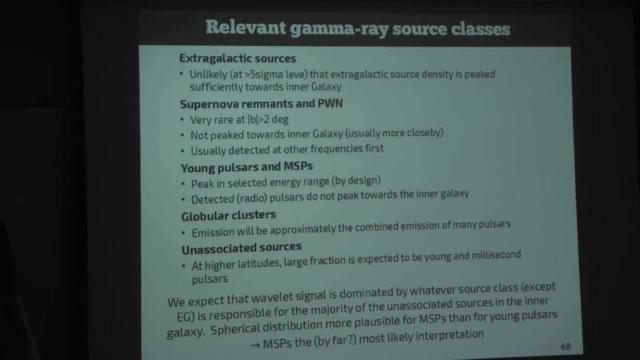 of millisecond passes free and the luminosity function with a fixed slope and a hard cutoff And the cutoff was free to move. OK, Good, So this was a nice result. Suggests that it's millisecond passes. Still, it's a quite indirect result. 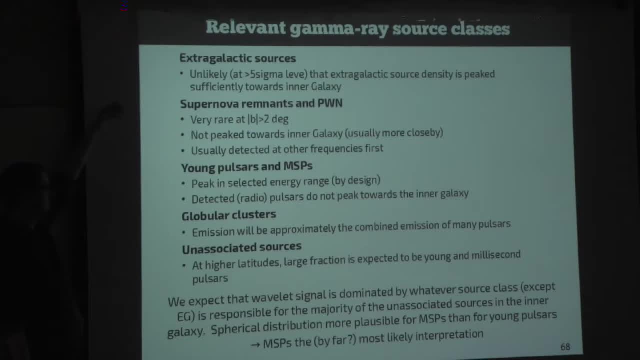 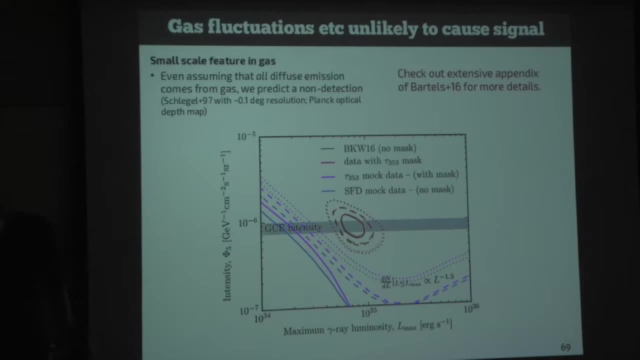 One can think about lots of caveats. First, other sources. I think one can go through the other source list and it's pretty unlikely that any of them matters. What matters, however, might simply be because either sources are extragalactic and then 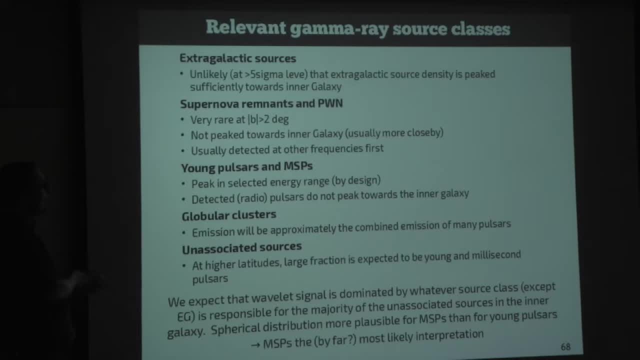 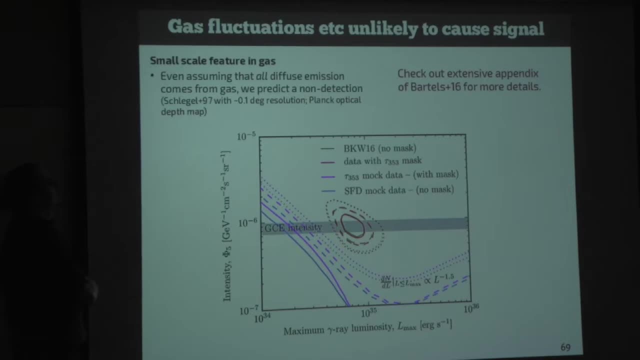 they don't just accumulate around the inner galaxy Right, Or the sources are galactic, and then they're usually in the disk. So that's the main reason. And then there are millisecond passes, but they are millisecond passes. So this would be what we wanted to look for. 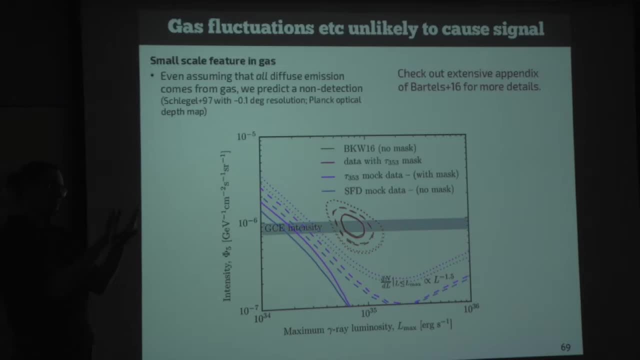 Gas fluctuations are maybe a concern. if one does this wavelength analysis, Then also gas has substructure and could contribute. But we tried this And in principle it could contribute quite a lot. But we can just mask at least the known regions that are problematic. 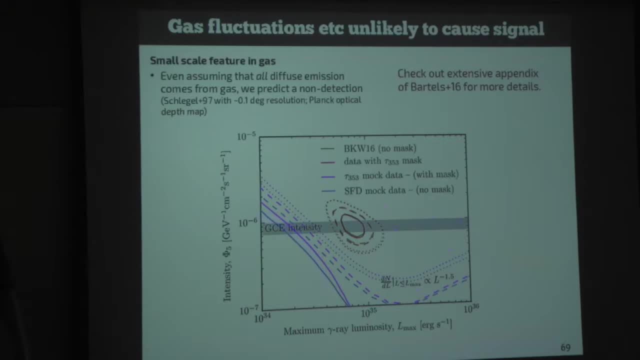 And this doesn't seem to affect the results. Still, this is no proof, obviously. How much time do I have? Oh, you don't worry exactly, Yeah, but I have a lot of time. Ah, so you have time. 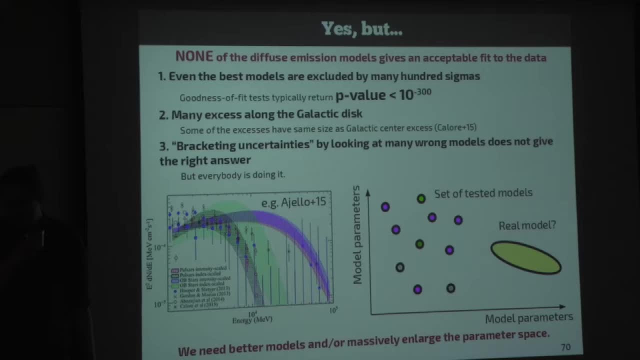 It's too much. even So, it should go to what? 12, sorry, no, 11.20. OK, 11.20.. 11.20,. you have like 15 minutes, Yeah, OK. 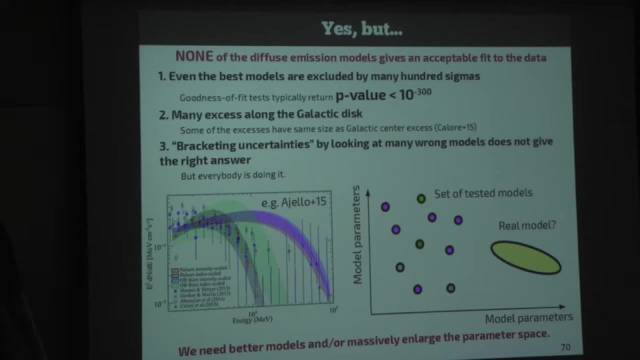 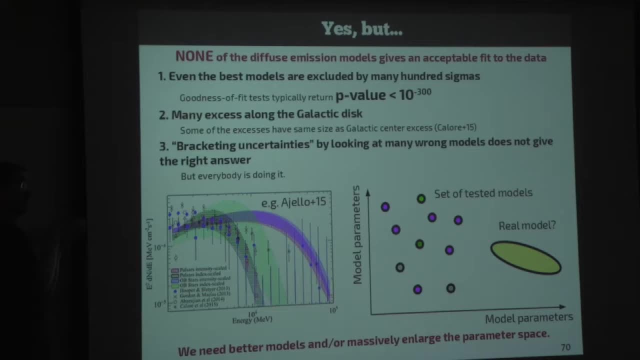 So I wanted to talk. So I will then talk about two things: One, our attempt to make galactic diffuse emission modeling a bit better by basically introducing hundreds of thousands of additional parameters, And another is how to test this Pulsar hypothesis in the near future, which is probably yeah. 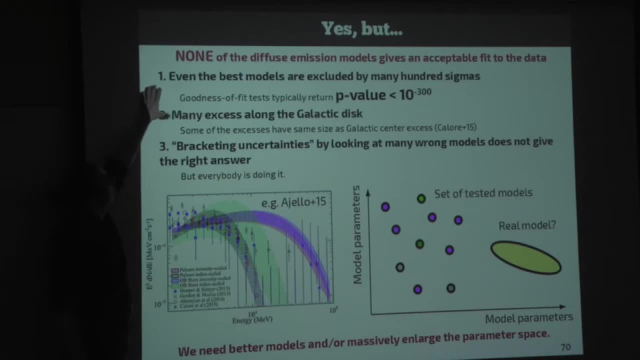 which would be pretty useful. Good. So the fun thing with these galactic diffuse emission models, submission models, is that if you look actually at goodness of fit, then it's ridiculously bad. So if you calculate the p value- I did this once- you typically get something around. 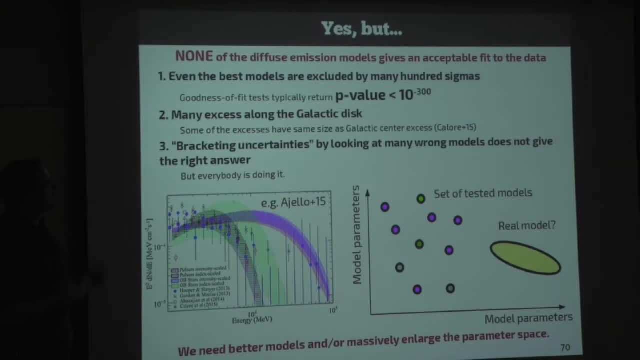 10 to minus 300 or something, because the models just don't fit the data, So they just don't fit And there are many excesses along the galactic disk, So we pointed this out in 2014.. Many other people. 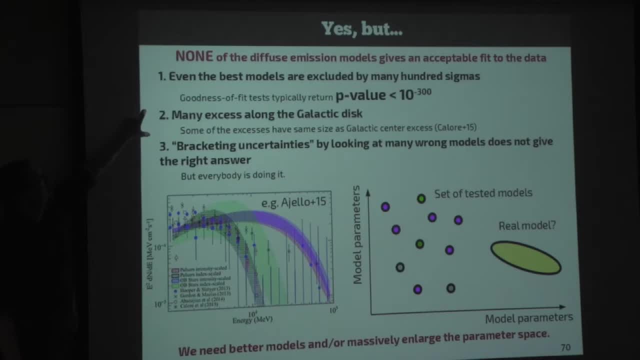 pointed this out as well. The interesting thing is the excesses have a different spectrum, so the thing at the galactic center is peculiar but still you might worry about. okay, there are lots of excesses, And then the usual way uncertainties are bracketed is by just 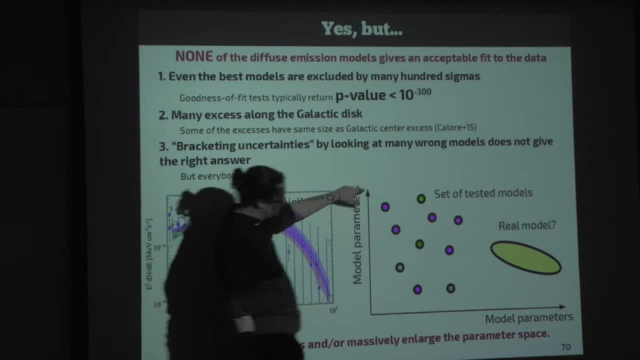 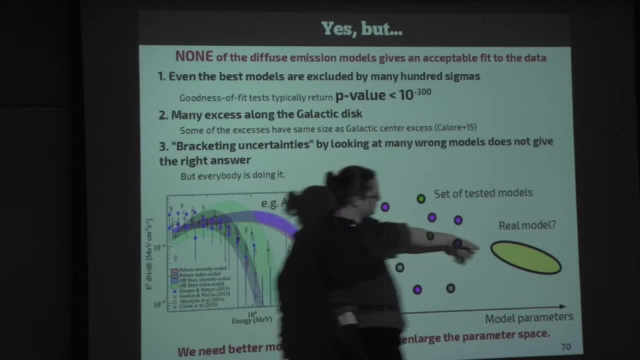 having a bunch of benchmark models and seeing then what are the results. But usually this is what happens. You have model parameters, you have tiny statistical error bars, you have different benchmark models and this all doesn't agree. Maybe the real model is over here and has a 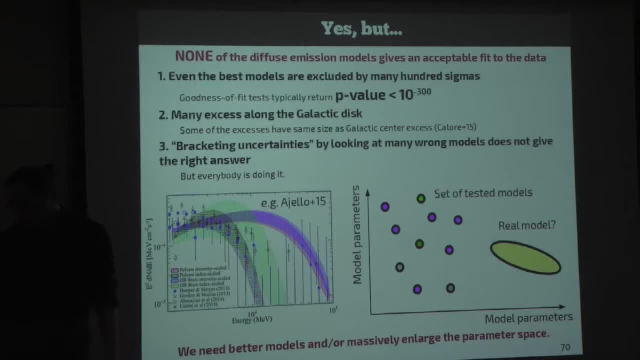 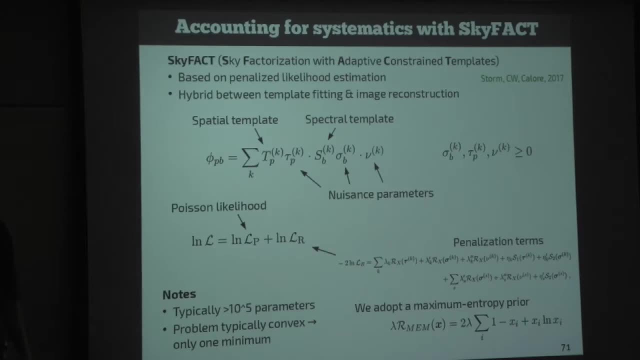 much larger error bar. So obviously, what one needs to do is to massively increase the number of parameters in some smart way that is not completely arbitrary, And this is what we tried with a new analysis tool that we called SkyFact for sky factorization, with adaptive constraint templates, and 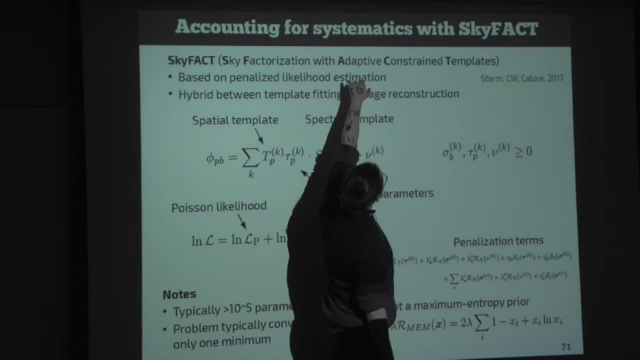 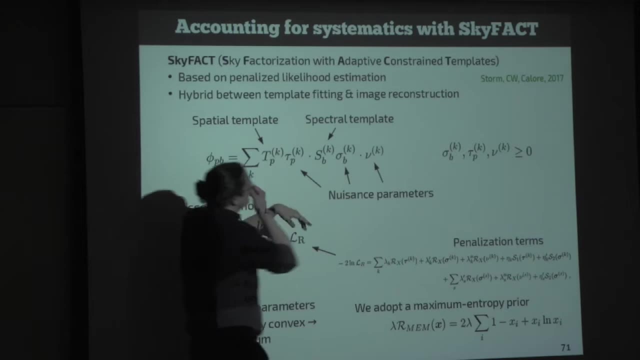 that's basically what it's done. So it starts with templates which can adapt to the data, so they have some nuisance parameters which are constrained. so it's like a penalized likelihood function And it's a factorization ansatz in the same. 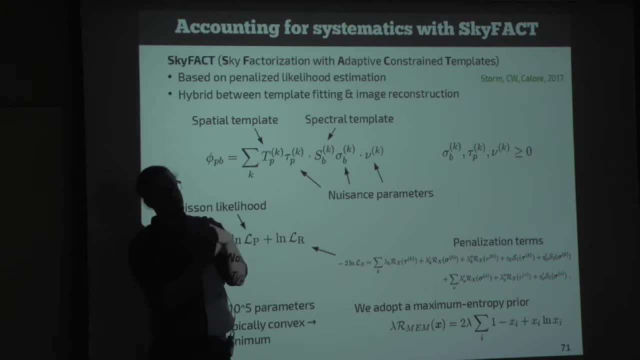 sense that we start with templates and then we assume that the nuisance parameters, that there are spatial nuisance parameters and spectral nuisance parameters, And this is basically how it works. So this would be the flux that we see in each pixel. This is the prediction. 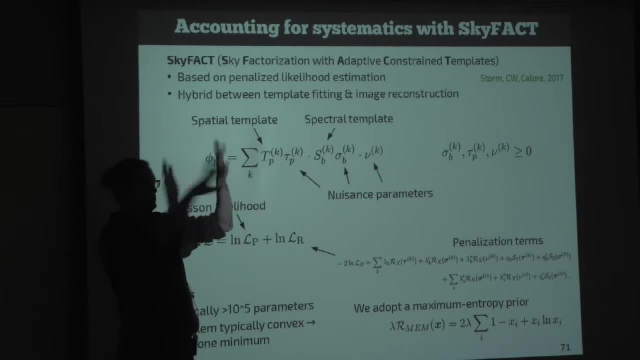 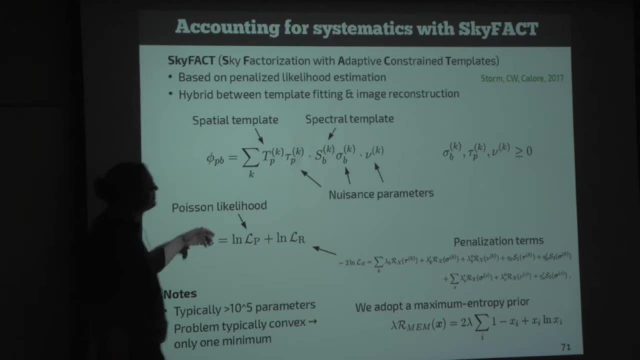 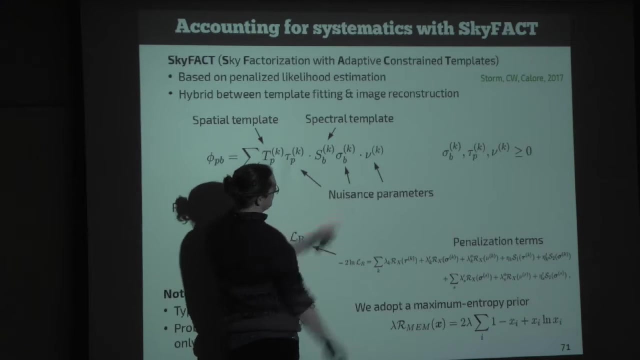 the spatial prediction of the flux, So this might be a sky map. This here would be the spectrum predicted for this component by GuyProp or whatever code, And these are nuisance parameters that can modify the template, the spatial template or the spectrum, And this is all. 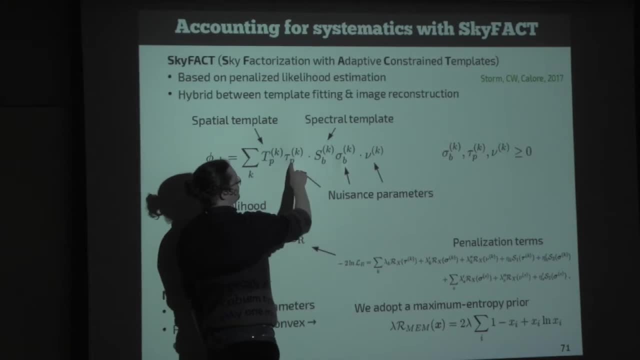 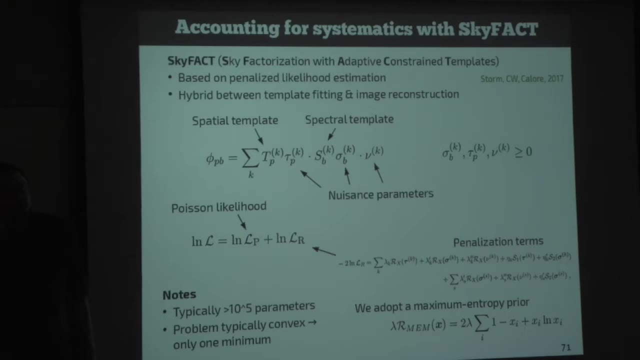 overall normalization, And these factors here are usually around one. so one point, one point nine. So they introduce tiny variations of the individual components at the ten, twenty, thirty percent level, or sometimes more, And then the likelihood that is fit is the Poisson likelihood that compares. 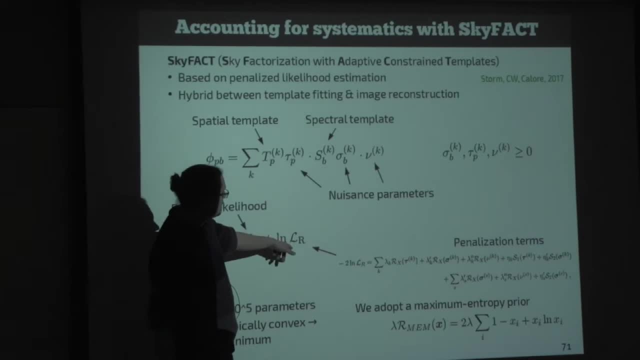 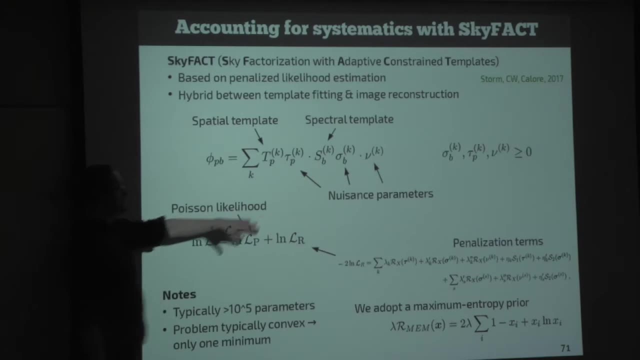 data with the model plus the part that includes penalization terms. So this I don't go into details, but basically these ensure that the nuisance parameters cannot be arbitrarily far away from one, And there's also some smoothing going on to avoid that all the Poisson noise. 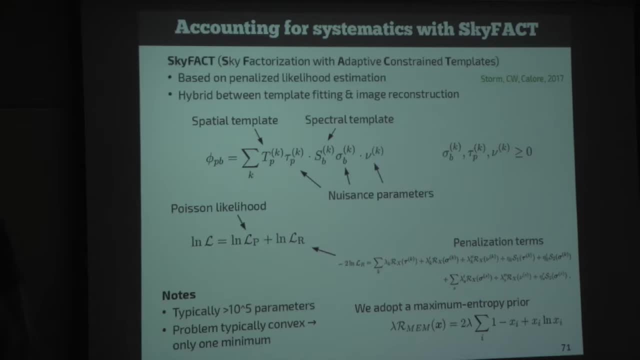 is just absorbed into the nuisance parameters, And typically this model for the analysis that we made up to now has ten to the five parameters. But one can show that this thing is a convex problem and then one can code up gradient descent and it works. 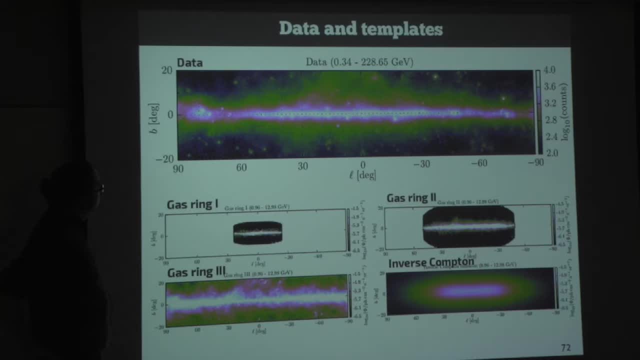 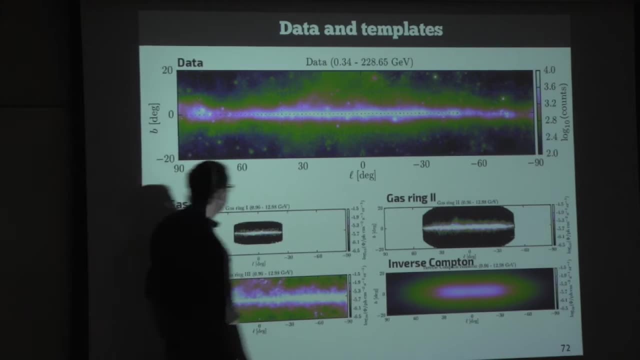 So just to quickly go through this. so what we did recently was to analyze again the galactic disk, So this galactic disk, galactic center here, with various components. These are just some of them. So various gas rings- This would be inner part. 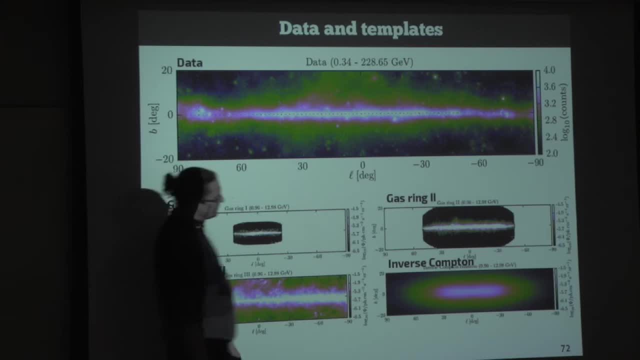 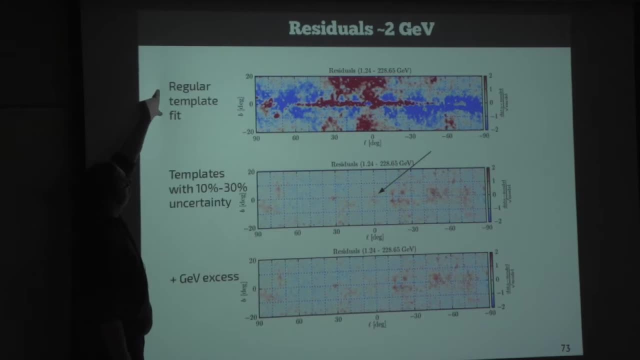 of the galaxy. This would be the one, the gas ring that contains us Plus one inverse component template that looks like this: And if one does a fit to the data with a regular template fit, these are the residuals that you get at one GeV. 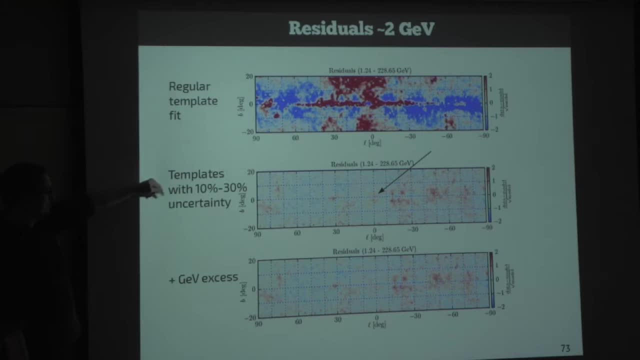 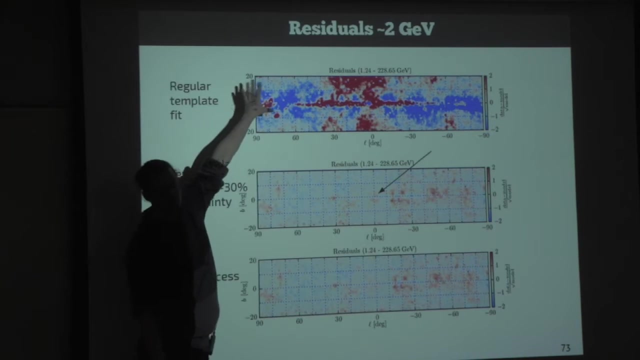 If one switches on the template uncertainties usually at the ten to thirty percent level, for inverse they were somewhat larger. Then the residuals look like this: So these are suddenly just residuals at the still one sigma. This is at the few sigma level, but this here were much stronger. 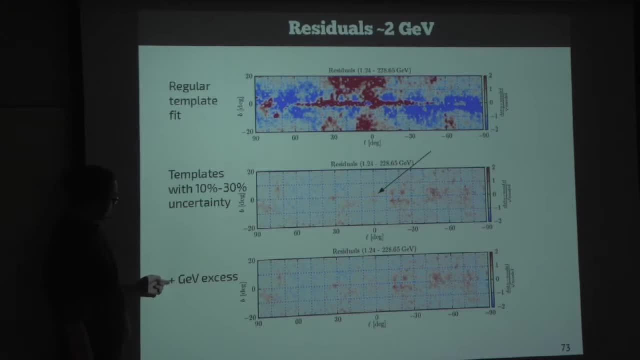 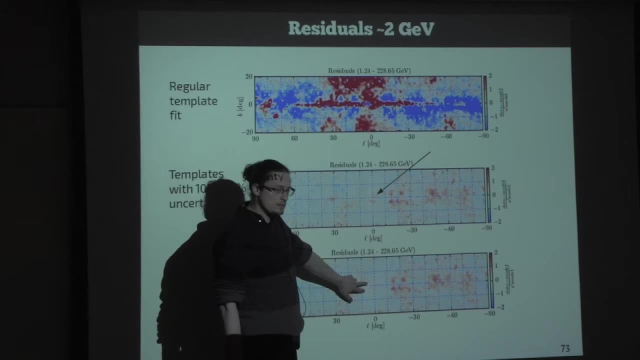 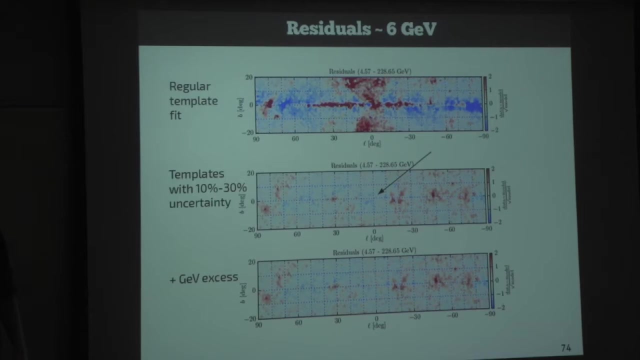 residuals, obviously, And this is when the GeV access is included, And you don't really see the difference here. So here's the tiny residual, Here's the residual. here the residual is kind of weaker, And if you now compare this with six GeV, 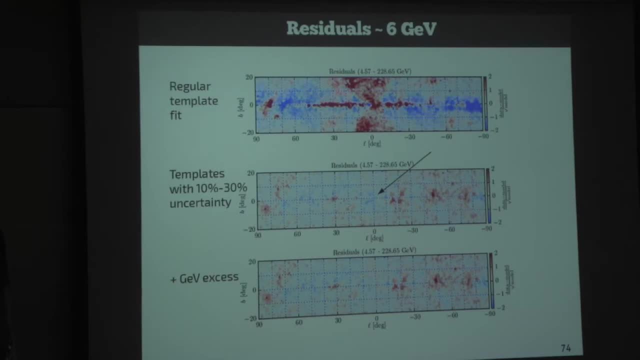 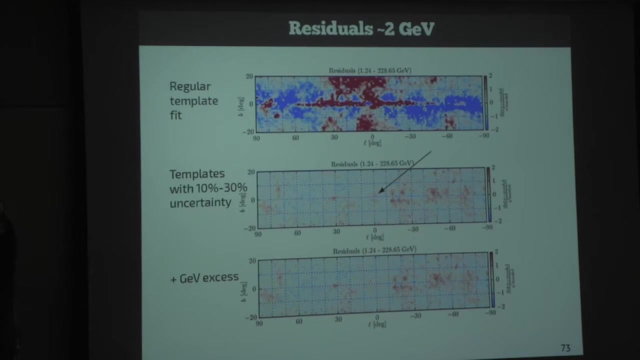 it looks basically the same, But what you see first is that at six GeV the access has become somewhat stronger. So there are along the galactic disk some hard components that we don't model, But the one thing that you see is that the 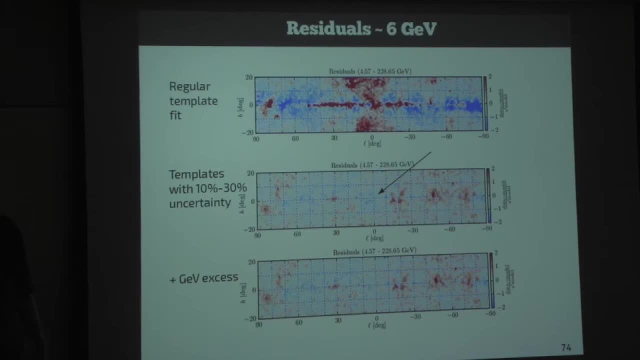 GeV access actually does exactly the opposite. So if you go to higher energies, it becomes blue, Which means before you were under subtracting, afterwards you were over subtracting, And this doesn't happen for anything else really in the sky. So this is what. 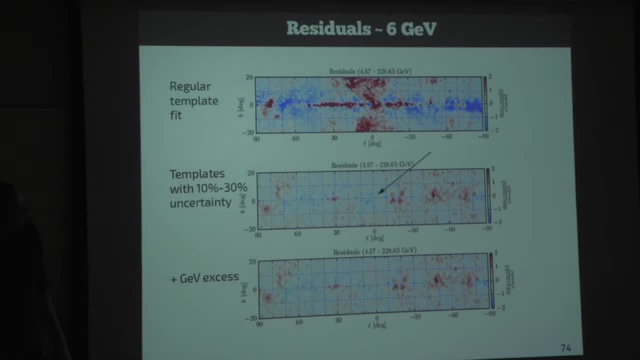 is peculiar about the GeV access And it basically means that this thing here has a harder spectrum, at least at low energies, So around one GeV, then most of the other things that you see in the galactic disk, Whereas this here, are probably extended. 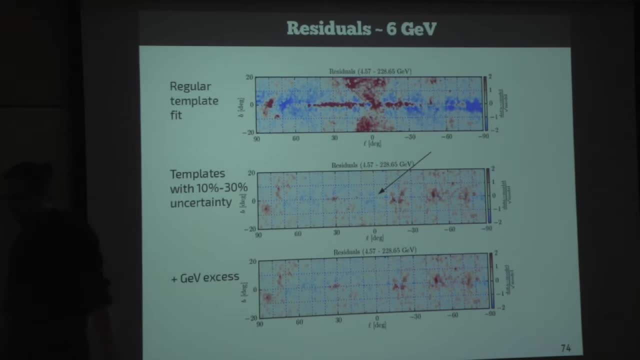 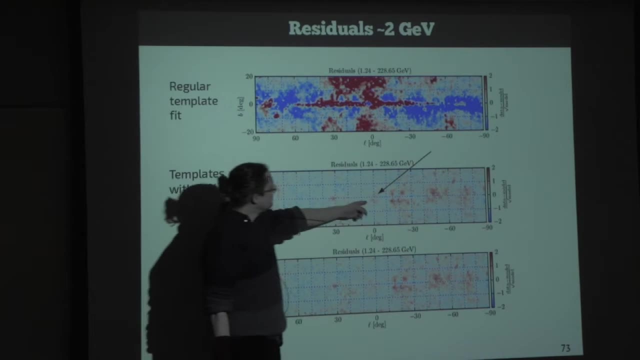 emission around sources that you also see in Hess. Where is the GeV? Yeah right, That's like the left, You can't barely see it, But it's basically this thing here. So here it's red If I go to. 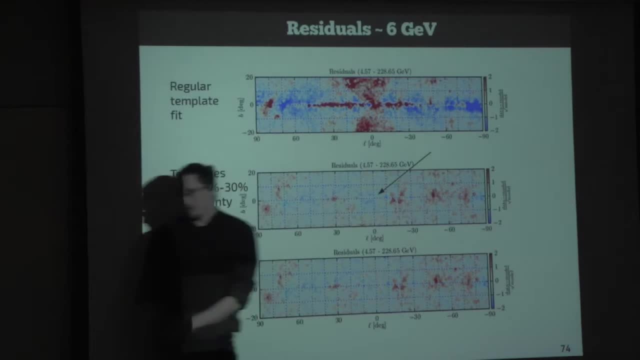 higher energies it turns blue, Whereas all the other- I mean you have brighter residuals in the disk, but they are red and just turn more red. What this means, if you translate this in spectrum, is simply that these accesses here have a relatively hard 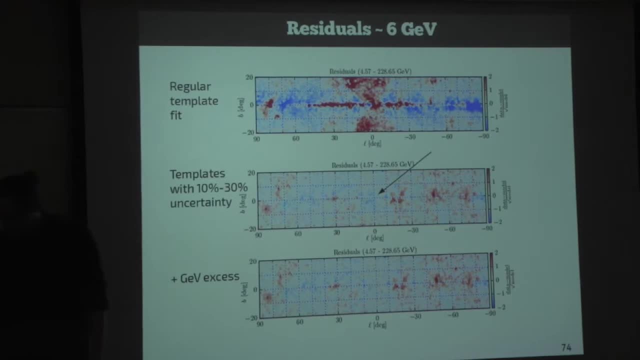 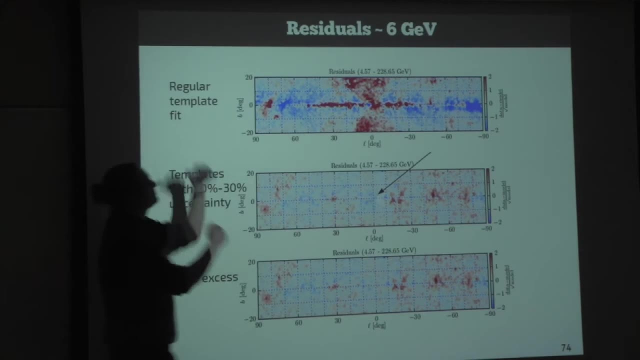 spectrum, Whereas the spectrum from this thing here is going down faster. So I can show it like maybe here. So most of the accesses would have a spectrum like this. The GeV access would have a spectrum like this And we are looking at this and this energy. 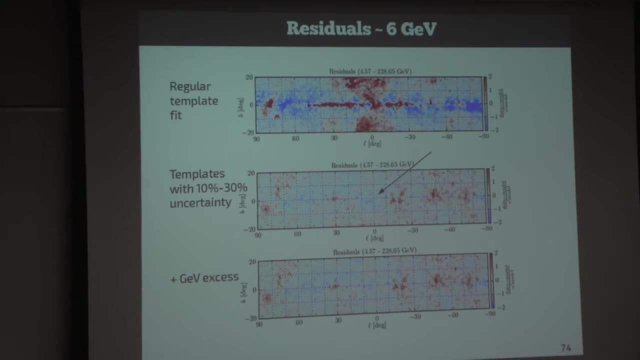 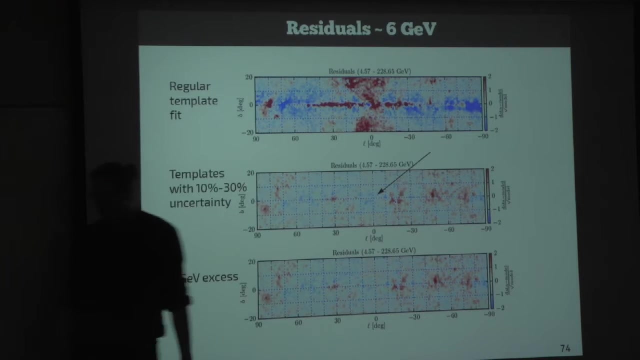 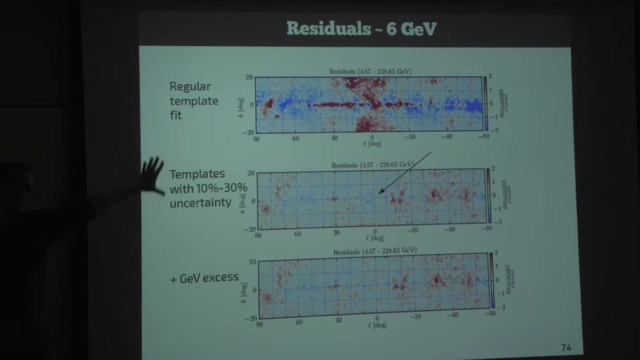 roughly So. this is why it looks slightly different here. If I would have had a slide below one GeV, then we would have seen the opposite effect again. So it doesn't look very significant here. But I'm not advocating that the GeV access is not significant or not. 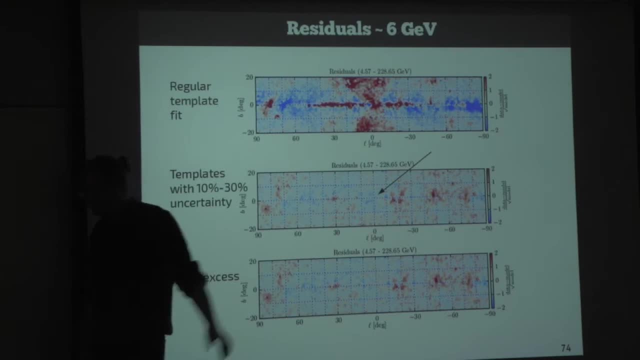 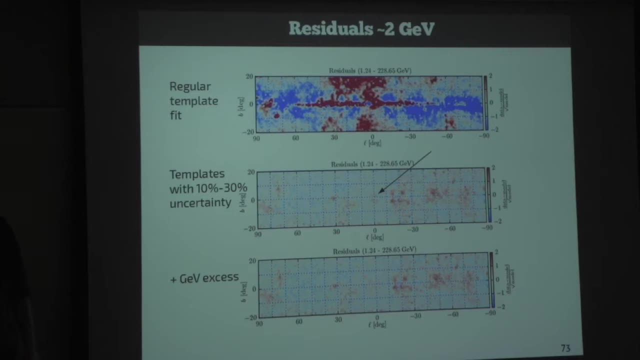 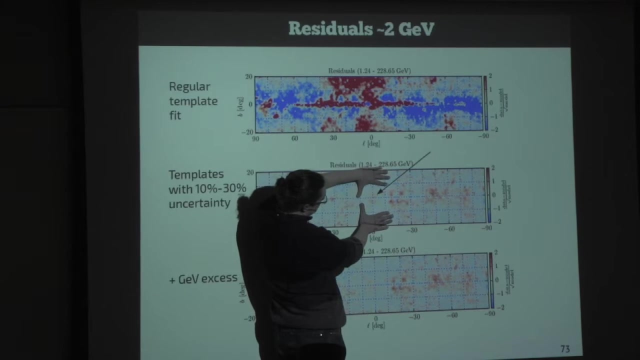 there. I'm mostly advocating that often residual maps are not very helpful to find anything or to show anything. So how big should it be in this map? I cannot see anything. It's tiny here, but the idea is that the entire thing is extended at least up to. 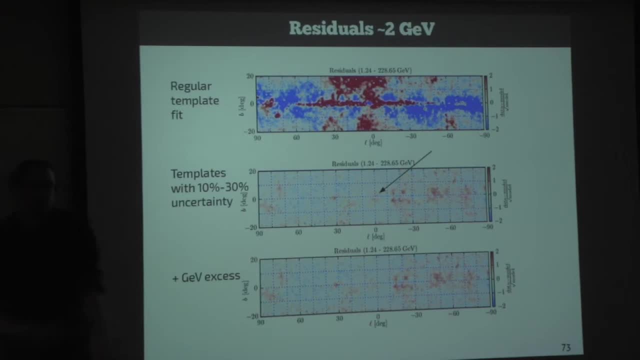 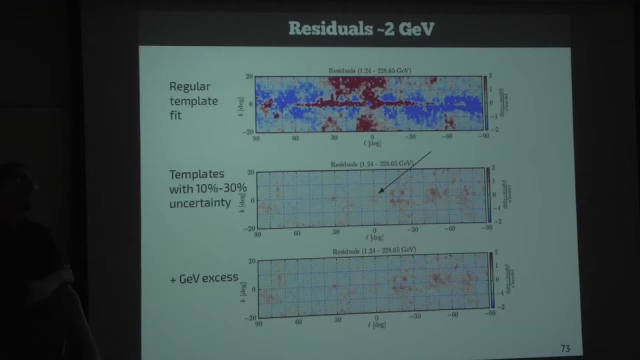 10 degrees, But there are other analyses where it's much more prominent. It depends a lot on how you do it. One way to make it very prominent is a paper by John Huang. If you just do a spectral decomposition of the sky and fit like a, 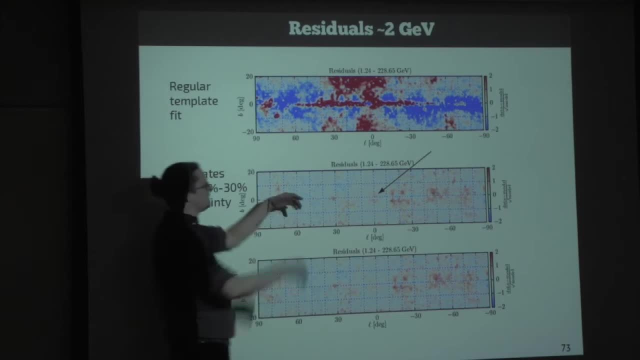 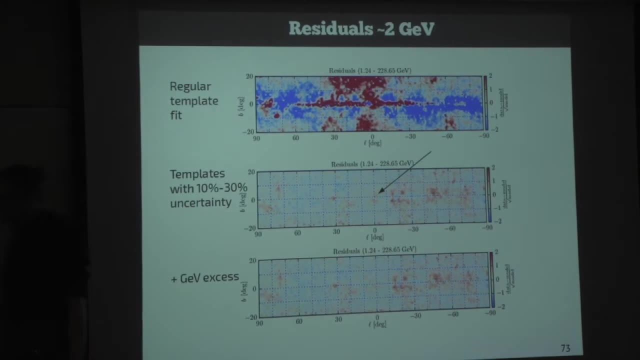 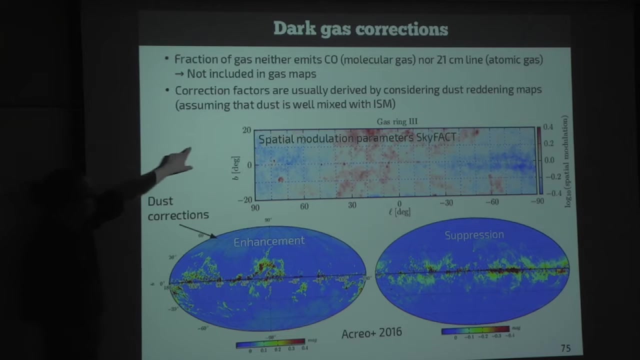 B-B-bar spectrum, or in that case they used B-B-bar and a bunch of other more like extended power laws, then you get a pretty significant access here in the center, Anyway. so this is just to show the spatial modulation parameters for the outer gas ring. 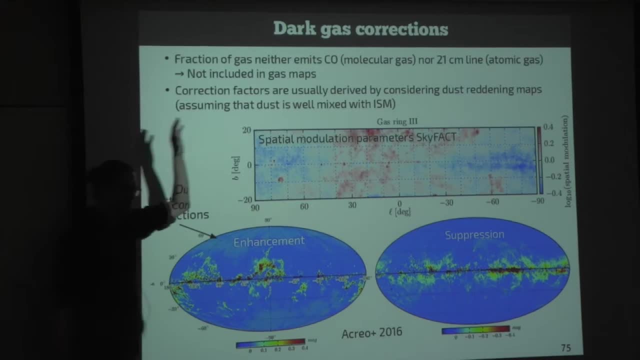 They simply absorb all the dark gas. There's something called dark gas which is not traced by a 21 cm line or the CO line. We didn't include these corrections in our analysis. They just came automatically because our rescaling factors could account for this. 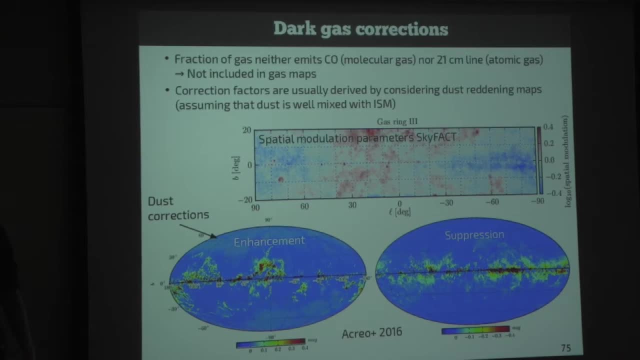 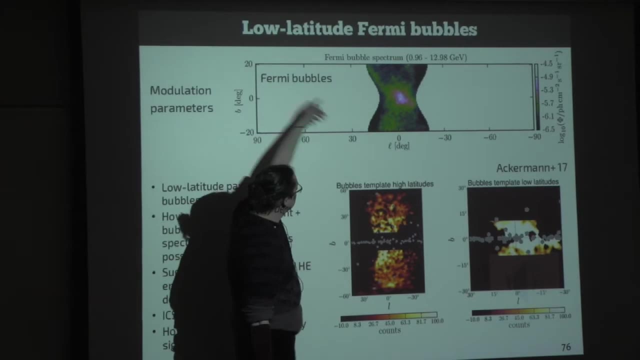 In the GALPROP papers. they usually include this, but that doesn't make a difference for us. For the Fermi bubbles, what we could find is that there- and this is what other people found before, but for us it was a bit cleaner- 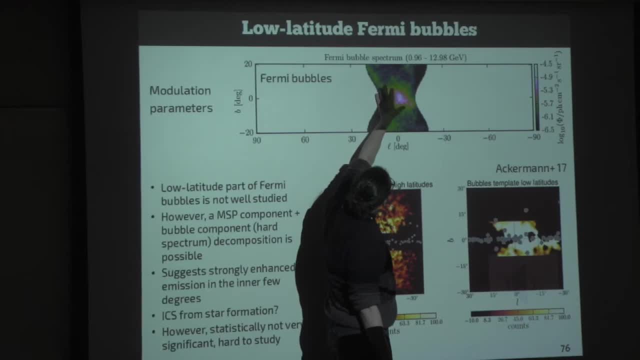 Instead of masking point sources, we also just fit all the point sources. We found that we have the Fermi bubbles here in this region, but then also some extra component that has a Fermi bubble that has a very hard spectrum. that is not part of what 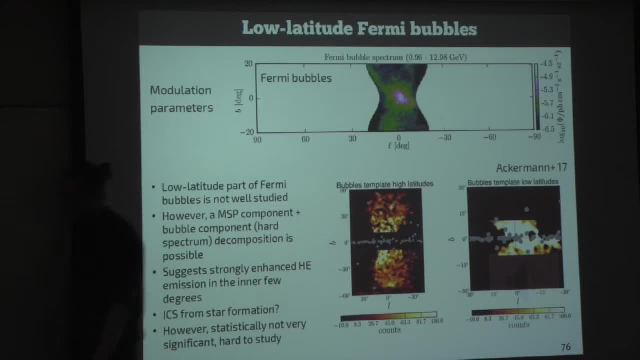 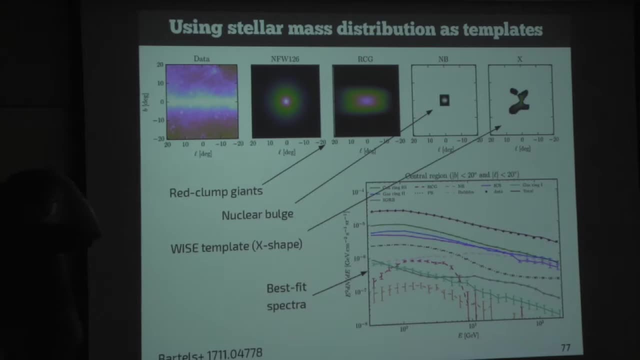 I would call V-access, but that seems to be there in the galactic center. Probably it's related to star formation activity. but that's future work. What we tried to do in a recent analysis was actually to just compare different models for the GV-access. This is the 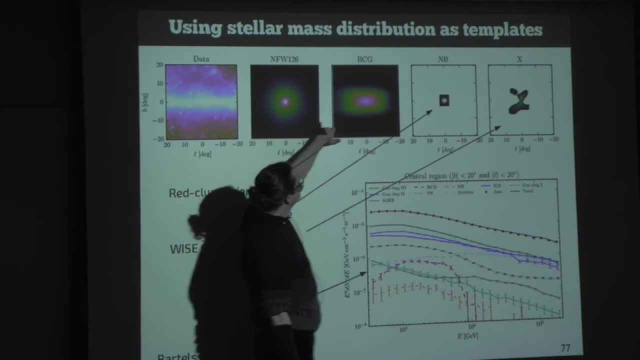 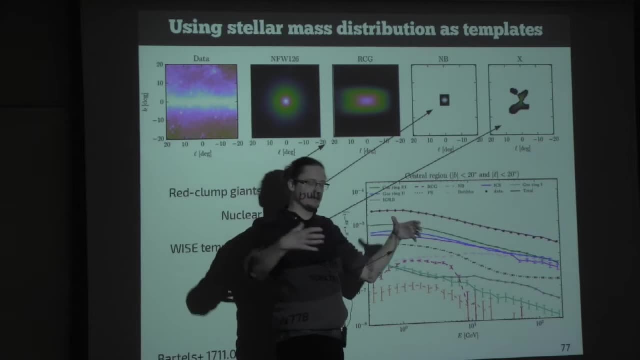 data. this would be in a contracted NFW profile for a dark matter signal, and this here are just templates for how stellar mass is distributed in the galactic disk. You know that the Milky Way actually has a bar, so this is how this 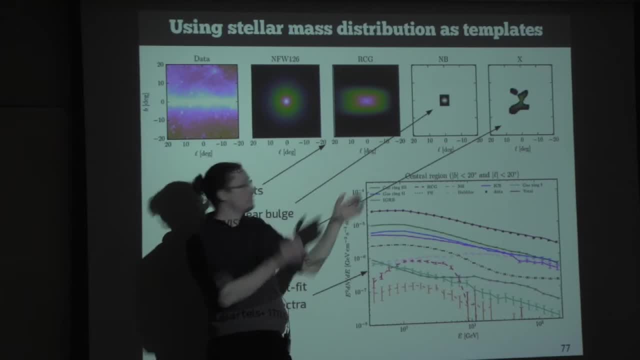 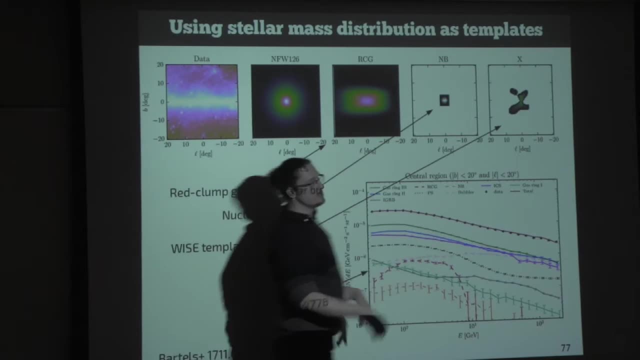 bar-like object would look if it would emit gamma rays. It's slightly extended and a bit thicker here, a bit box-shaped, and then there's a nuclear bulge. This is a disk plus some stellar, very dense component, And then we also tried to. 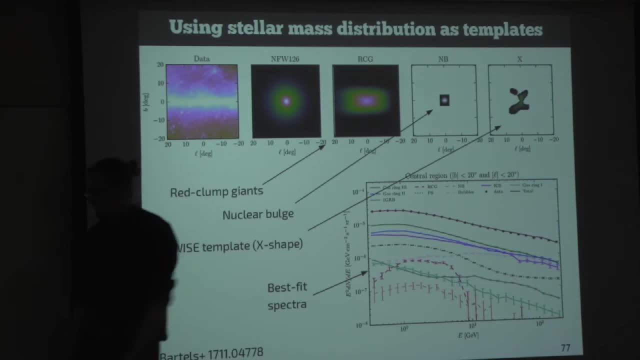 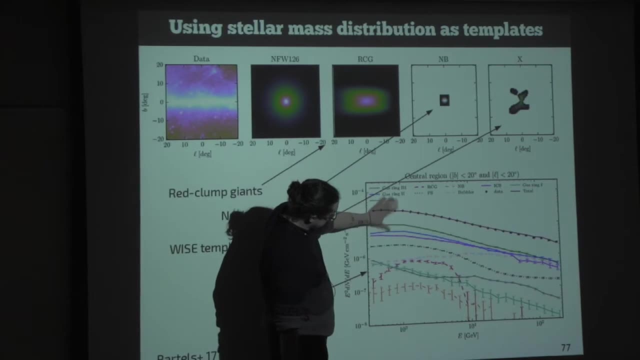 X-shaped thing, because this was proposed in other studies, that this could actually expand the GV-access. We do the analysis and basically this is what you find. These are all components in our fit and the red one is what is absorbed by the red cluster. 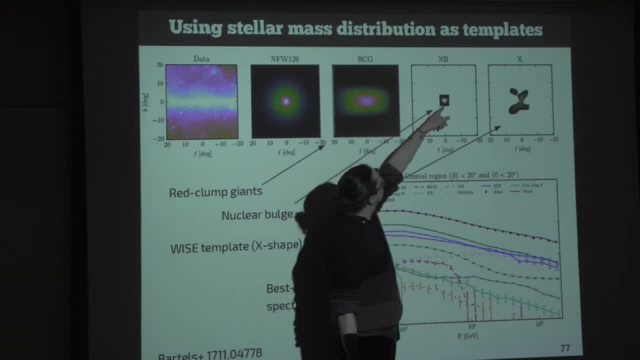 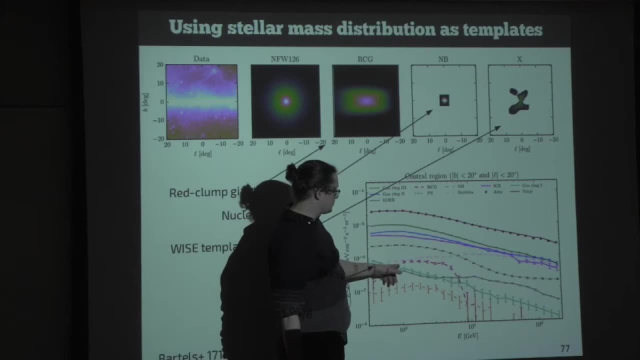 red clump giants and this yellow one is absorbed by the nuclear bulge. So you can see, at least for the red cluster giants, that they have clearly this typical GV-access spectrum that peaks here around a couple of GV and then it drops down. 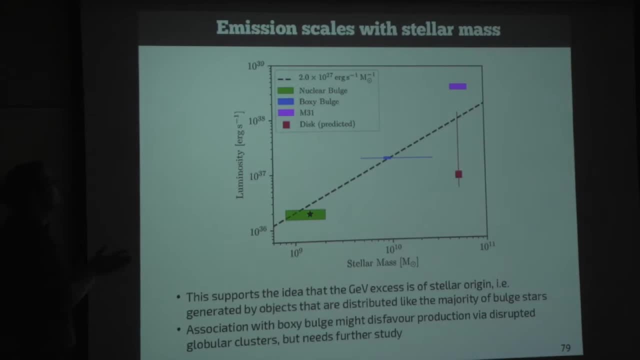 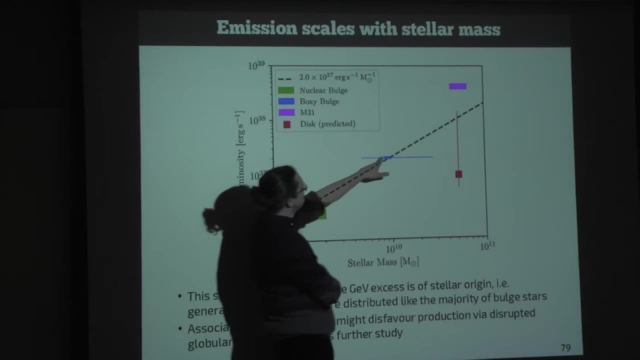 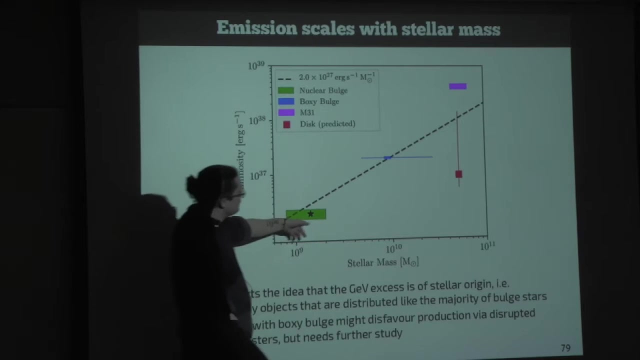 And what's interesting, what we found is that now, if one compares the emission from these components, from the nuclear bulge and from the boxy bulge, the gamma ray emission absorbed by the GV-access, with their actual stellar mass, then this is just a linear relation. 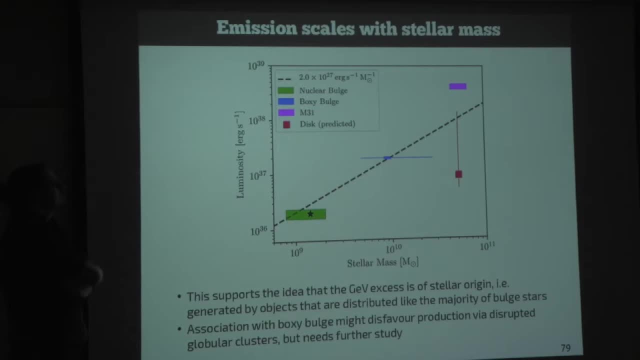 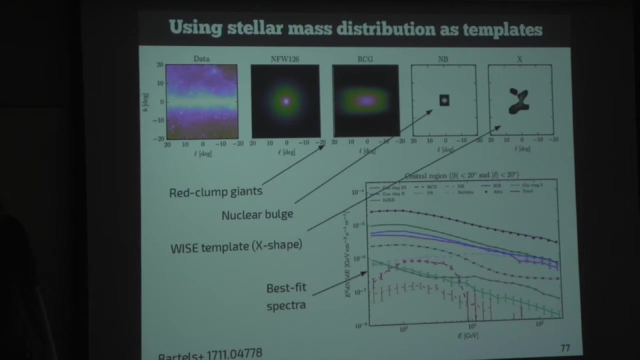 So this suggests that there is a connection between the distribution of stars in the galactic bulge and the GV-access. This could have looked very different, but it didn't. It's, in retrospect, not really a big surprise, because if you overlay this with this, 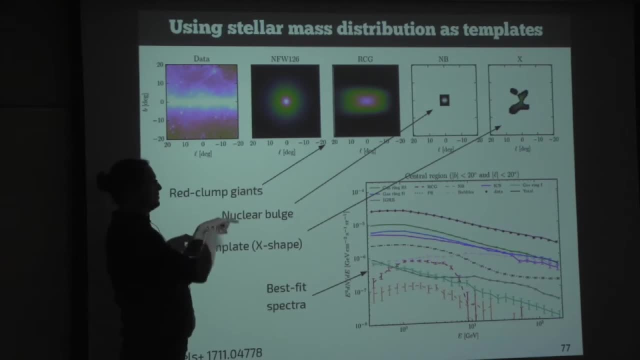 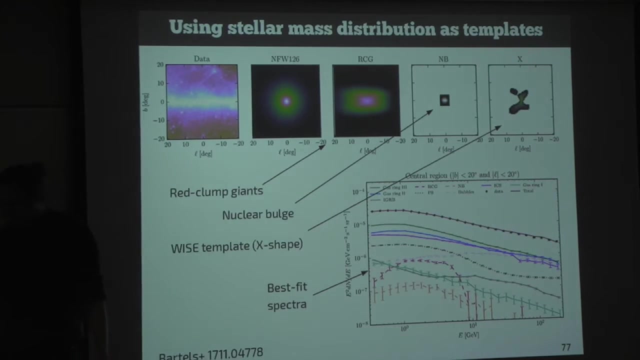 then on average, if you just do an average around different angles, it looks pretty much like a contracted NFW profile. But still, we also found that this combination here fits the data much better- by 10 sigma or something- than this shape. So this was a nice. 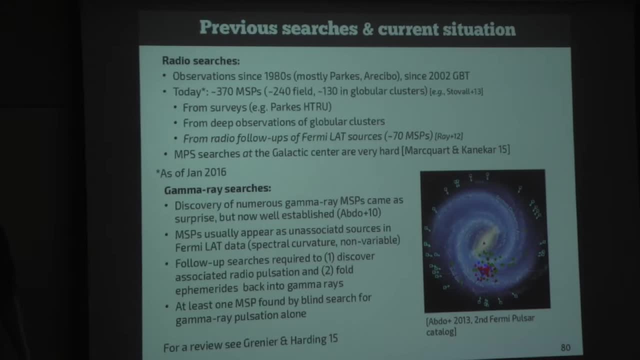 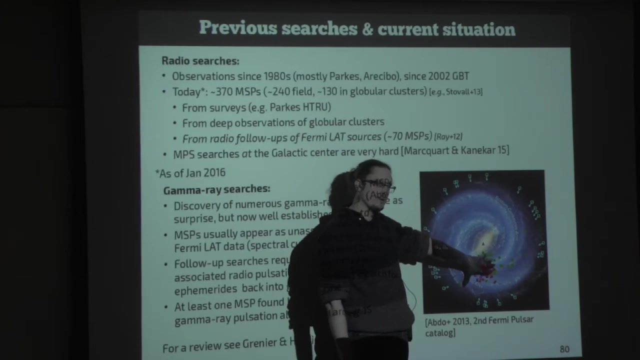 result. Still, that doesn't prove the GV-access is necessarily millisecond pulsars or related to the bar. What one needs is to actually find the millisecond pulsars, And so the situation there up to now still is that most millisecond pulsars that are found are found close to us. 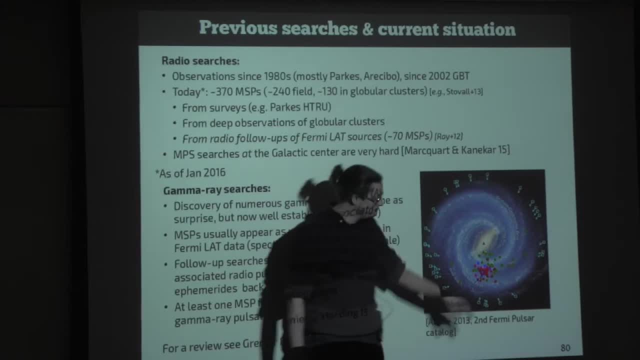 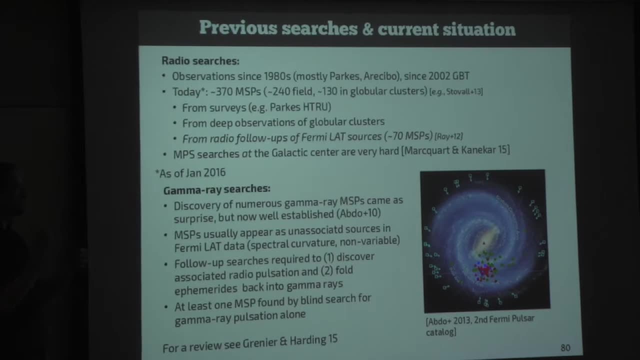 So this is where we are and most of the millisecond pulsars that are found close to us. The reason is simply that it's not so easy to find them Traditionally, you just found them. one way to find them is to look at distant globular clusters. 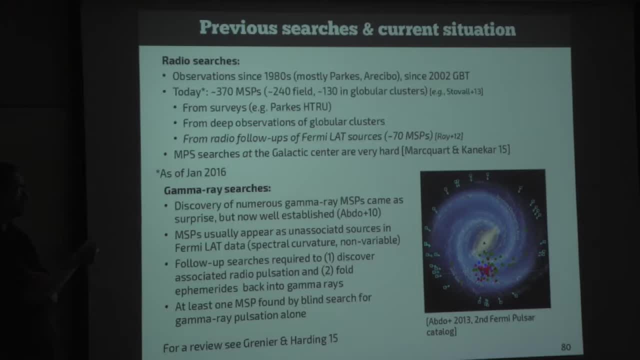 for instance, and then you look for a very long time with a radio telescope. This you can afford because you know where to look. The problem with radio telescopes, compared to Fermi, is that they have a usually tiny field of view, So you have to know where you want to look. 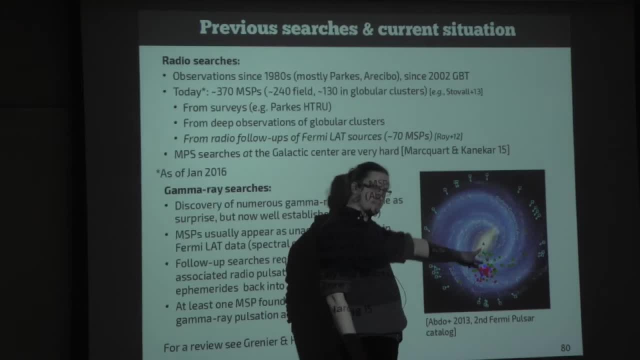 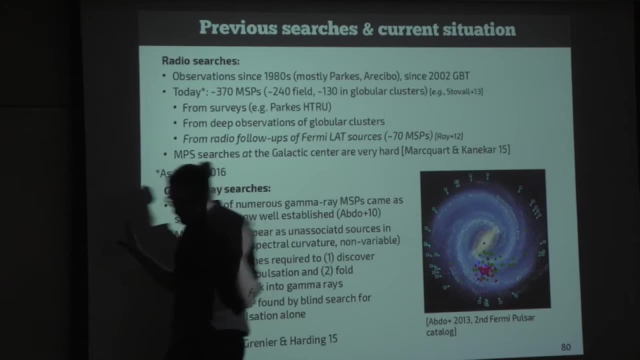 Then you can find distant ones, like this one here, which is not at the galactic center, It's above or below or something. Then the usual other way was just surveys, where you can't go that deep, so you find only close ones. 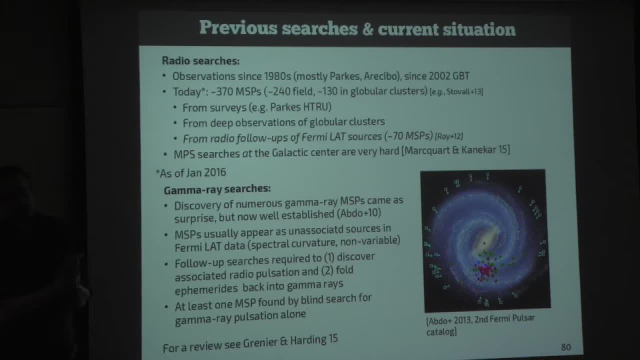 Or what was very promising is to look at gamma-ray, unidentified sources, So Fermi sources found by Fermi satellites and gamma-rays. You don't see their pulsation because you see a couple of photons per day or something like this, but they pulsate. 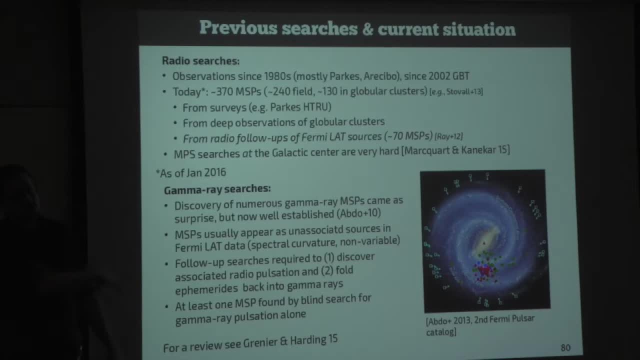 every millisecond. So to find pulsation in the gamma-rays you first have to write the radio pulsar in radio, millisecond pulsar in radio. Then you can measure the ephemeritis, so the frequency, basically Fold this back into gamma-ray data and then confirm that. 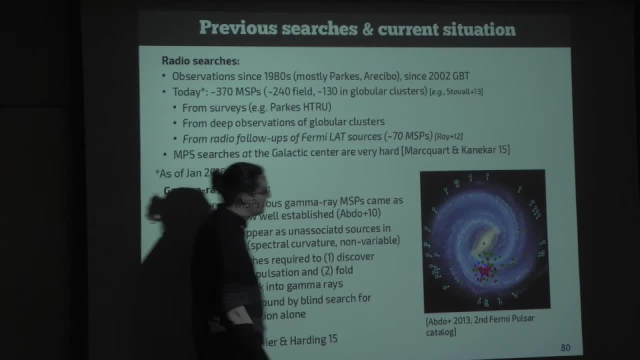 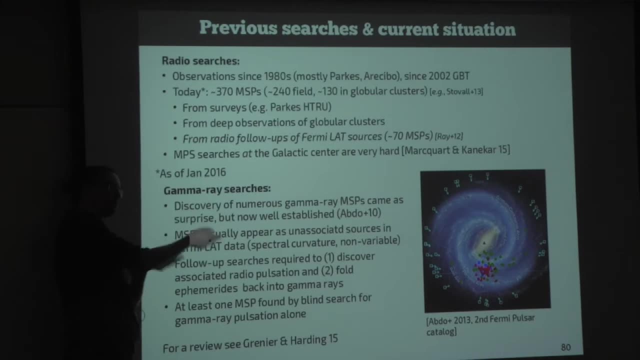 also the gamma-rays are pulsating with the same frequency, And this again only works for sources that are nearby, because first you have to see them in gamma-rays, then you have to see the radio counterpart and then you need enough statistics to see the. 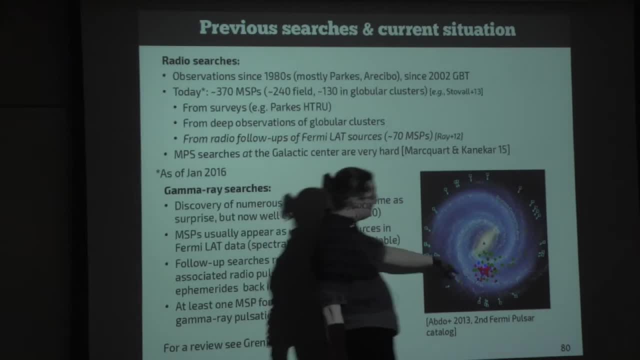 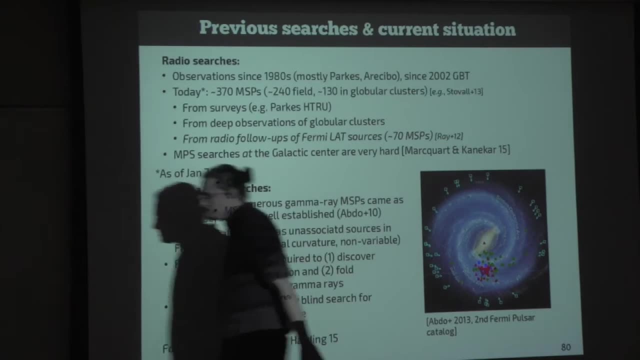 pulsation in gamma-rays again. So this is why you typically see only close ones. But it's you wouldn't be surprised if there are millisecond pulsars everywhere. right, If they are here. So what we did to estimate now? 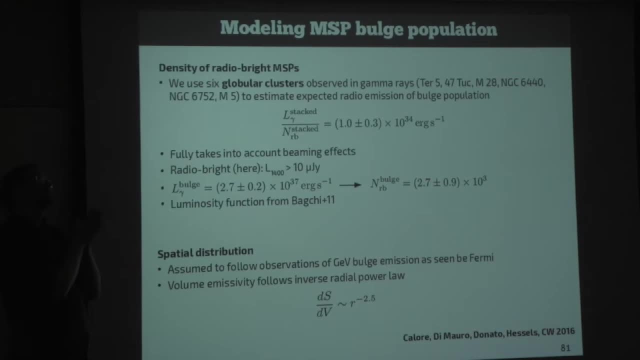 so the trick is now to estimate what this GV axis would look like in radio. right, The problem is tricky, because what we see in gamma-rays is just the diffuse emission of, if there's a millisecond pulsar, all millisecond pulsars at once. 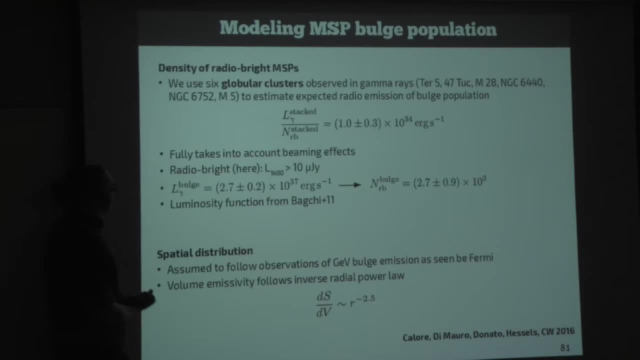 Whereas what we are interested in is the radio luminosity function of individual millisecond pulsars in the bulge right And the normalization. And this is made complicated by the fact that, depending on the angle at which you look at the millisecond pulsars, you either see lots of emission or not, And also the emission angle of gamma-rays and radio emission is not the same. So for some you might only see the gamma-ray emission or the radio emission. So you can't do this easily on a source by source basis. 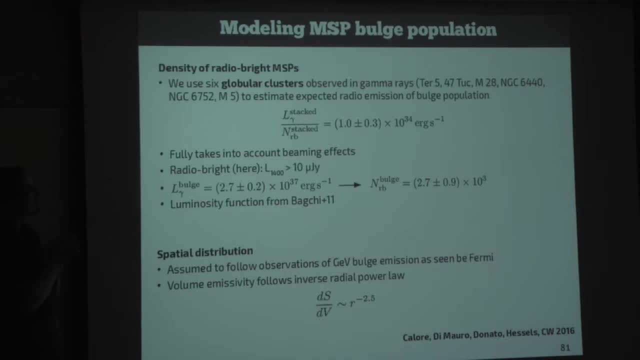 And you can't do this easily by just modeling the entire population on first principles. But what we did, what works, is to use globular clusters as proxies. So globular clusters, as I said, have lots of millisecond pulsars in them. They are just observed in radio And they shine in gamma-rays, And the gamma-ray emission is most likely completely dominated by the millisecond pulsars. So basically it's like a mini galactic center excess right? So you have the combined gamma-ray emission. 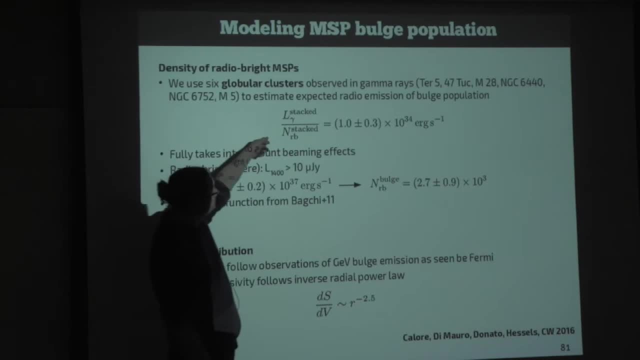 and you have the radio luminosity function that you get from individual sources. So what we used is a bunch of globular clusters- six- to estimate the combined gamma-ray emission that we would get per per radiobright millisecond pulsar And radiobright means. 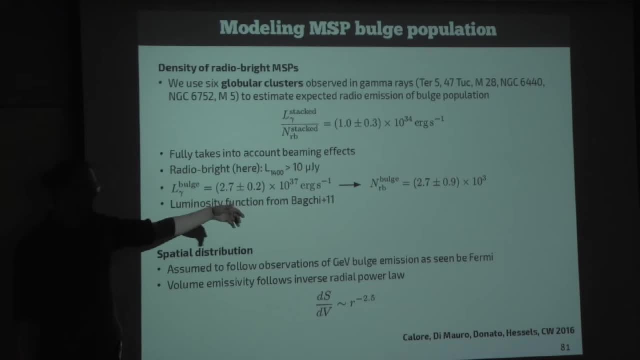 it has a luminosity of 10 micro Jansky at the distance of the galactic center. This is some radio astronomy unit, But it's not very bright. This is actually. we call it radiobright, but it's already on the hard to detect. 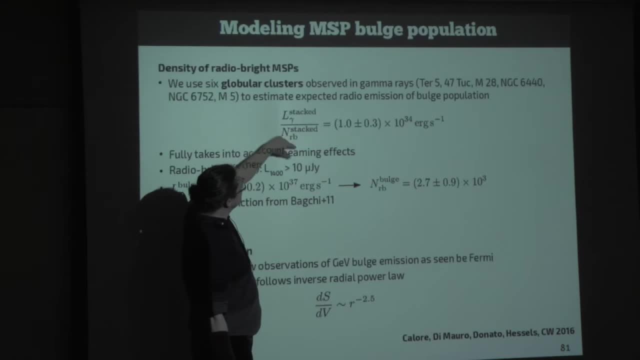 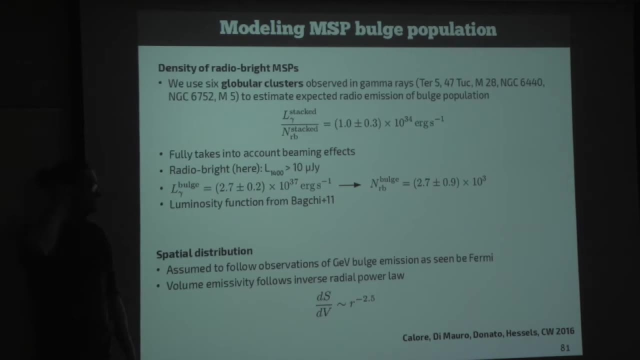 side Anyway. so in this way one gets that per radiobright millisecond pulsar one should see around 10 to the 34 ergs per second, And then one can just rescale this to the 10 to the 30s, roughly 10 to the 37. 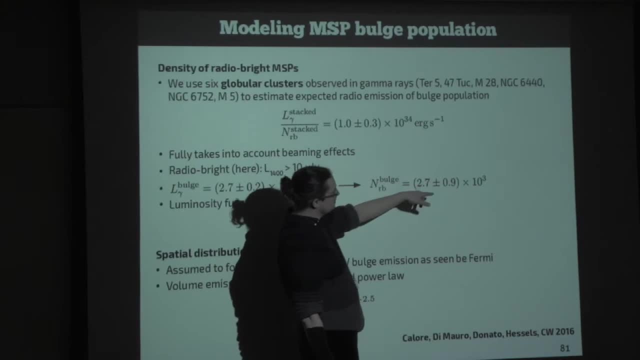 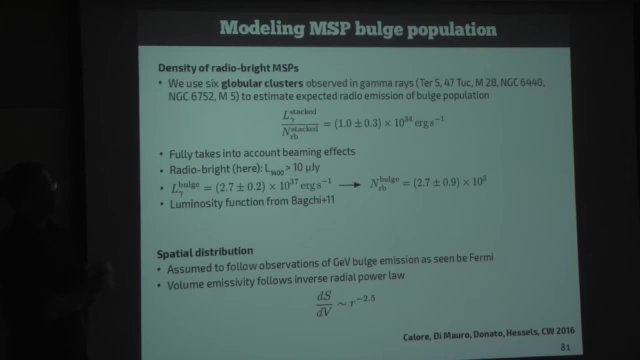 ergs per second And we got that. there should be around 3,000 radiobright millisecond pulsars, And probably there are tens of thousands, Because most of them, or many of them, will actually not point towards us, But anyway, so in this, 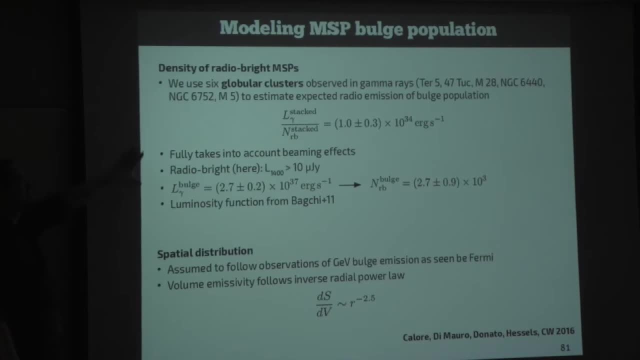 way one can get a relatively reasonable prediction for the amount of radiobright millisecond pulsars. There are caveats to this. Maybe there's a difference between the millisecond pulsars in the global clusters and the one in the bulge. Anyway, that's the number. 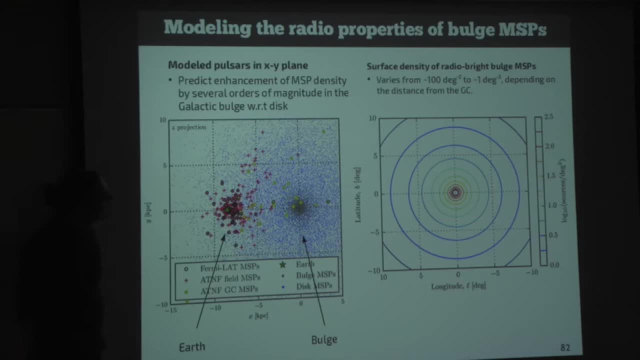 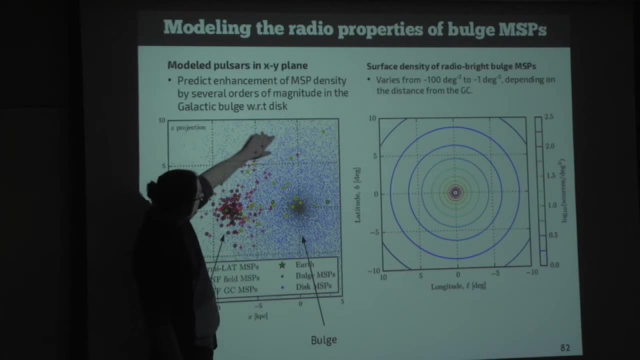 Spatial distribution. one can just infer from the GV-axis And then one can put this together. So this is a model for millisecond pulsars for the galactic disk seen from the top. This here would be all the millisecond pulsars in the 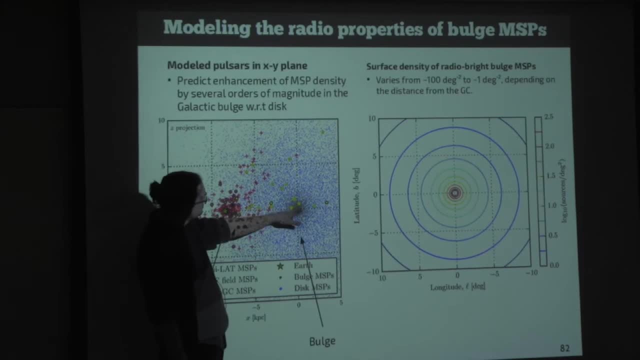 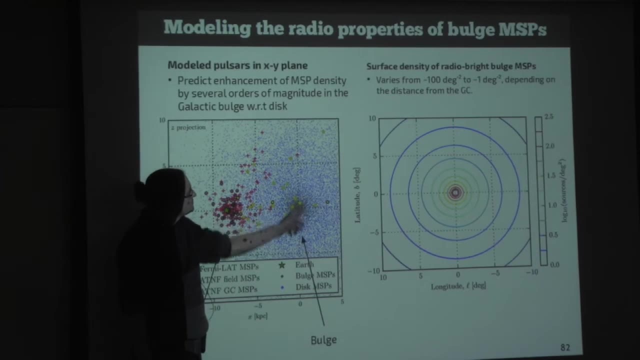 disk just extrapolated from the ones close to us. And then there's this huge gray dot, which are the many, many millisecond pulsars- 3,000 in our case- that would sit just in the galactic center region, in the galactic bulge. 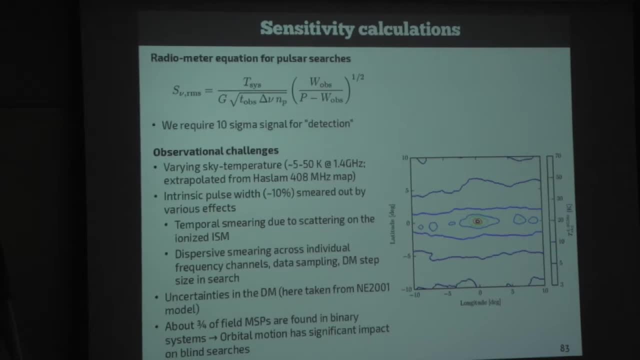 And what one can then do is to do a careful sensitivity calculation for a radio using the radiometer equation. There are lots of effects that play a role. In particular, if you look through the galactic disk, you look through lots of ionized 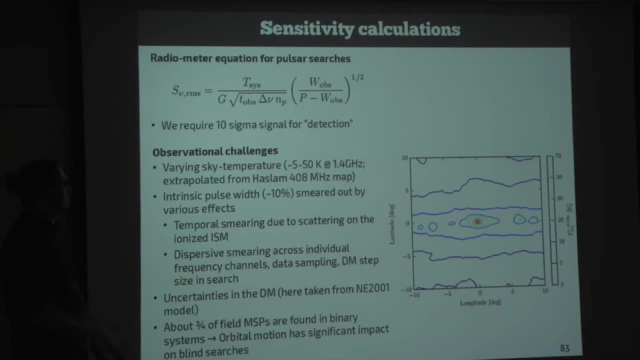 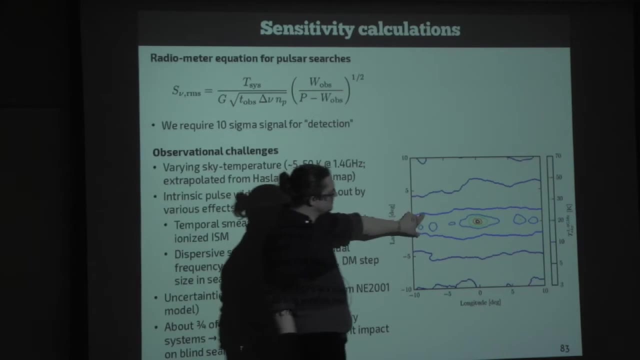 material which distorts the pulsation. So basically you get temporary smearing due to scattering on the ionized industrial medium. So you can't very well look for millisecond pulsars in the disk and you shouldn't look for millisecond pulsars 20 degrees away. 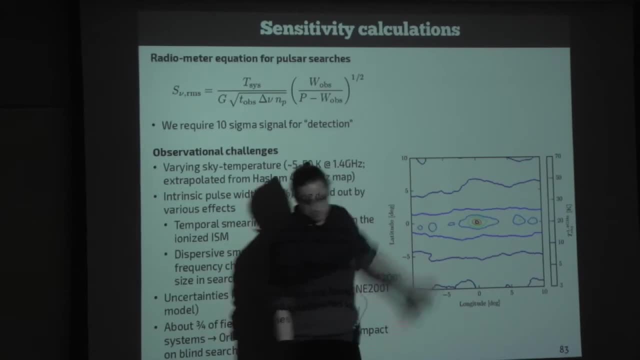 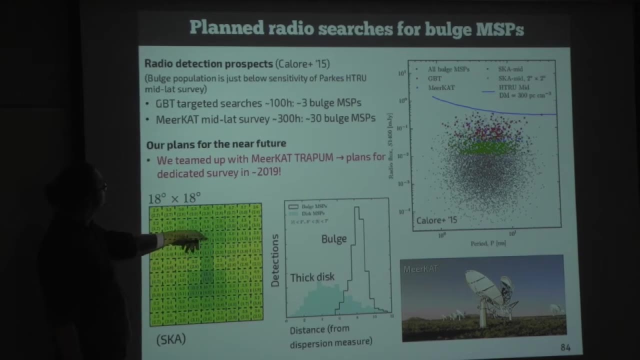 because there's no GV access there. There's somewhere, a sweet spot which we identified to be roughly here, so like 2, 3 degrees away above and below the galactic center, And the good news is that future radio telescopes should be able to see this. 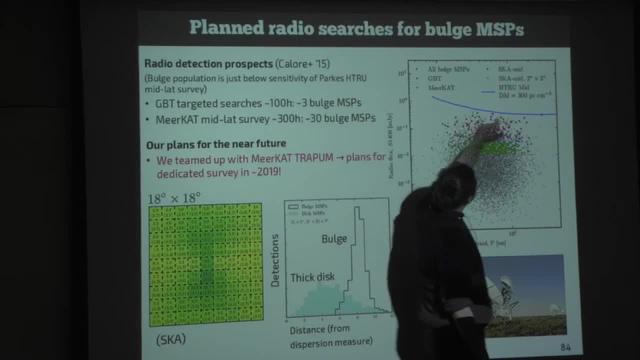 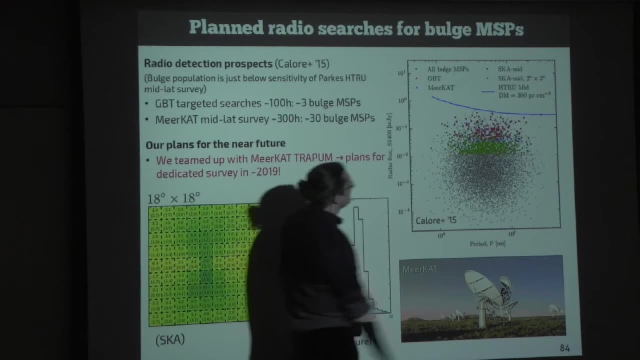 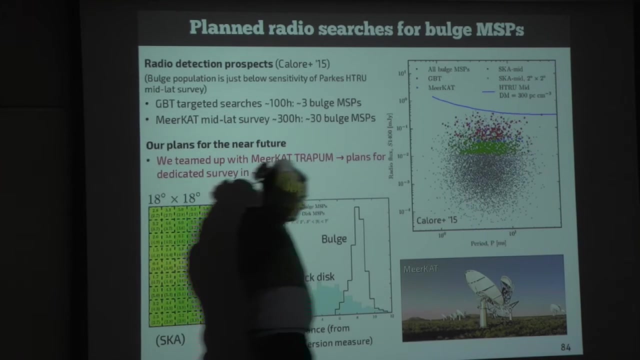 So this is the entire bilge population that we modeled. This is the best upper limit from the Parkes high time resolution universe survey And the dots here show what GBT should see. So the Greenbank telescope, The problem with Greenbank telescope: 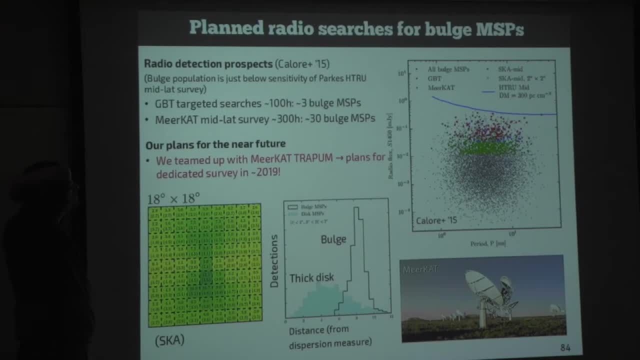 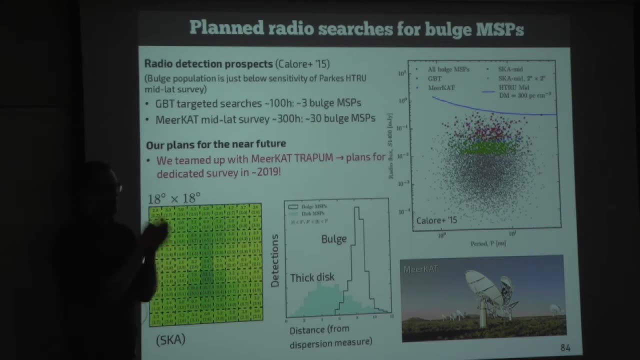 we tried several times to get time on Greenbank telescope. The problem is that you can't do a survey with this thing because, again, the field of view is pretty small. so one already needs to know where to look and one needs to know, basically, the strategy. 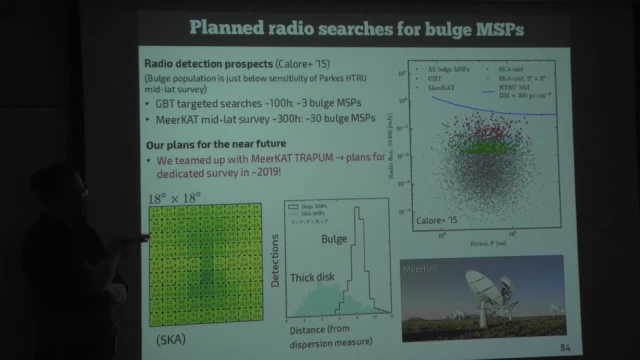 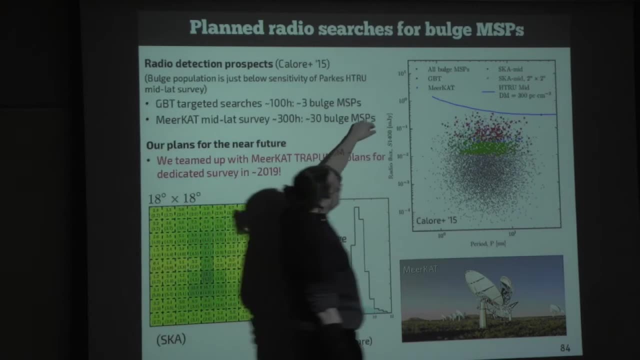 there would have been to look at reasonably bright gamma ray sources in the inner galaxy. They can't be too bright because then they couldn't be possibly part of the bilge population And then there are various problems with this. So it boils down to, if you have like, 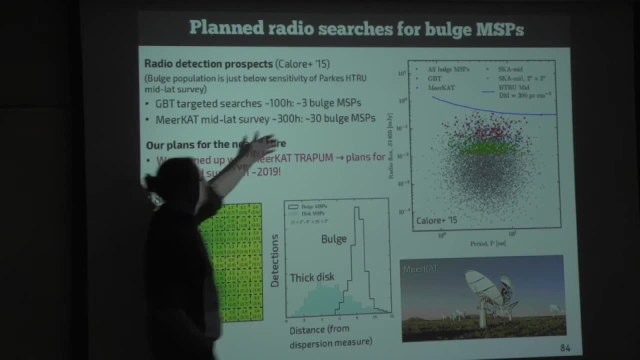 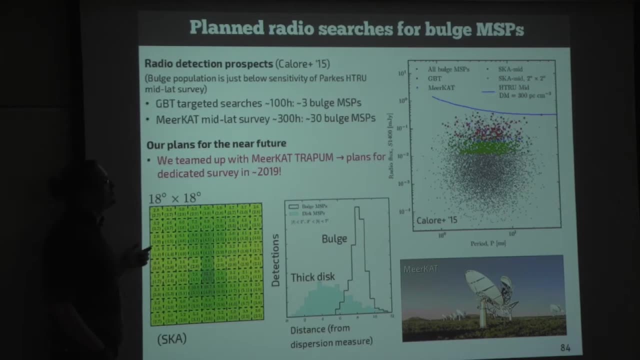 100 hours on GBT, you maybe find 3.. And they didn't find this very convincing, So anyway. so the good thing with MERCAT is that MERCAT can actually do surveys. So this is an interferometer. instead of one beam, you have like 400. 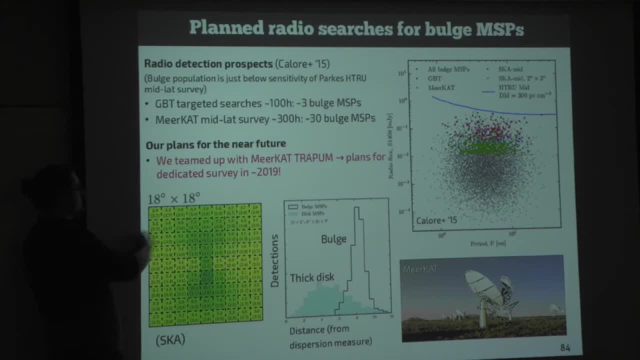 So you can actually go through a large region of the sky and just do a blind survey And it turns out that with 100 hours of MERCAT time one should maybe see 10 or so. So this was like if you get 300. 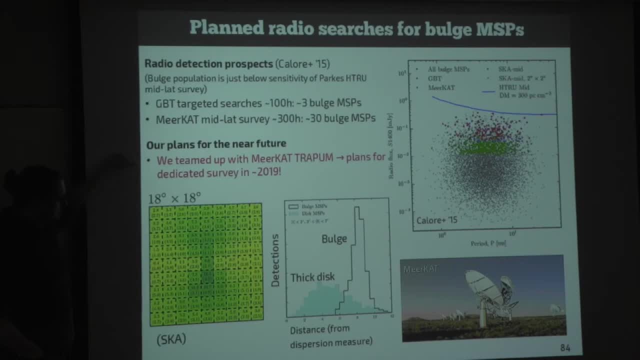 hours. we should see 30. And yeah, so we worked together with them to make this happen. hopefully in 2019 or something. The telescope is now getting commissioned and up and running. It's in South Africa- one of the precursor. 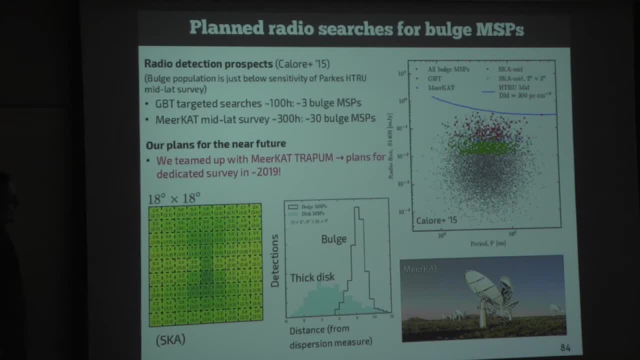 instruments for SKA And yeah, hopefully there will be a search next year. we will see. And the nice thing with is that one can use this dispersion measure so the effect that the radio emission is affected by the free electrons along the line of sight one can use. 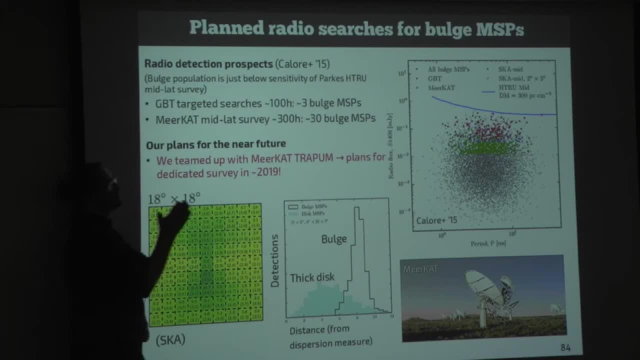 and it distorts or basically delays in frequency dependent fashion the pulsation. One can use this to estimate the distance, And so one should see around 10, maybe within 100 hours of observation time from the bulge, Then probably also 10 or 20 along the line. 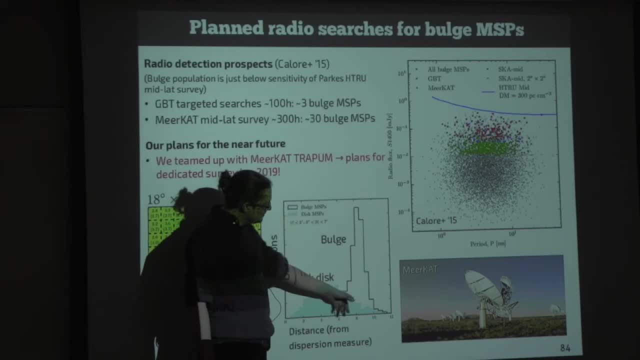 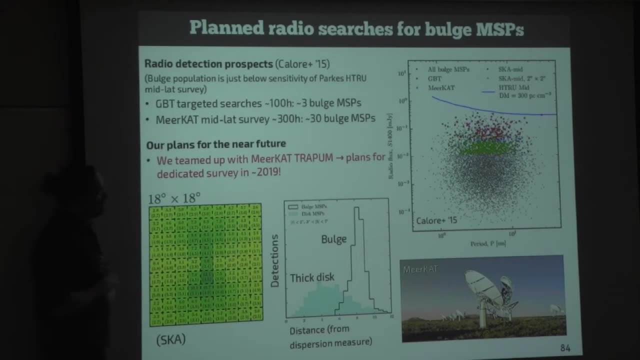 of sight, But you can actually make then a histogram, in principle at least, where you should see that there are a bunch of them really just peeking at the distance of the galactic center, And this would be a pretty strong indication that there is that the 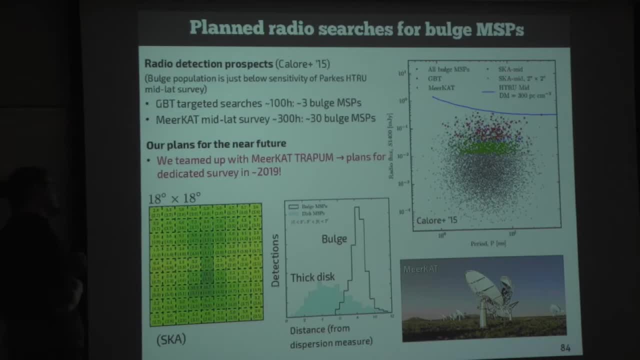 GEV access is from millisecond pulses, Then to prove that 100% of the GEV access is caused by this and it's not like 50% and then 50% of dark matter signal, would be super hard, But I mean. 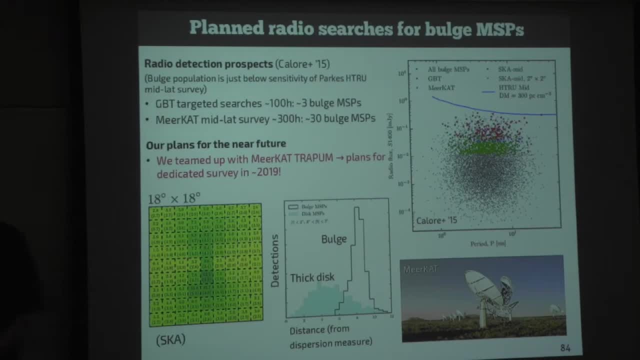 this would be it. So how big? how? in degrees? I don't know whatever. what fraction of the galactic center can this meerkat away observe at the time? How large is the field of view? Yes, With respect to the galactic center. 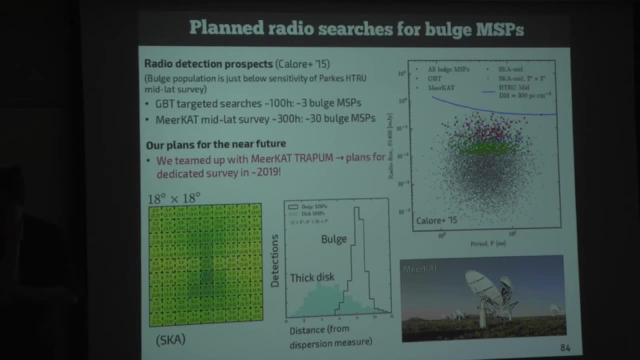 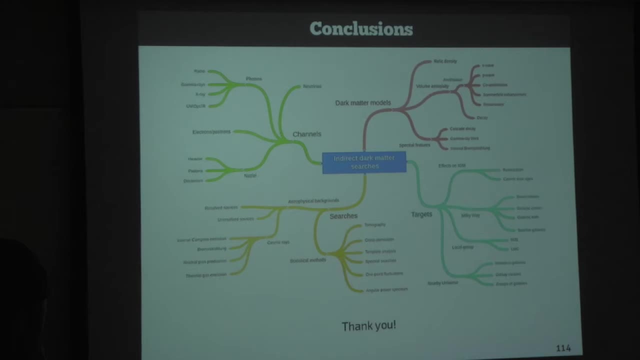 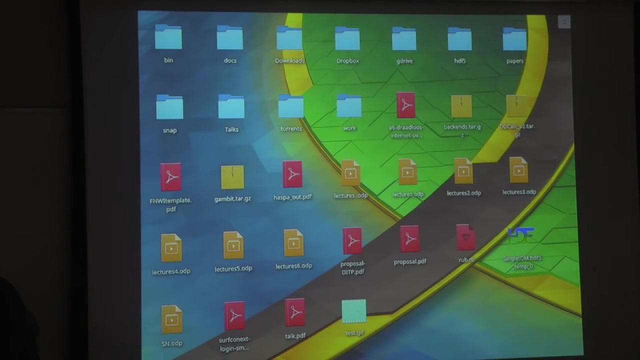 is it comparable or is it still much smaller? Maybe I still have. Usually it's very, very small. Yeah, I deleted the. okay, I don't have the slides here. Okay, fine, Let me just go back. Yeah, I don't. 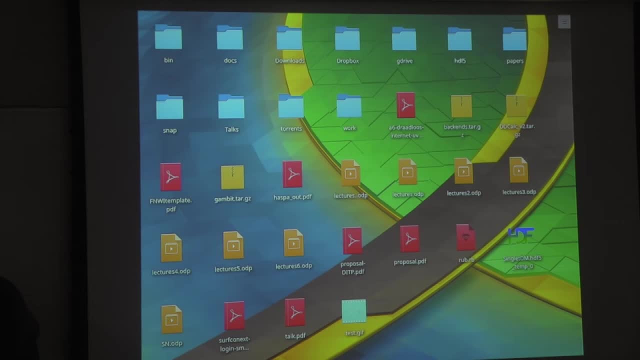 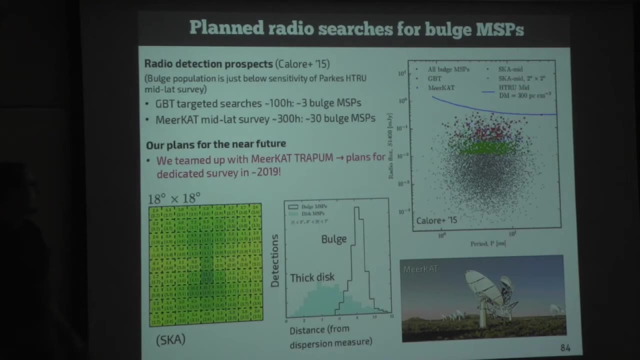 remember the numbers. Yeah, I can check it later. The point is, the field of view is about 400 times bigger than for meerkats, in some sense, So you can in principle do the survey just 400 times faster. So that helps a lot. 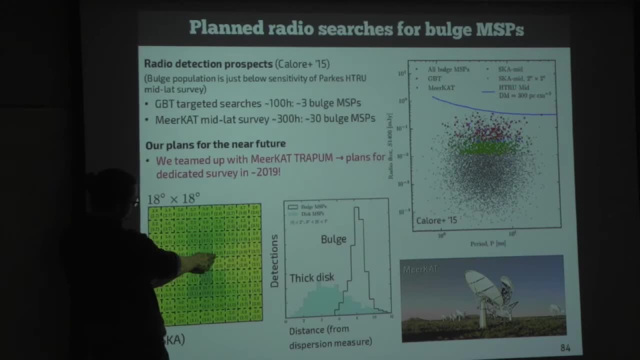 But I think for each of these- these are one or two by two degree patches- you still need a couple of pointings. So I think with- yeah, I don't remember- probably you need 10 hours per two by two region. 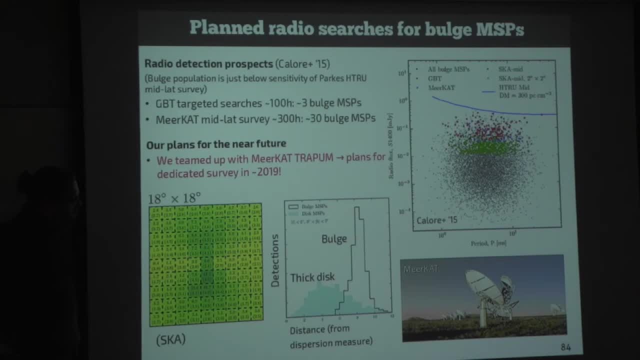 Is this a priority of the? would they dedicate the time? So the radio is the radio group and they are pretty much interested in this, definitely because it would be a pretty cool discovery And it's like in their hands somehow, right. So I mean they 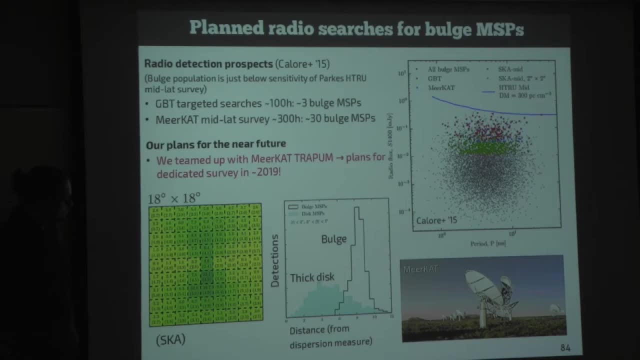 are the first instrument that should be able to actually do significant progress there. So we are together with Francesca Calora, actually we try to make this happen. We joined them and, yeah, the only challenge will be, or one of the challenges, 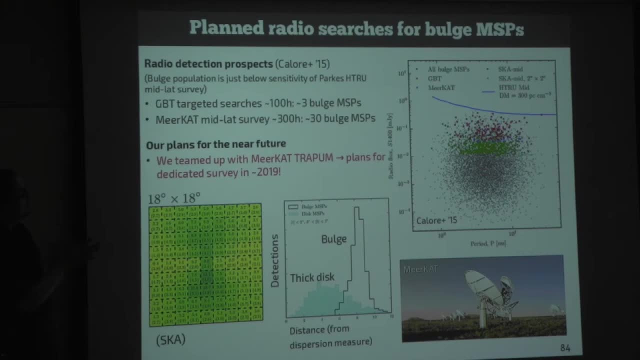 will be to get observation time. So this is not part of the key science goals, but this will have to go through the open calls. But since the entire Pulsar group is behind this, I guess likely that we will get the time Then. initially we try to. 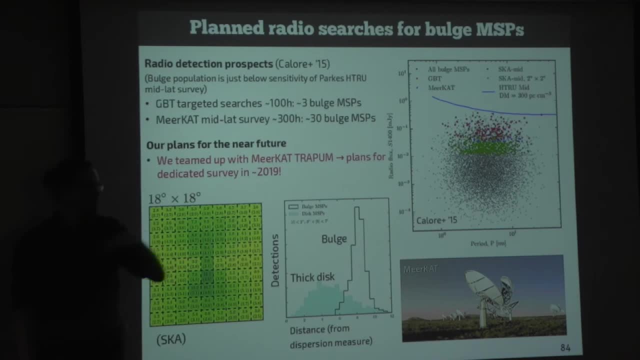 sneak in 300 hours of survey in their key science goals, which kind of didn't work. This would have been nice, but so now, since it's an open time proposal, we probably have to just take 100 hours. And then the problem is a bit if the 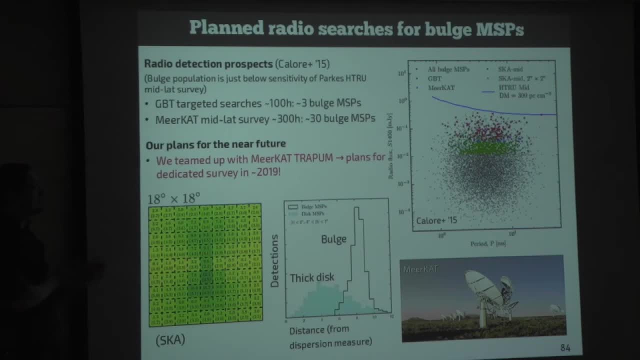 expectation value is 10, and the uncertainty of this expectation is probably still a factor of 2, at least. then maybe you find like: then maybe in truth it's 5, and maybe you find 2.. And then what do you say? So 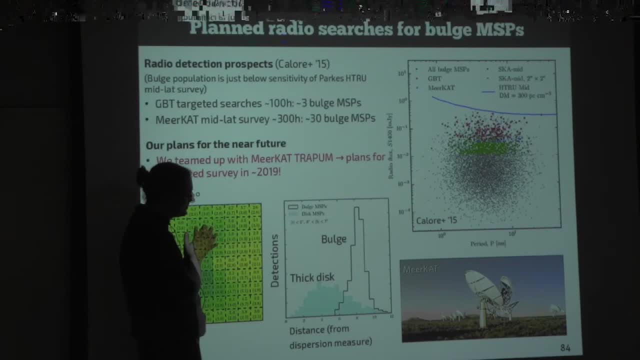 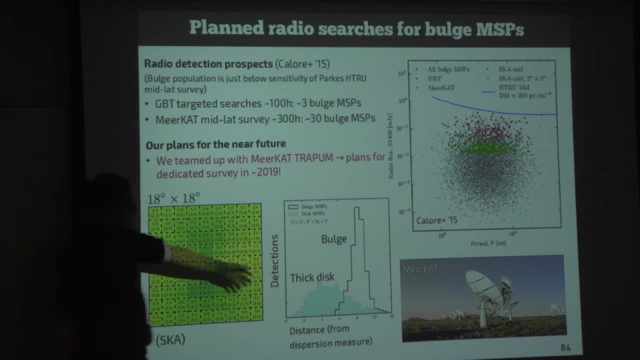 I think the goal is to find at least 1 or 2 in this first attempt and then get more time. Maybe we are lucky and we find immediately 10 or something. But, as I said, the nice thing is you can actually say something about. 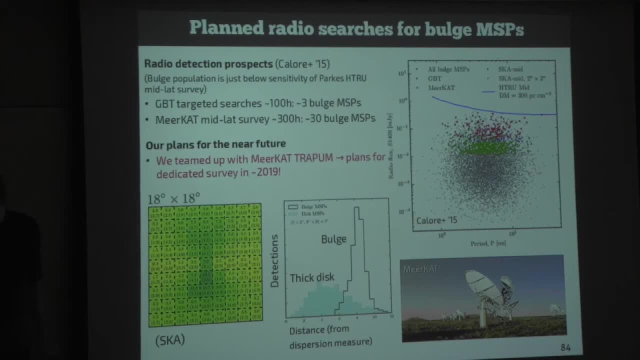 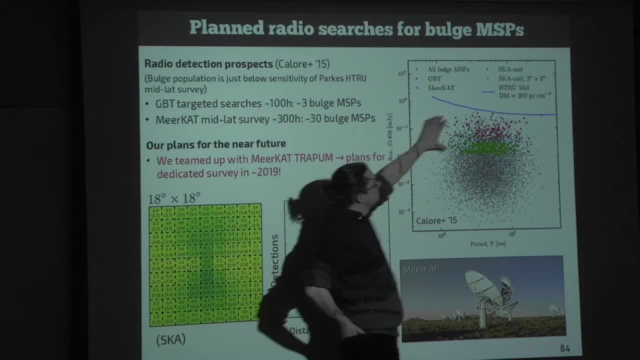 the distance. If one finds 0 at this distance, one has to see what this actually means, because then you could still argue that maybe the bulk population is just not as bright as the GBT, as the global cluster population. But if one starts finding something, this would be good. 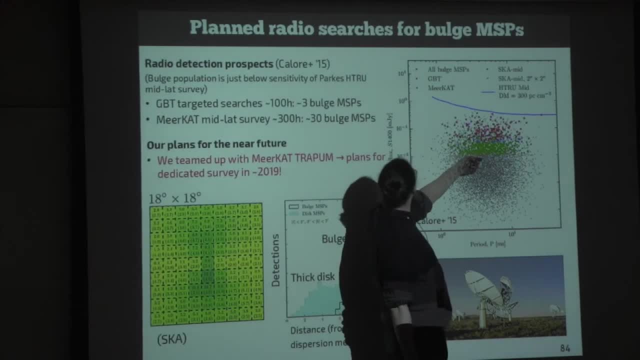 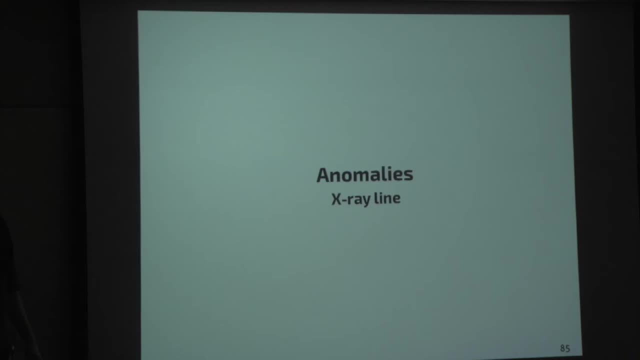 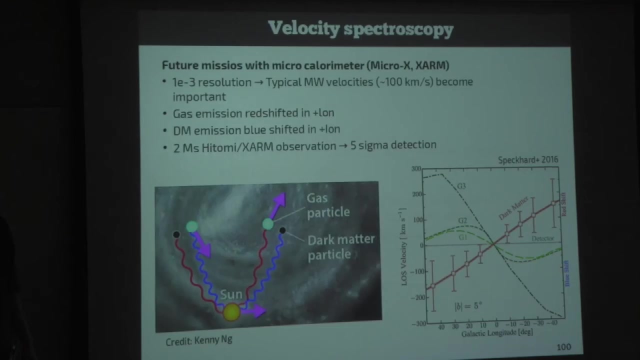 But okay, even then, with SKA, we are down here, so they should find lots of them, But someone just has to wait a bit longer. I guess my time is up. no, I think so. yes, Should we then ask? 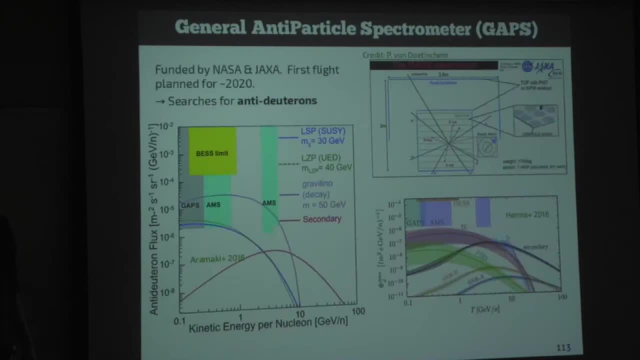 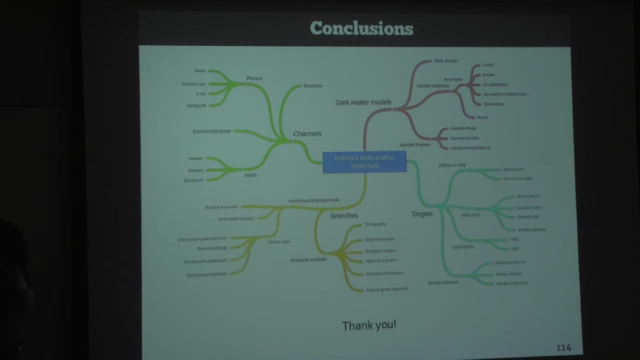 one more question, Maybe we have time for some questions, or two questions. So the resource for OIDLs? you don't see any gamma rays from them. Yes, yes, I'm not sure that everybody would agree, because there were at least some discussions about gamma. 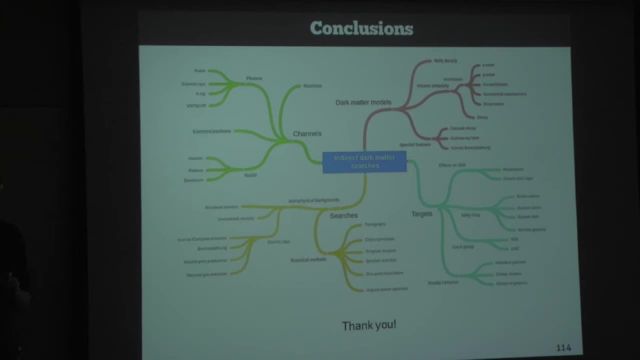 emission from reticulum 2, which is one of the dwarf swaddles where I don't know if the situation has changed. but the J value, I think, was not very well known, But the position was known and there were analysis about the gamma. 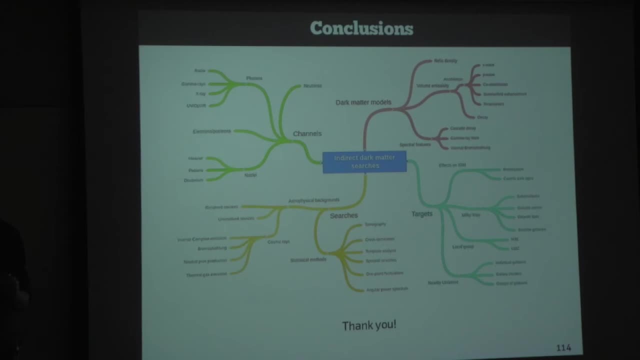 emission. There was weak indications for actually gamma emission from the source, but at the few sigma level. So the gamma ray accessed in this galaxy turns out to be from dark matter. The question is going to be: why Can you repeat the question? 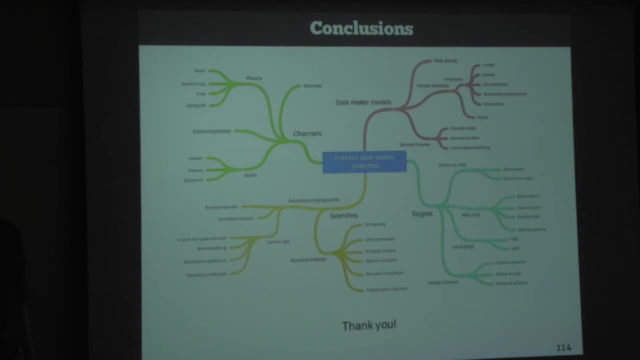 Why are these dark matter dominated dwarf swaddles? why don't they show it Like if it turned out to be dark matter in the galaxy? That would be the question. Yeah, so independently of reticulum 2, if the galactic 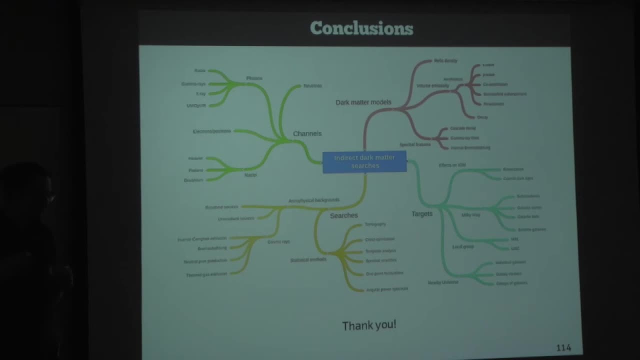 center access turns out to be dark matter. I mean, the only way really to prove it would be to find emission from dwarf swaddles, for instance, Given that there is no even interesting hint from them except for reticulum 2, but I mean the others. basically just give you limits. Even with more data- I mean, Fermi could measure now twice as long, but the mission time is already almost over the official one, so it depends a bit on what's going on. Still, this just gives a factor of 2 in. 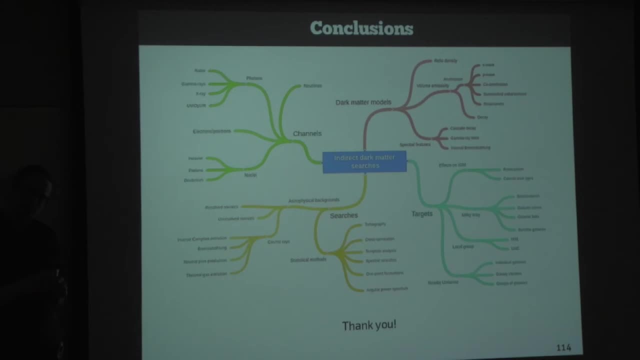 the data. so this will not make a huge difference if there is nothing already now. So with Fermi alone, this might be hard. What's fun is that antiprotons, which could have completely killed this thing, just don't do it, because. 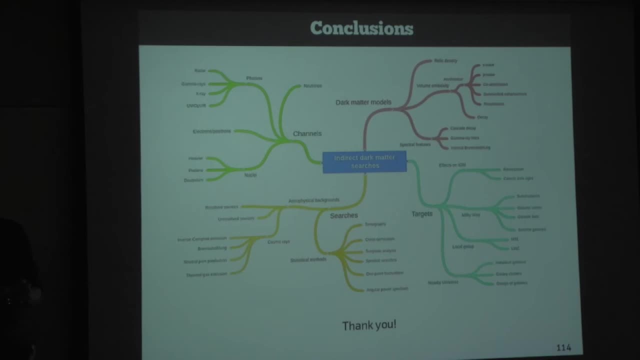 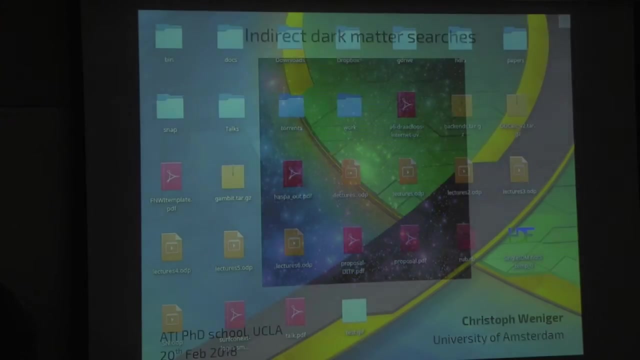 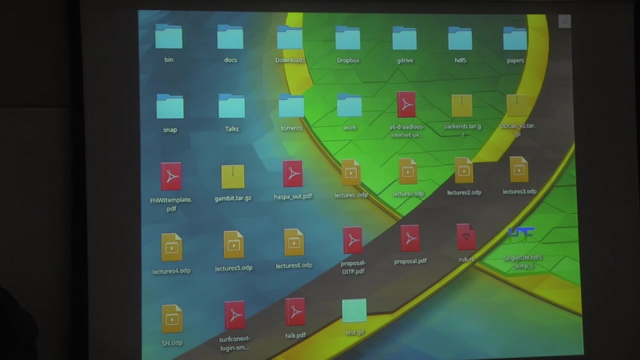 you get this like huperonophilic line. I mean you basically: yeah, it's a bit hard, but let me just show the slides again. I mean you get basically all analysis I have seen using using AMS data. you get this funny shape form.